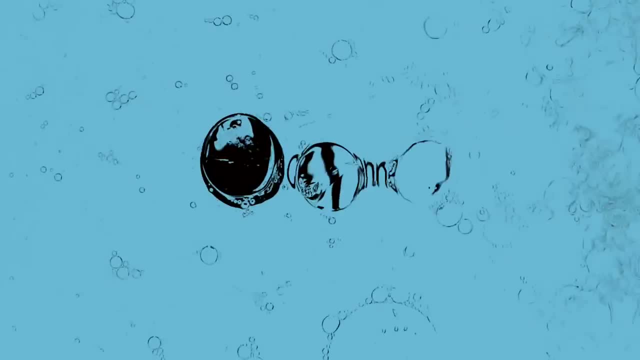 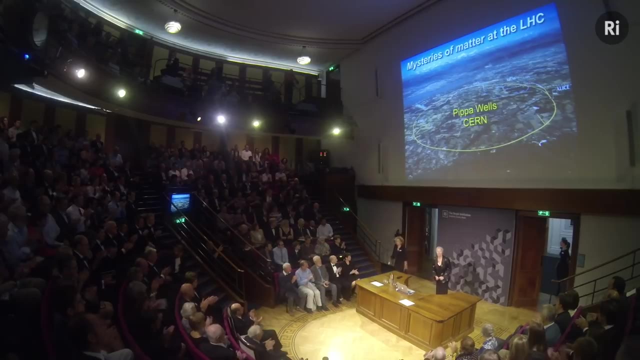 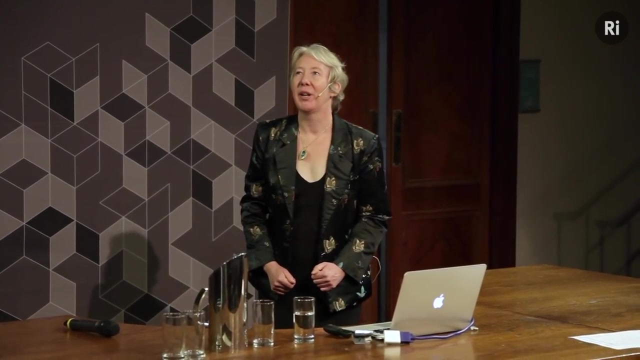 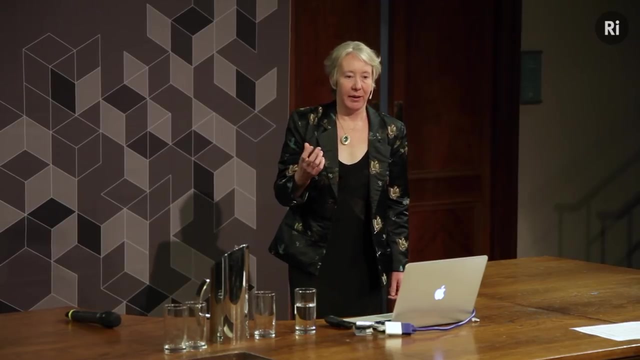 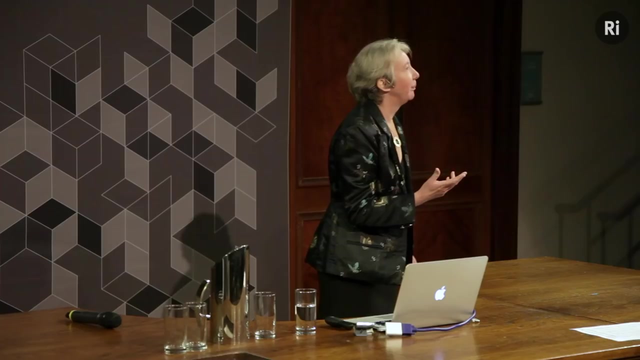 I work at CERN, home of the Large Hadron Collider, where we're exploring the mysteries of matter. Now, the LHC is a particle accelerator. It's the largest, highest energy particle accelerator in the world and it's housed in a 27-kilometre-long tunnel. 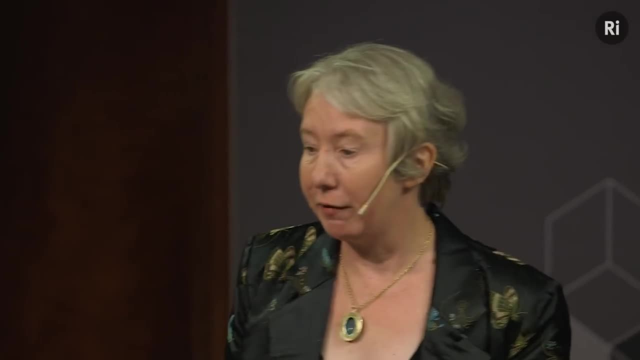 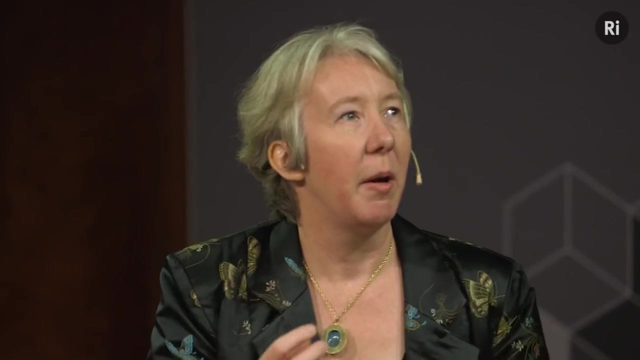 under the French-Swiss countryside near Geneva. Now I work on an experiment called ATLAS. It's one of the four huge detectors trying to measure the products of high-energy particle collisions at the LHC. I'm going to try and explain how the detectors work. 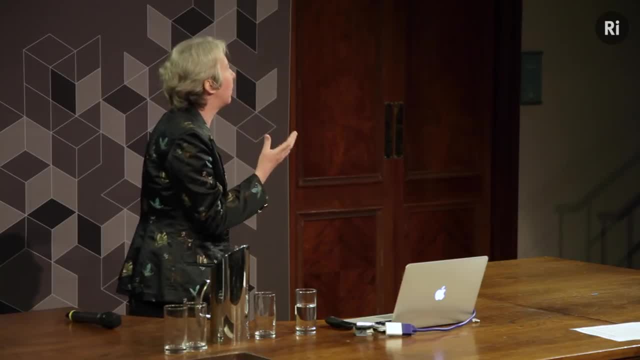 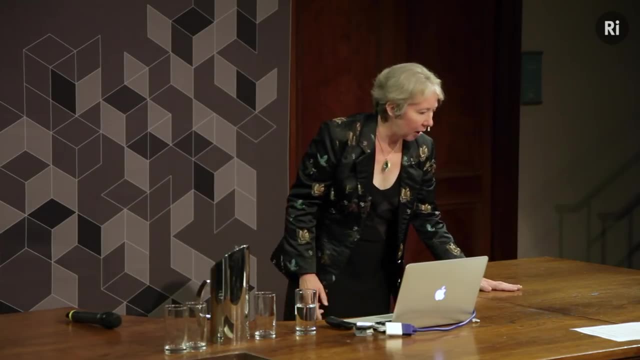 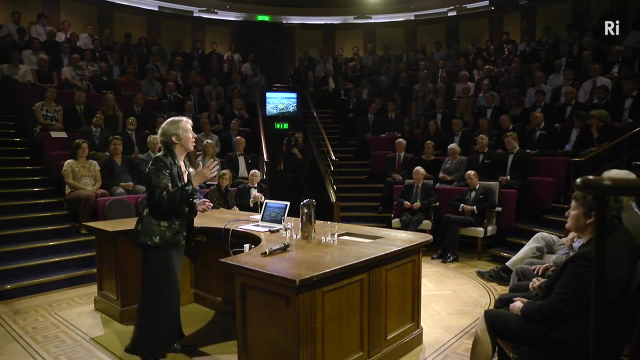 How do we pick out if a new subatomic particle might have been created? We want to understand how those particles interact. We want to understand matter at the deepest level, not just matter in the world around us, but matter out in space, in stars, in galaxies. 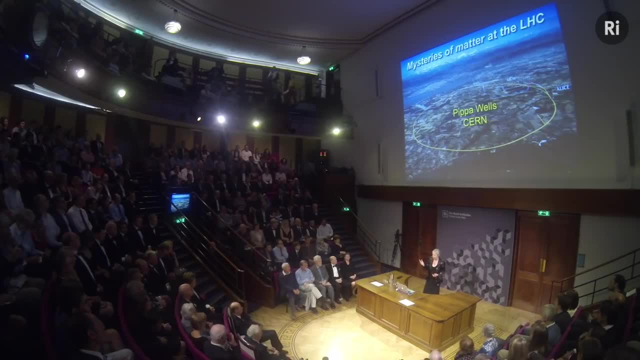 all the way up to the largest structures in the universe. Now, scientists here at the Royal Institution have had an awful lot to say about this. They've had an awful lot to say about this. They've had an awful lot to say about this. 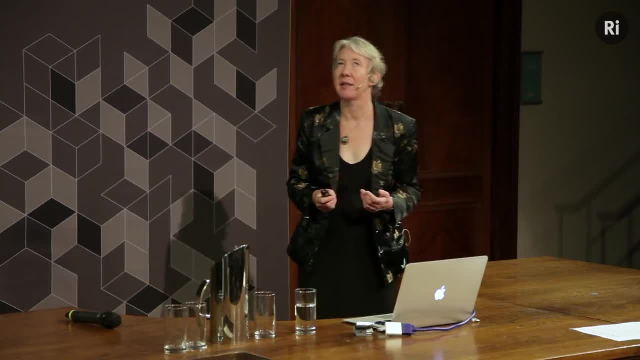 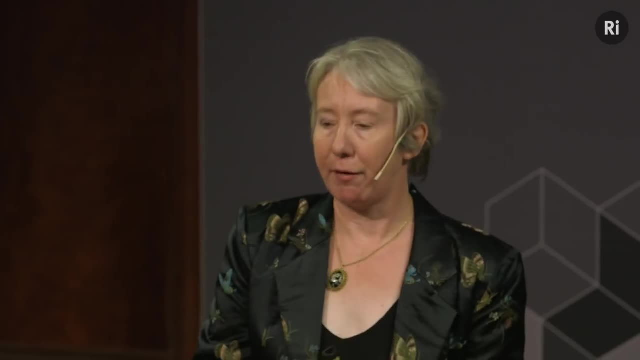 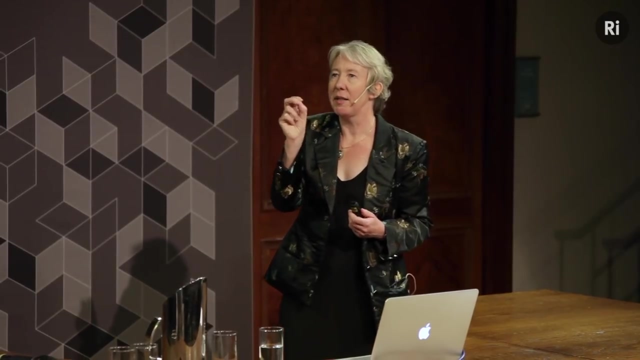 They've had an awful lot to do with unravelling the mysteries of matter over the years. Michael Faraday understood the connection between electricity and magnetism, and several new chemical elements were discovered here. Chemical elements are made of atoms, which were thought to be the smallest indestructible bit of matter. 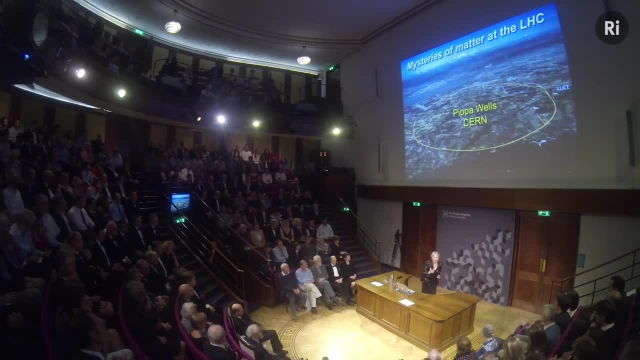 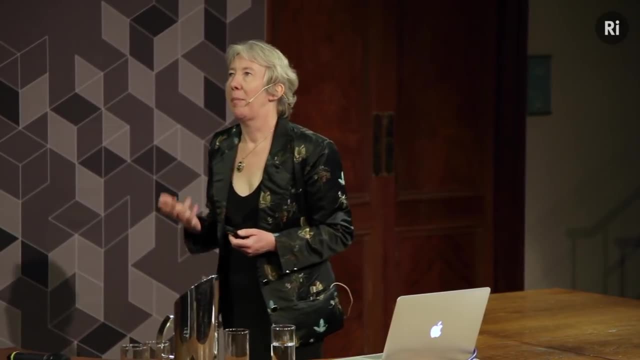 the smallest piece of matter you could have Now. each element has its own atom, and if you arrange the atoms in order of increasing mass, a pattern starts to emerge. Now I'm sure you're all familiar with the periodic table of the elements. 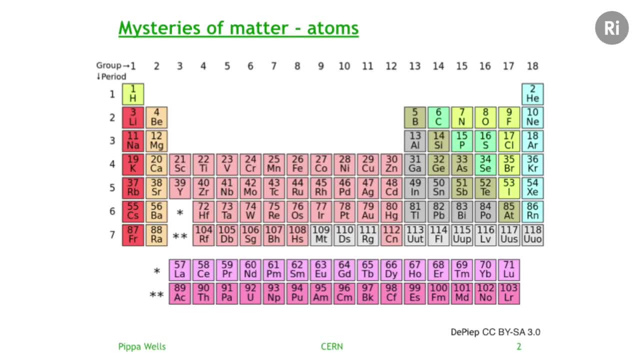 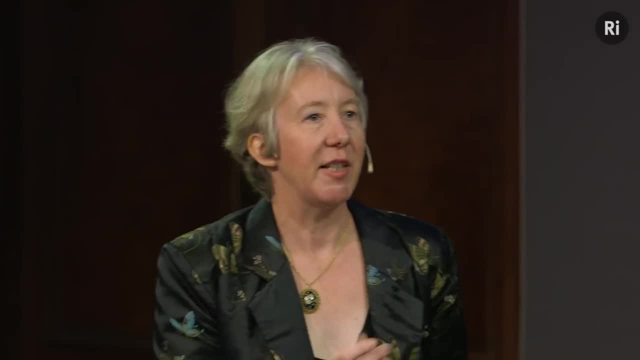 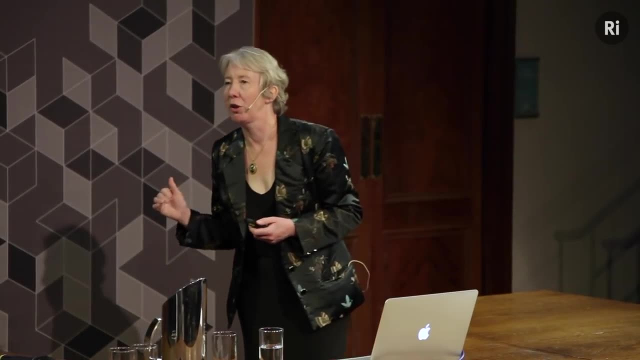 It's quite complicated. There are hundreds of different chemical elements, But we can understand this whole structure with just three subatomic particles. So each atom has a very dense nucleus. Inside the nucleus there are protons which are positively charged and there are neutrons which have no charge. 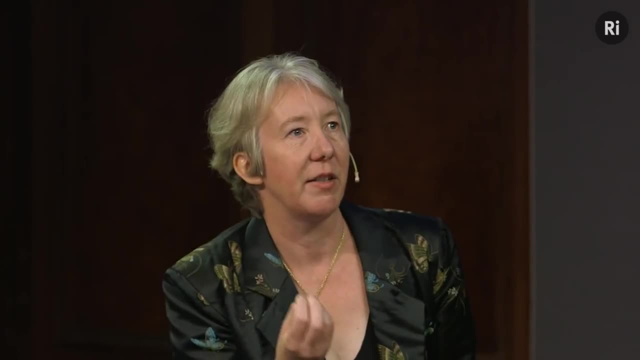 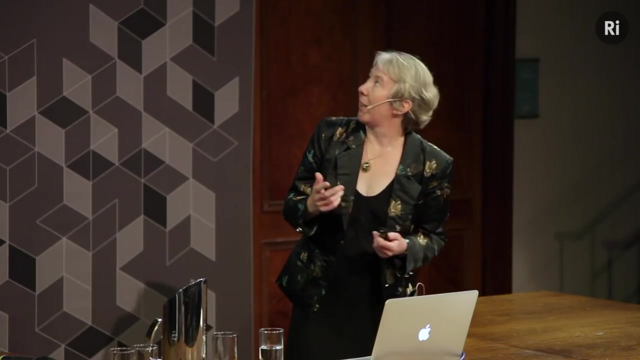 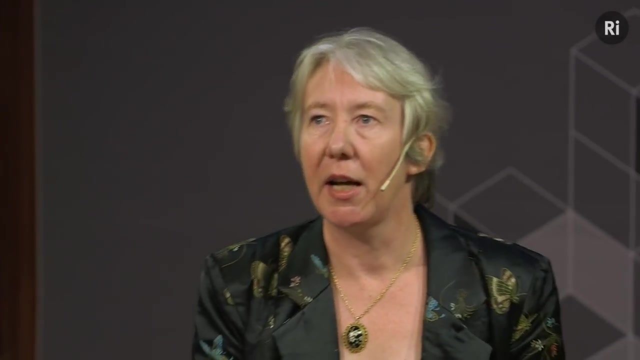 Almost all the mass of the atom is concentrated in the centre, in this very dense nucleus, and then there are electrons flying around the outside. The hydrogen atom is the simplest. It has one proton and one electron, and it's protons that we use in the LHC most of the time. We accelerate protons to very high energy and let beams of protons going in the two opposite directions collide together in the experiments For a few weeks of the year. we go to the other extreme. We choose lead nuclei with 208 protons. 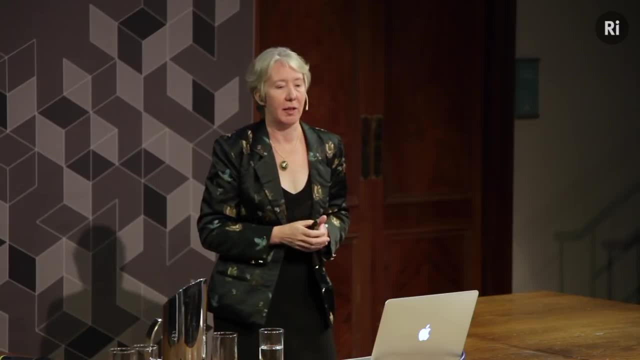 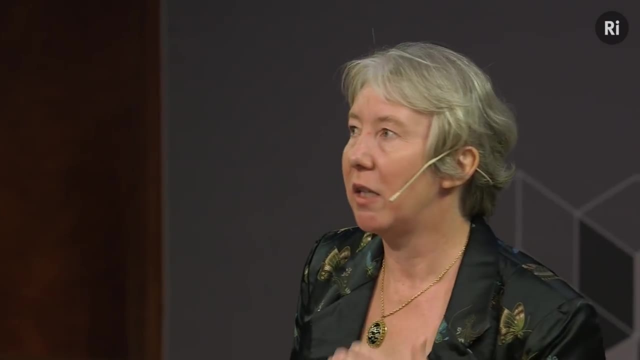 protons and neutrons all packed in that nucleus, We collide lead nuclei together. But the protons and neutrons, they're not fundamental particles either. We can actually go a layer deeper and that brings us to our standard theory, our standard model of particle physics. 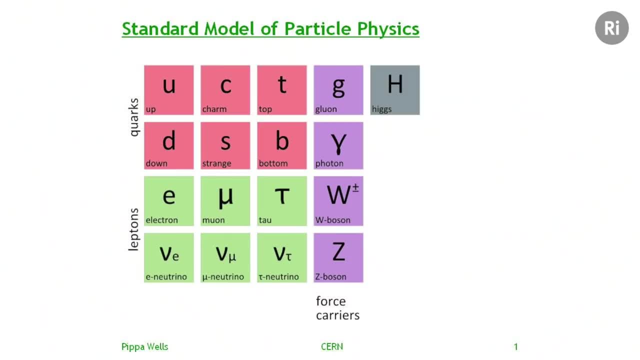 So this is a sort of periodic table of fundamental particles, the smallest particles we know. Now let me break it down for you so you can see the different pieces, Starting with ordinary, so ordinary matter, protons and neutrons. they're made of quarks. 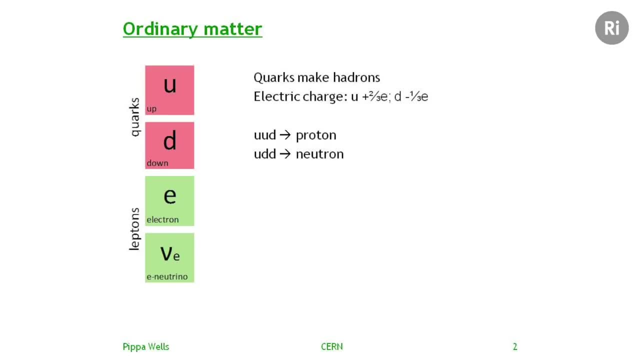 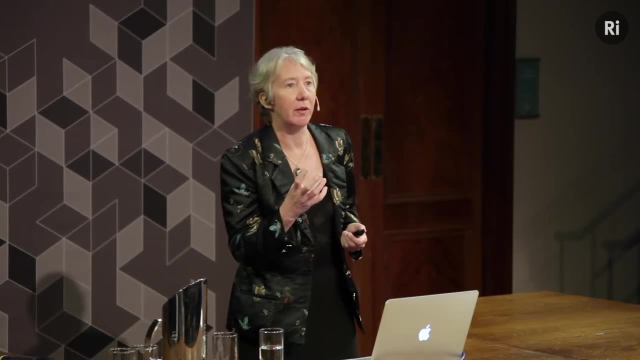 We need two types of quark to make protons and neutrons up quarks and down quarks. So the up quark has two-thirds of the charge of a proton, The down quark has minus one-third. So if you put together two up quarks and a down quark, you've got a proton. If you put together two down quarks and an up quark, you've got a neutron. Electrons, on the other hand, are lighter particles, So the quarks are lighter particles. The quarks make up these heavier particles. 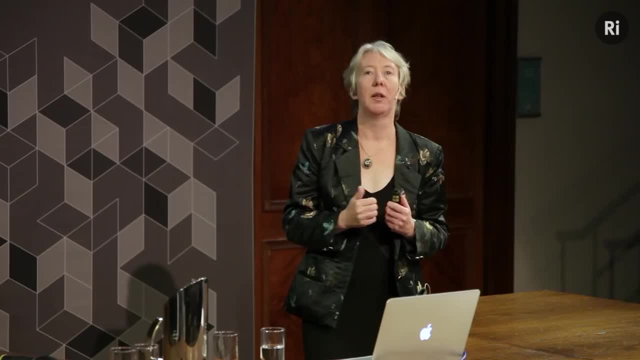 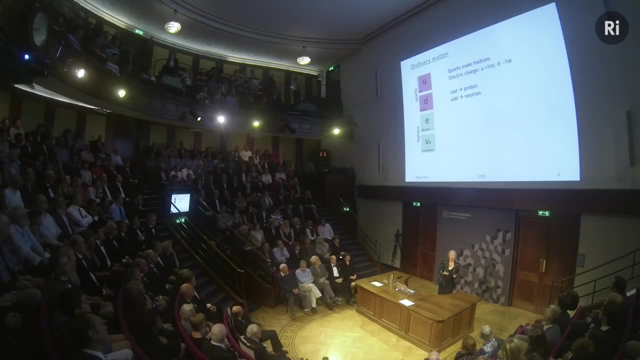 hadrons like protons and neutrons. The leptons are the lighter particles. We know of no substructure for electrons. So there we go. With three particles. we can still explain all of ordinary matter: up quarks, down quarks and electrons. 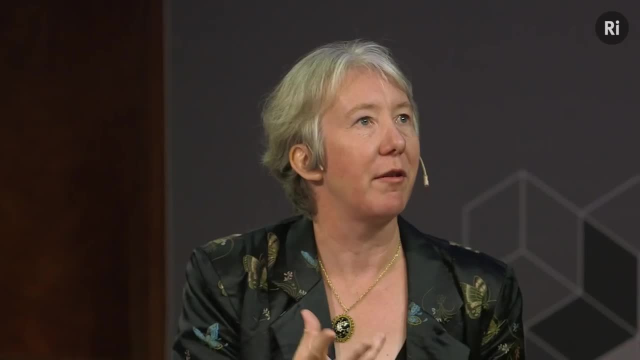 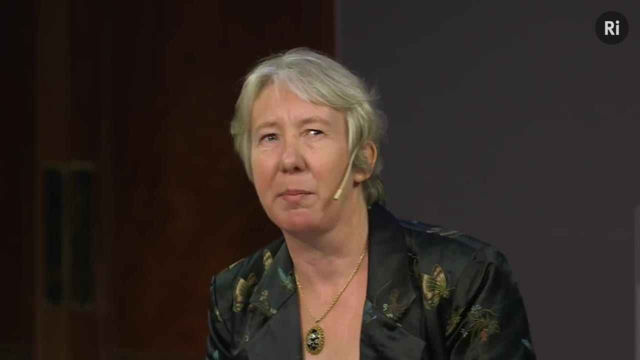 But I've had to add this fourth particle and you'd need that fourth particle whether or not you knew about quarks, whether or not you thought that protons and neutrons had substructure. That's a neutral particle, It's almost massless and it's a neutrino. 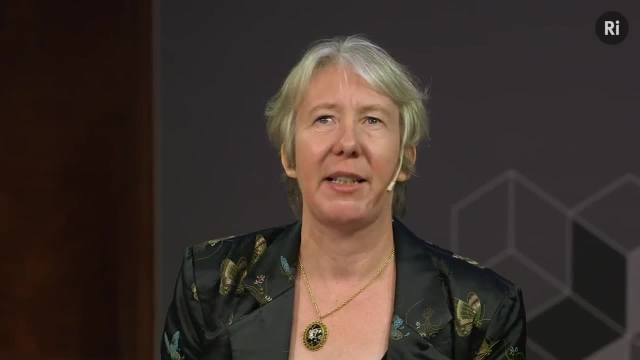 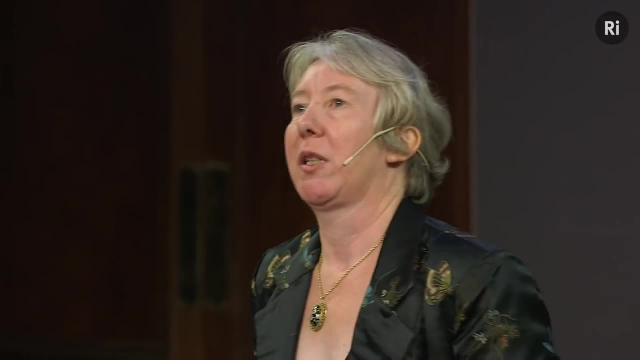 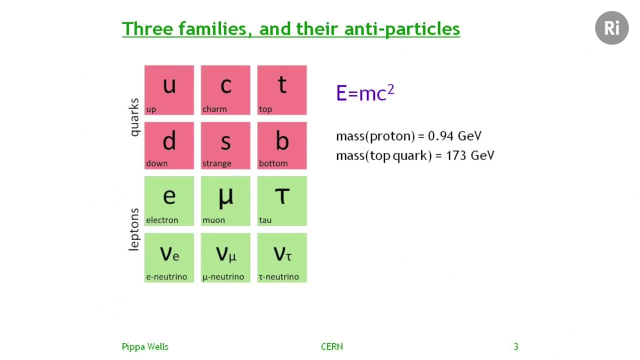 You need neutrinos if you want to understand radioactivity, if you want to understand nuclear fusion that powers the sun. But there are more families of particles. So this is actually just the first family In cosmic rays or in particle collider experiments. 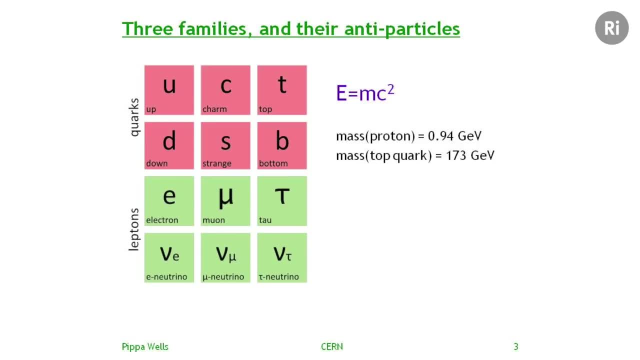 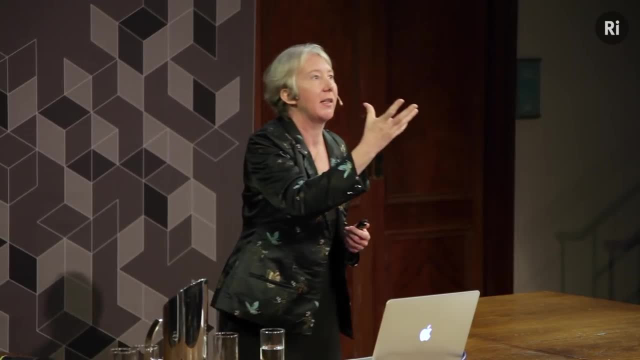 we can actually make weirder particles. The strange quark is named after cosmic rays that were observed that lived for a certain amount of time and then decayed. So these heavy particles, these heavy particles, heavier particles, they're not stable. They're unstable. They live for a short amount of time and then they decay. The strange quark is a sort of down-like quark. It has a partner, the charm quark, And then in the third family there's the bottom quark B. 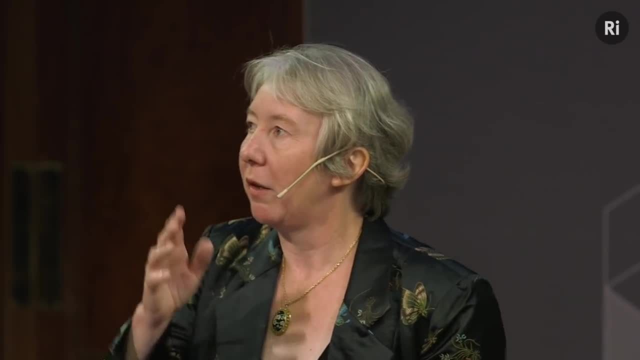 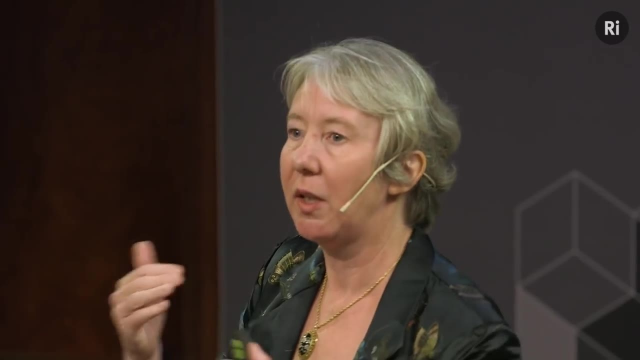 and heaviest of all is the top quark, Then the leptons. they're also repeated in the three families. So the electron has partners in the other families, muons and tau leptons, and each of those have their own neutrino. 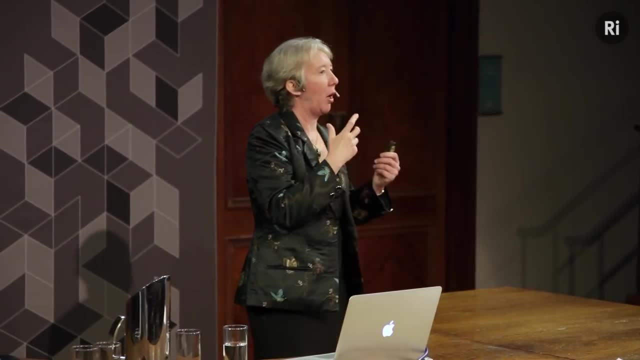 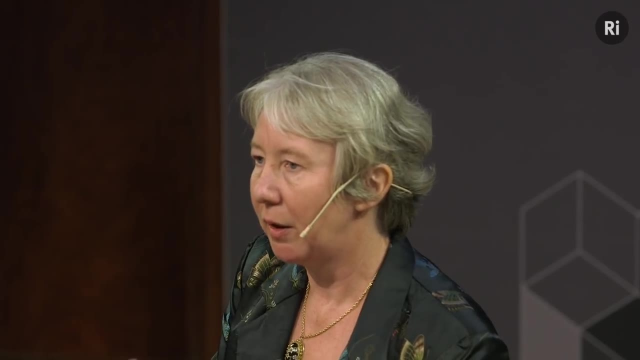 And each of these particles actually has another kind of partner, an antiparticle. An antiparticle is like a mirror reflection: It has exactly the same mass but it has the opposite charge. So the electron, for example. the electron is a negative particle. It has a positive antiparticle called the positron. It has the same mass but positive charge. So these new strange charm top-bottom particles, we can make them in particle collisions. We take advantage of the famous relationship between matter and energy. 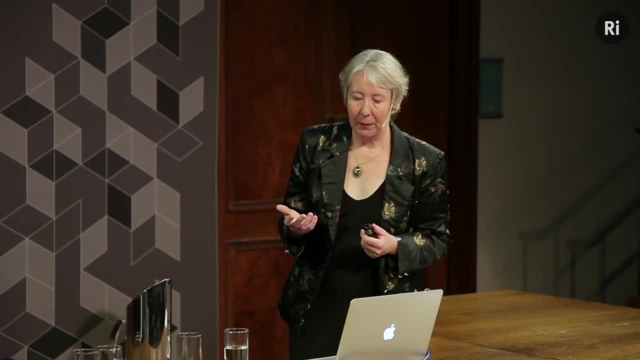 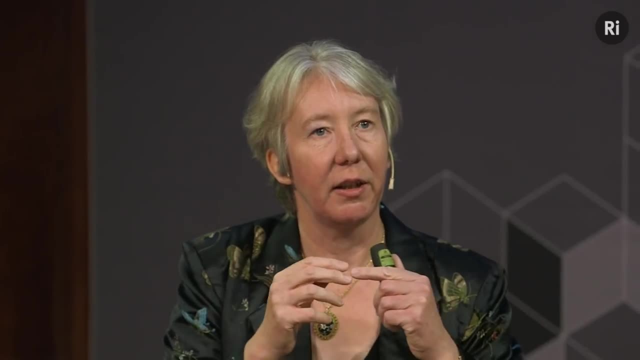 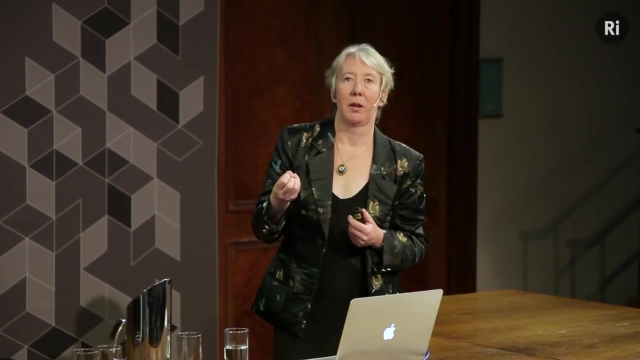 Einstein's equation E equals mc squared. So with this equation, if we accelerate particles up to very high energy and collide, then we can actually use the equivalence. Energy turns into mass and we can make these brand new unstable particles. And because of this relationship 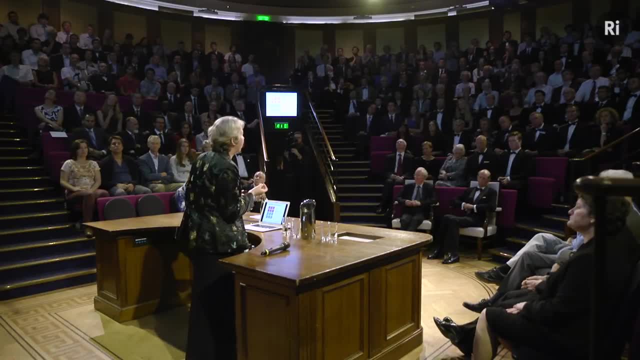 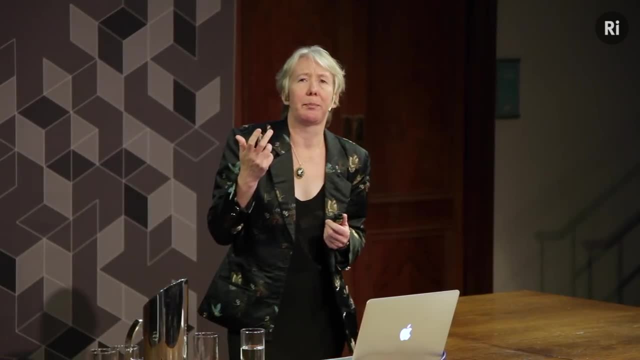 it's actually more convenient for us to use a unit of energy to measure the masses of particles, And I'm going to be using this unit through the lecture. So the unit we choose is an electron volt. That's the energy that would be picked up by an electron. 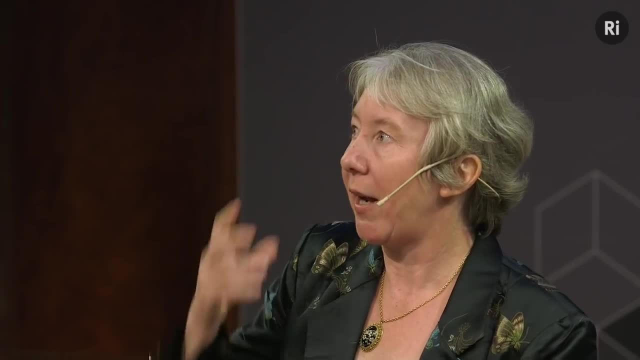 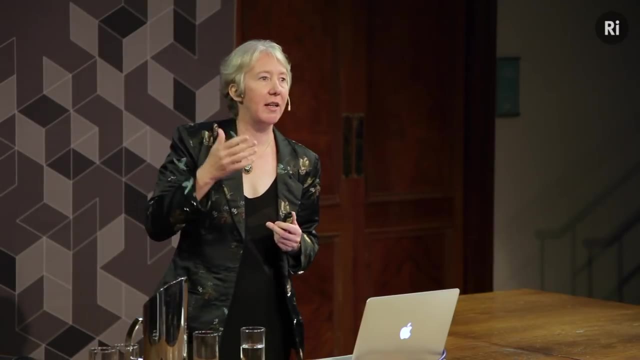 if you accelerated in an electric field through one volt And to get up to the mass of a proton you actually need a billion electron volts. So 10 to the 9 electron volts, a giga electron volt which we've written GeV. 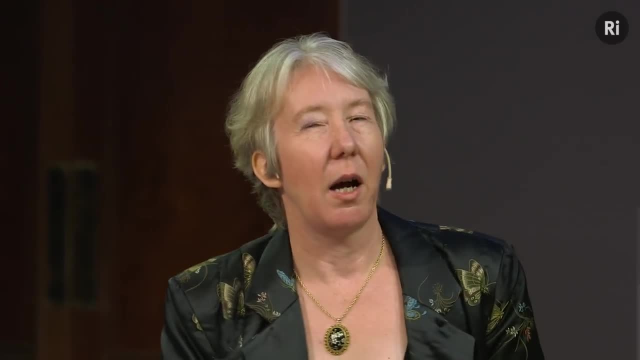 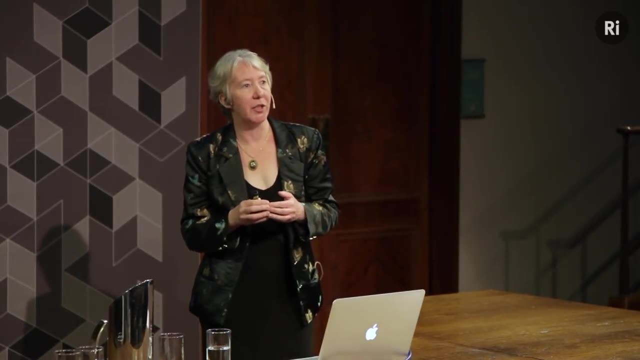 A proton has about one GeV. A top quark is 170 times more massive. It weighs 173 GeV. But we can make top quarks in our particle collisions and then, because they're one of the most massive particles, they're unstable. they decay immediately. 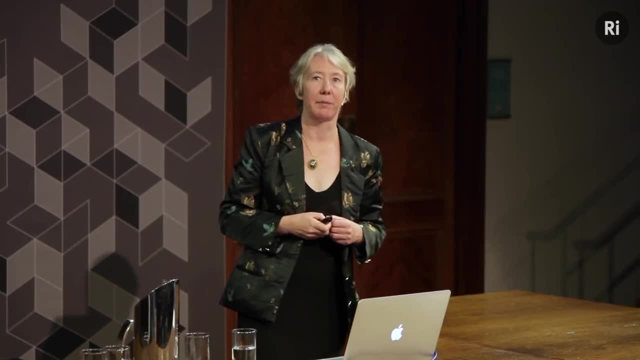 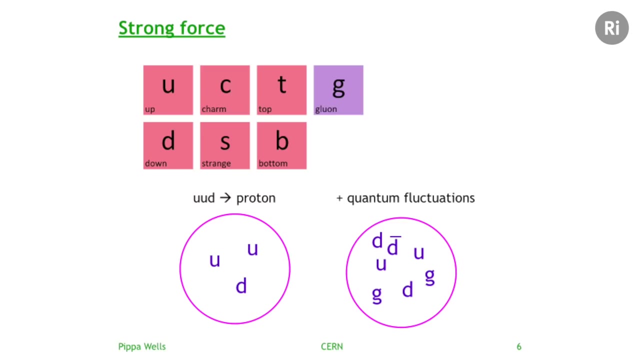 and we have to infer that they were there from the decay products. In the standard model, in our theory, forces are also due to particles. So the strong nuclear force that's binding together the protons and neutrons, that's carried by gluons G. 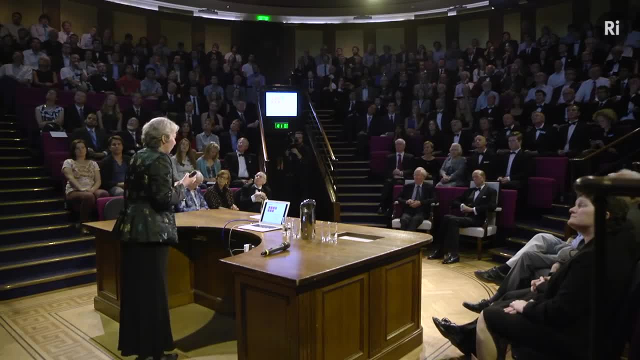 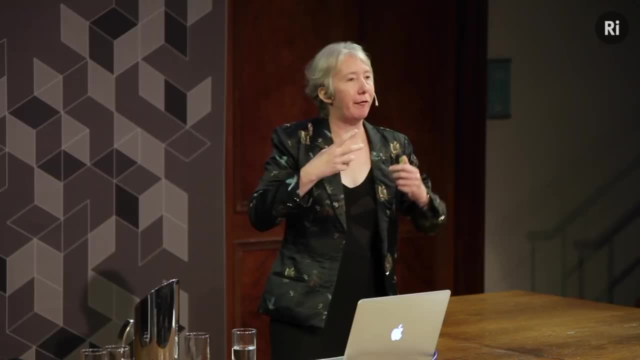 A different type of particle. It's a force particle, not a mass particle. So I told you that the proton had two up quarks and a down quark, But in reality, thanks to the fact that in quantum mechanics, forces are also due to particles, 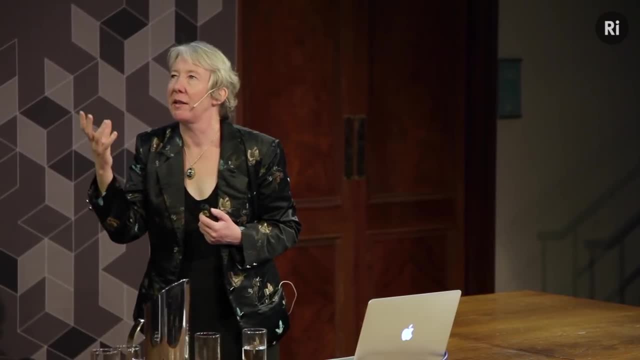 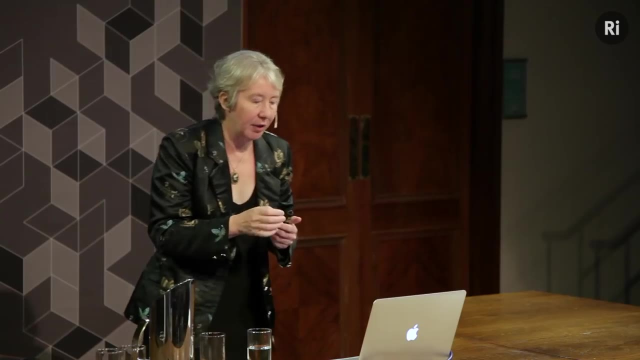 At any instant there are gluons winking out of existence. inside the proton They're being exchanged between the quarks. The gluon can even turn into a quark-anti-quark pair. So the D inside my sketch of a proton. 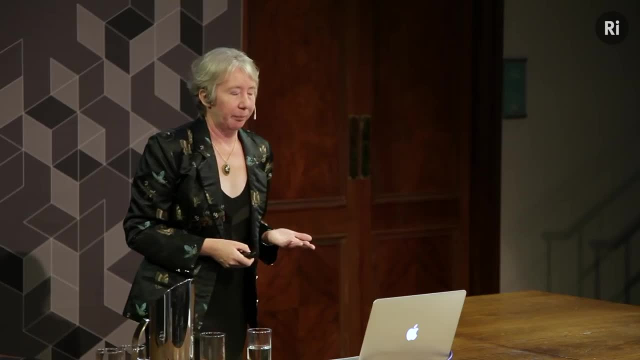 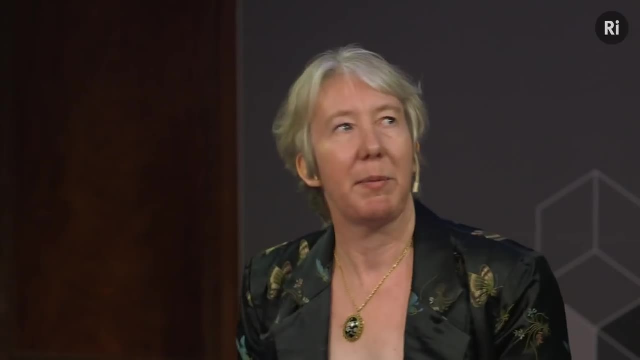 It has a bar over the top to indicate that's actually an anti-quark. So when we collide protons together in the Large Hadron Collider, it could actually be two gluons that we picked up. It could be a gluon-gluon collision. 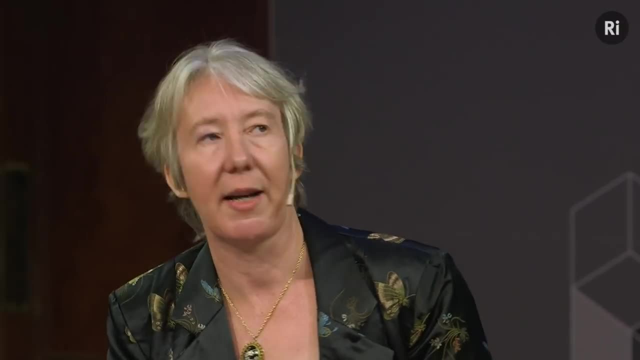 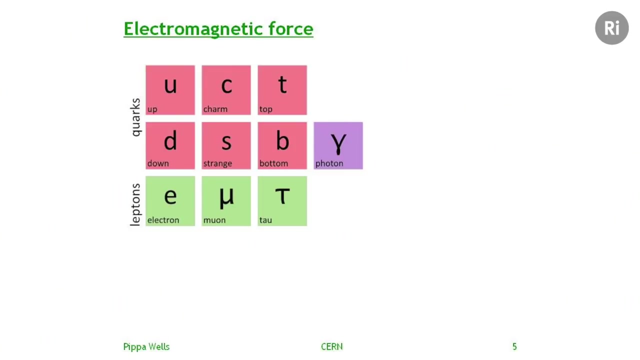 It could be an anti-quark hitting a quark. We just don't know what's going to happen. It's a statistical process. Then the electromagnetic force. I think we're all a lot more familiar with photons, That's the force particle of the electromagnetic force. 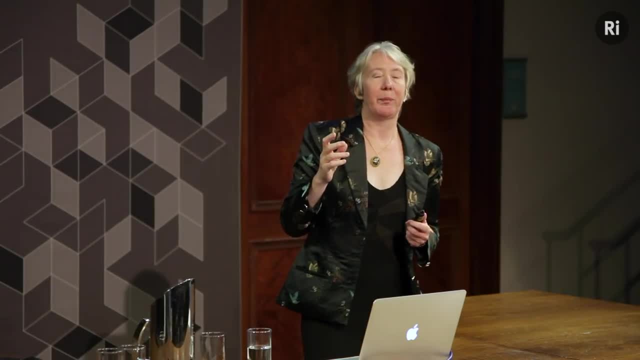 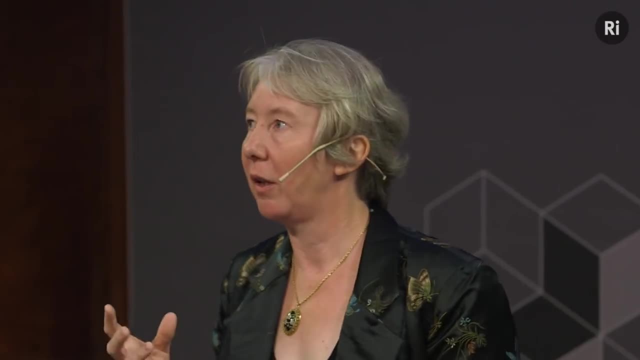 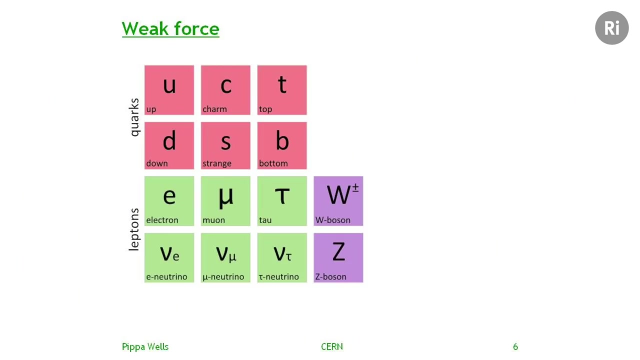 So photons are in light rays And it's a slightly simpler force than the strong force. All of the charged particles feel the electromagnetic force, And this was actually the first one that was worked out in quantum mechanics. Then there's the weak force, the weak nuclear force. 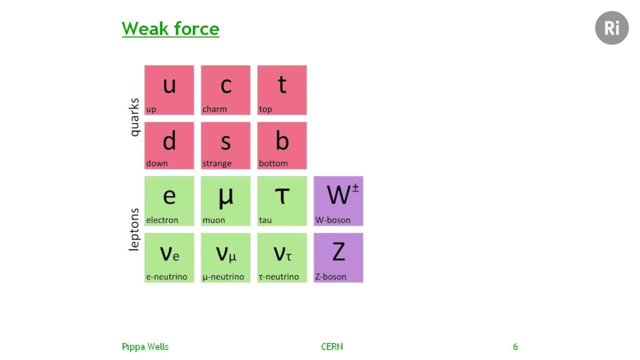 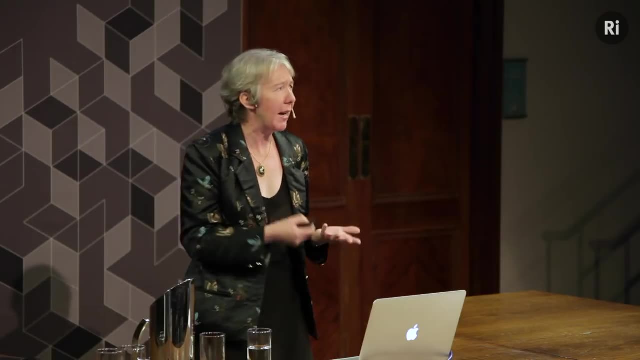 There's no actual reason why that should be any weaker than the electromagnetic force, apart from the fact that the two force-carrying particles, the W boson and the Z boson, are really heavy. The W is about 80 times the mass of a proton. 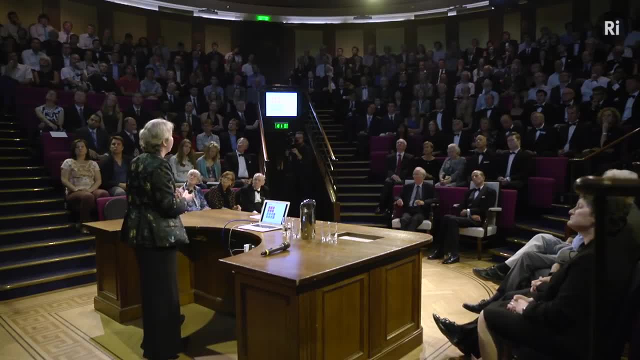 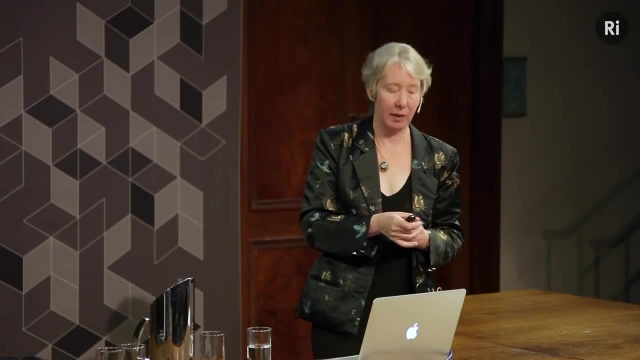 The Z 90 times the mass of a proton. So that's why the force is too weak In these quantum mechanical processes that cause the forces they've actually got to create these really heavy particles. And then we come to our first mystery. 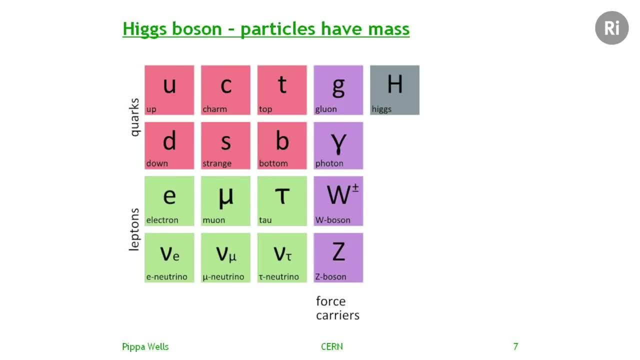 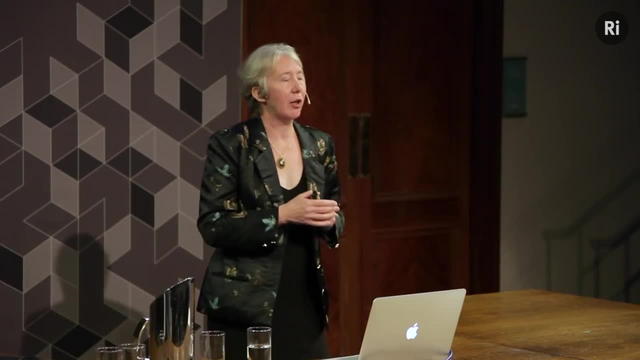 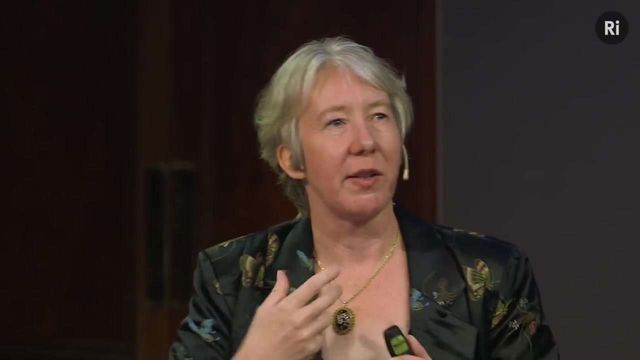 How do any of these fundamental particles get mass? And this was first understood about 50 years ago by several theorists. They understood that there could be a special field permeating all of space And when the particles move through this field, they interact with it. 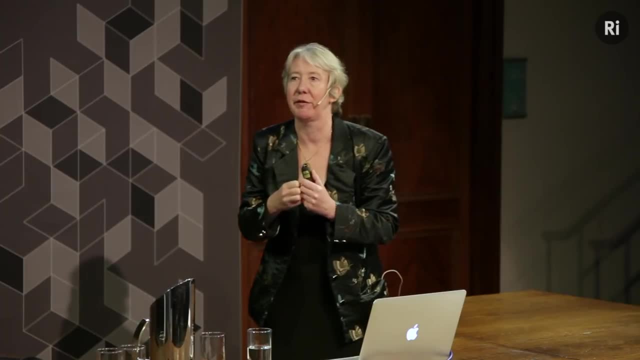 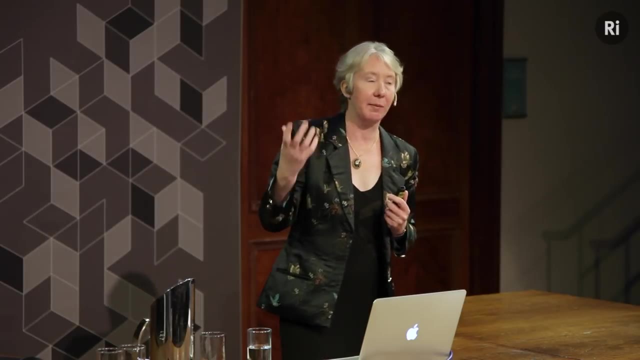 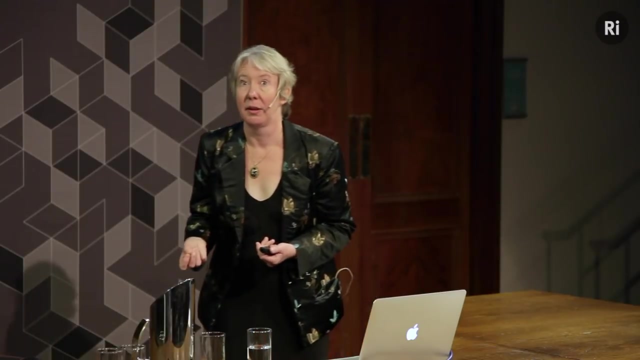 And the heavier the particle, the more strongly it's interacting with this special field. And Peter Higgs in Edinburgh was the one who pointed out that this field would also have a particle associated to the Higgs boson. So if this whole mechanism is going to work, there has to be a Higgs boson. 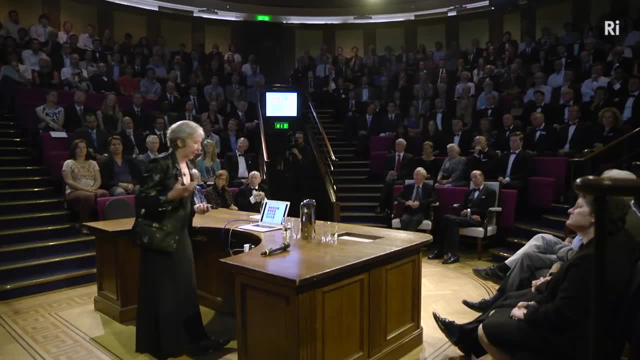 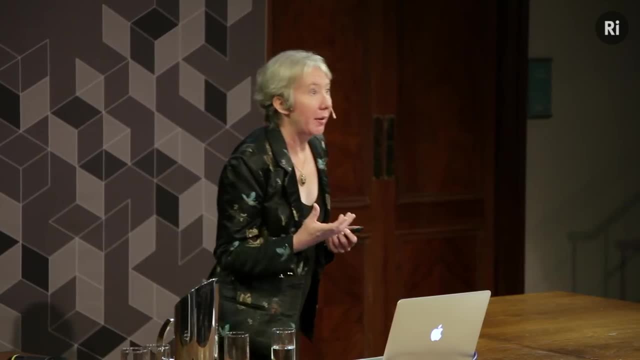 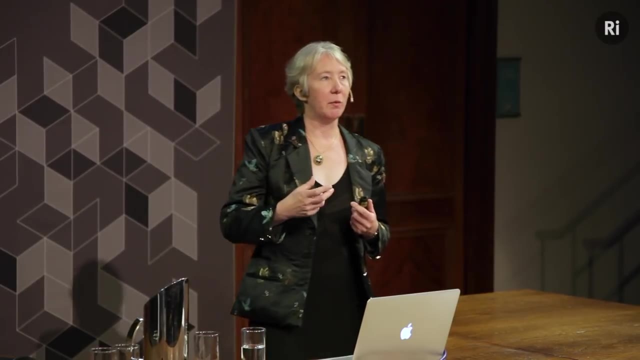 Now, over the last decades this standard model of particle physics has worked superbly well. The W and Z were predicted by the theory and then they were observed at CERN in 1983.. Then in the 90s CERN was operating the LEP collider. 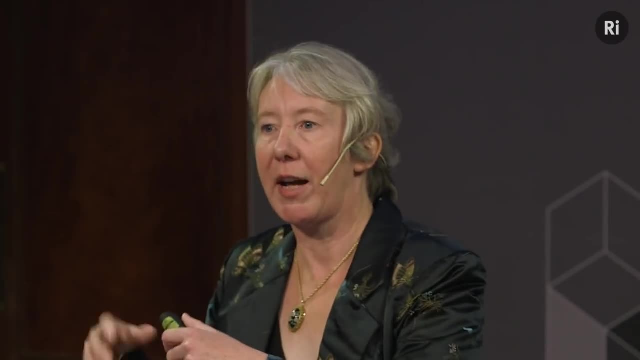 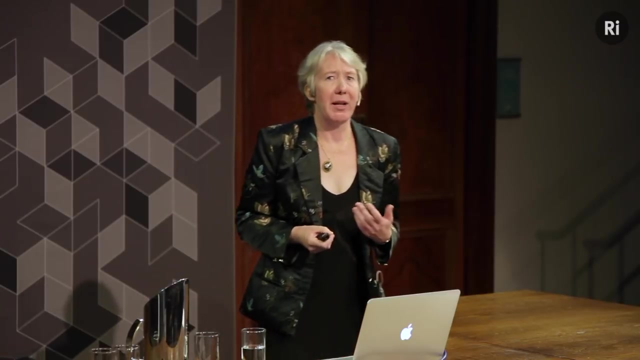 That's the Large Electron Positron Collider, And it used the tunnel that's now the LHC tunnel. It was the first accelerator in that tunnel. The LEP experiments measured the properties of the W and Z bosons to great precision- one per mil precision. 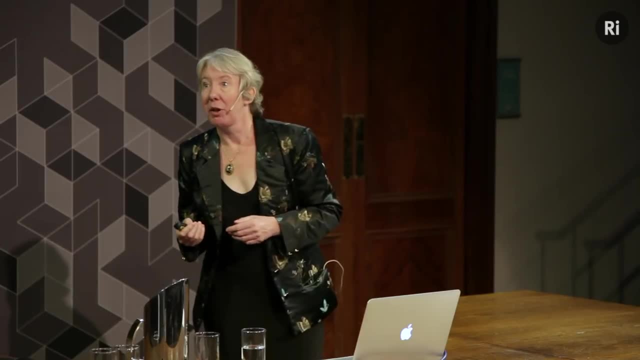 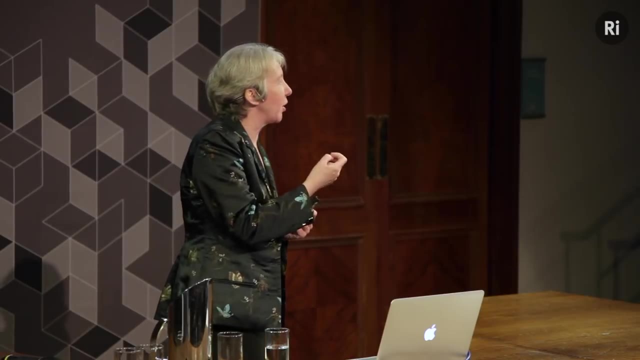 Everything fitted together And even more remarkable. at the same time, the Tevatron Collider near Chicago discovered the top quark And the mass of the top quark was just right. It fitted in precisely with the measurements that had been at LEP. 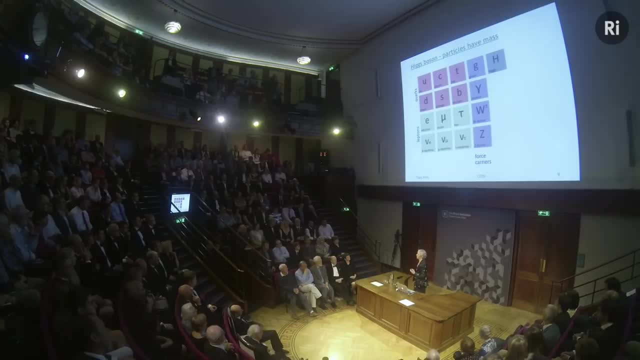 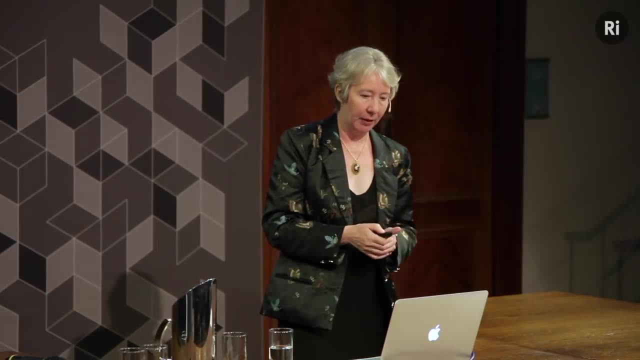 Everything worked perfectly, but where was the Higgs boson? So this was the situation when we were about to start the LHC: The theory worked beautifully, but there was still no sign of the Higgs boson. But there are other mysteries if we want to understand the history of the universe. 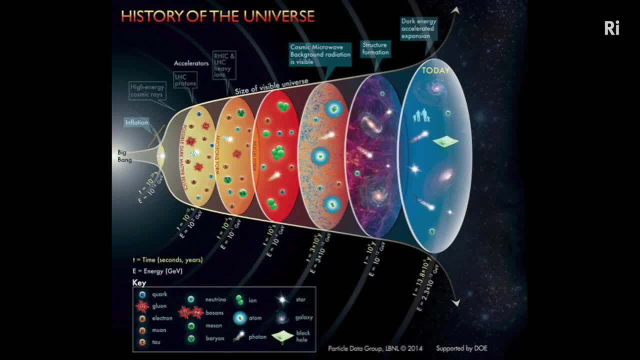 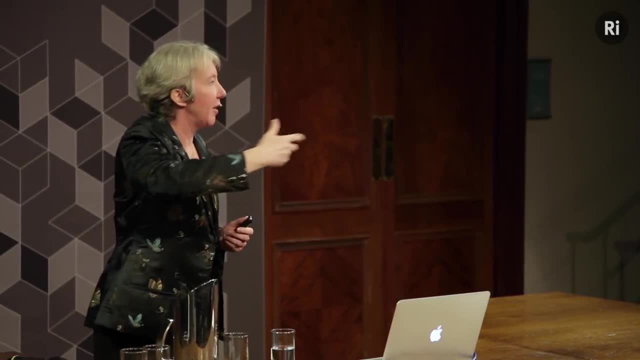 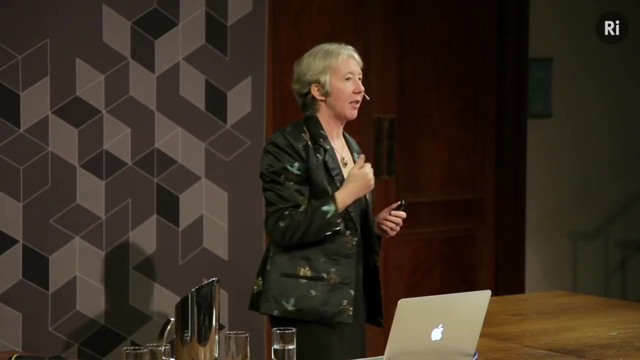 the evolution of the universe. I think it's well established that the universe is expanding from observations that have been made of distant stars and galaxies. So if you look out in space at a distant object- because the light takes some time to get to us- 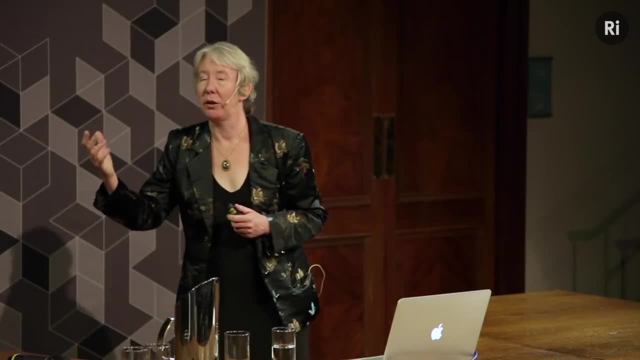 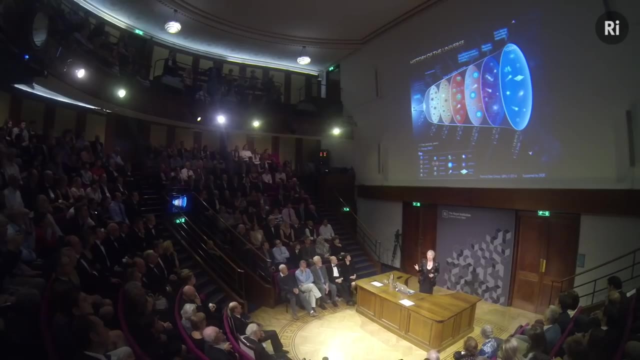 the further away the object, the further back in time you're looking. you're actually looking back towards the Big Bang. The universe is about 13.8 billion years old And you can start to look back towards the Big Bang And then you hit an opaque wall. You can't get any further back. You can get back to a point about 300,000 years after the Big Bang. That's the point when the universe had expanded enough and cooled enough that photons could actually travel freely. Light rays could travel freely. Before the Big Bang the universe was just too dense. Atoms hadn't even formed, And even when atoms had first formed, the universe was still a little bit too hot. But eventually the photons decoupled And this was like the last afterglow of the Big Bang. 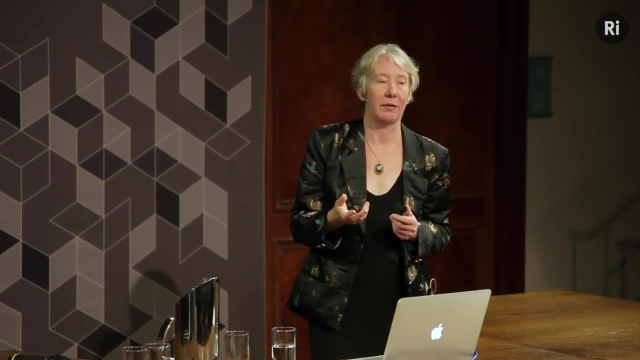 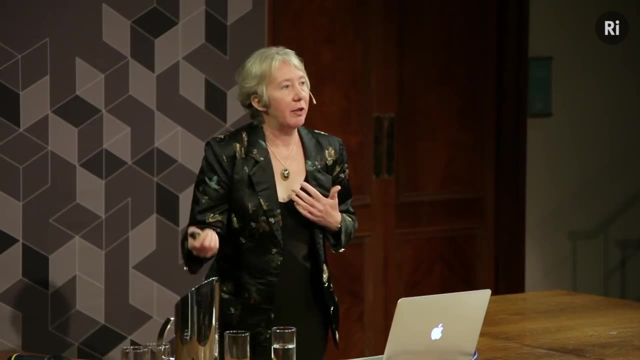 And we can still see that today. That's the cosmic microwave background that we can observe today with radio telescopes. So if you want to understand how the universe got in that state, you need to understand what was happening just after the Big Bang. 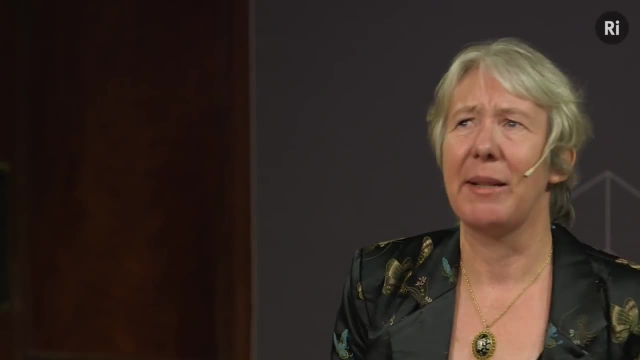 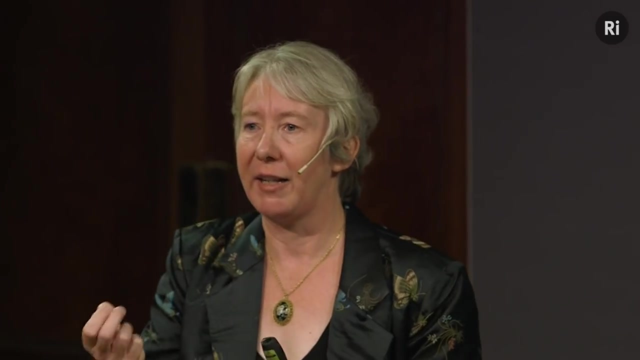 If you want to understand why we're made of matter and not antimatter- what's this dark matter that you might have heard of? You have to run collider experiments. You have to try and recreate the very hot conditions at the start of the universe. 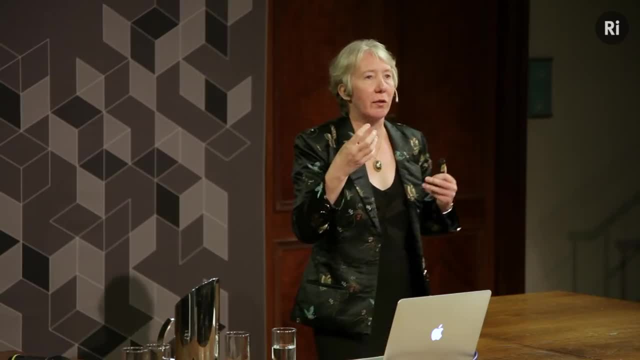 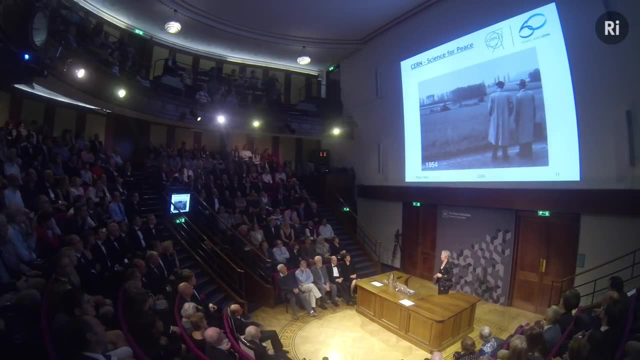 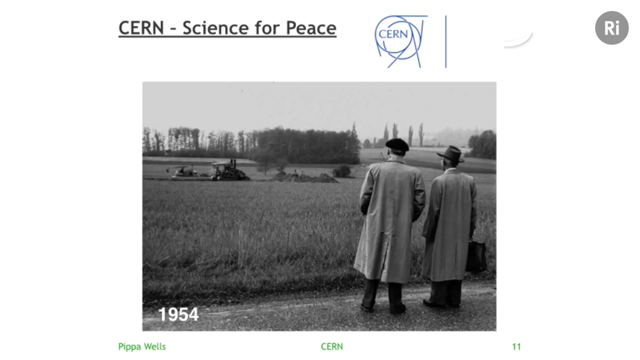 So, instead of using telescopes and looking out, you can think of the LHC as a sort of super microscope for looking in finer and finer detail. CERN was founded 60 years ago with the aim of doing science for peace. So Europe was coming out of the war. 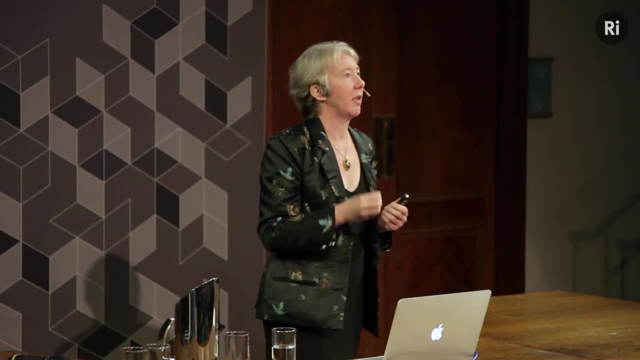 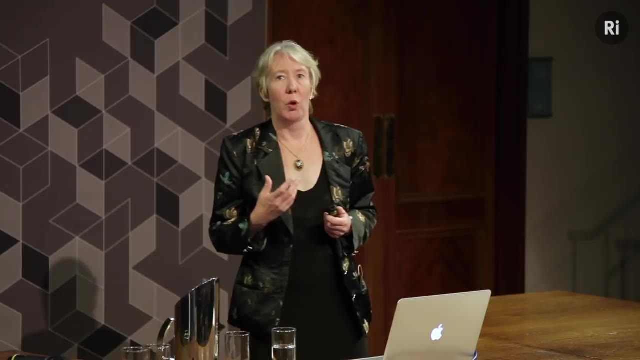 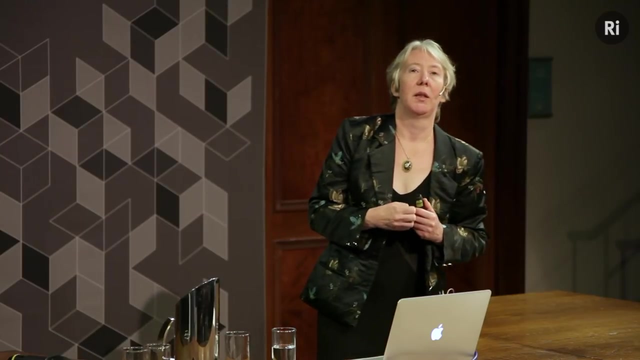 A bunch of European nations signed a treaty to start doing science for peace, trying to understand subatomic particles. So the aim of CERN was to build accelerators to accelerate particles, try and start to understand substructure of the atom better and better. 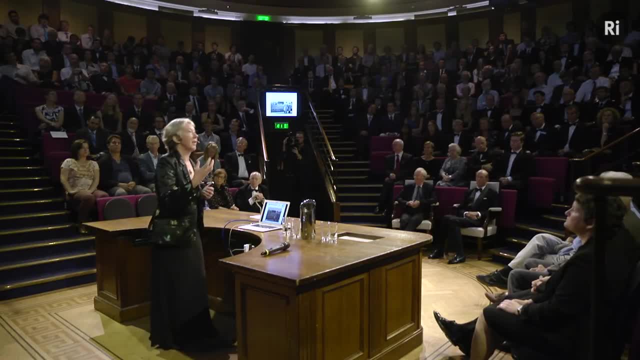 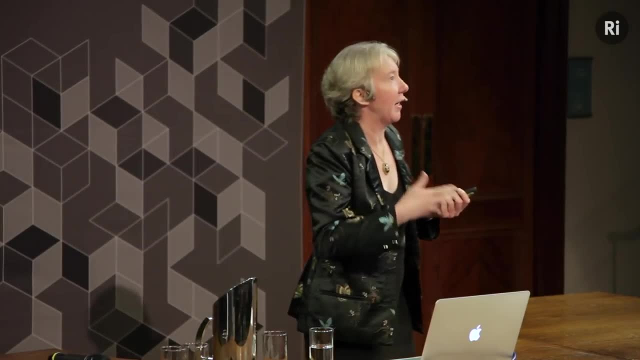 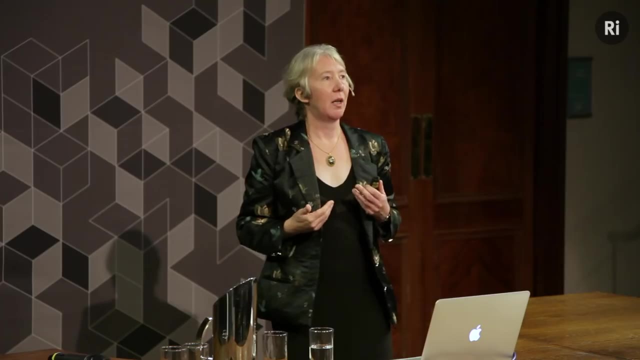 So to build accelerators and to build the detectors to look at the products of accelerator experiments. CERN had to innovate. So to do fundamental research, it had to innovate and build its own technologies And then it had to bring people in and educate them in those technologies. 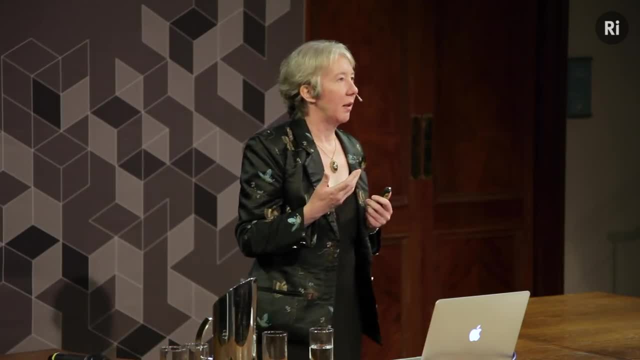 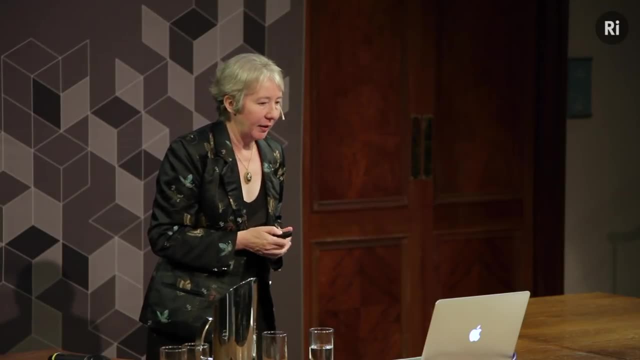 to be able to take the next steps. And in all three of those activities CERN was uniting people from across Europe and across the world to do science for peace. But I think these people watching the very first excavations at CERN would have been astonished. 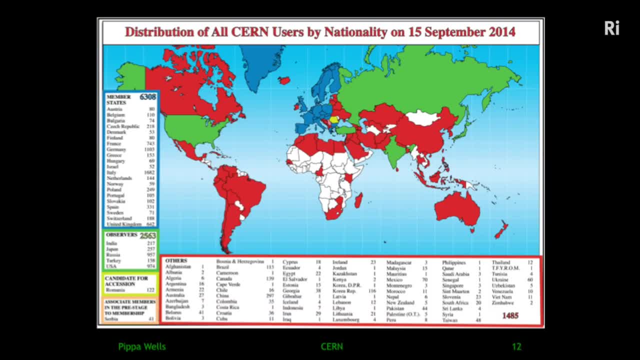 to see this. This is a map telling you where all the scientists come from who are working at CERN. today. There are over 10,000 scientists who come to do experiments at CERN, So there are a few of us- 2,000 people employed by CERN. 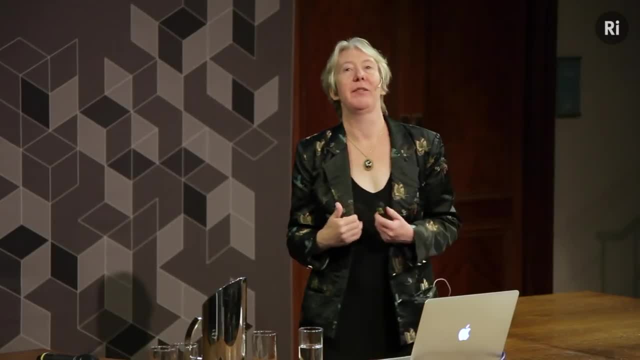 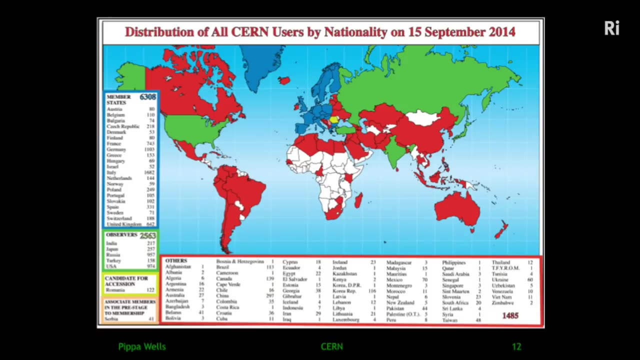 and then another 10,000 who visit to do the experiments. The countries that are coloured in blue: those are the member states of CERN, So they're mostly European. The UK was one of the founding members and is still a member. 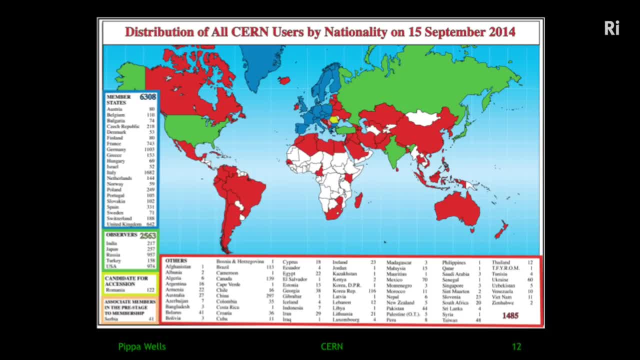 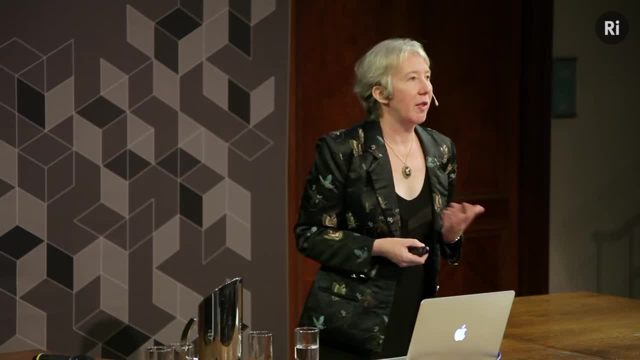 The countries that are coloured in blue, the countries in green. they're countries that have made a particular contribution in the recent years to the LHC programme and so on, and they have observer status. There are more than 600 scientists from the UK alone coming to work at CERN. 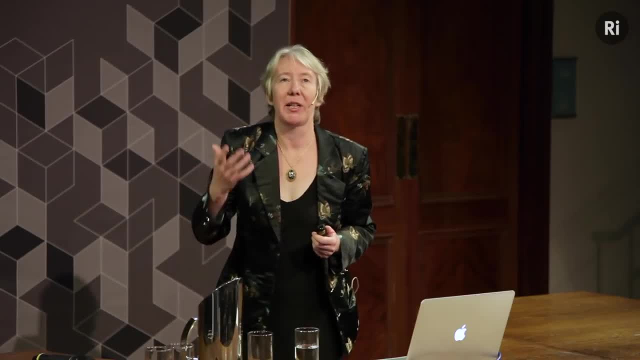 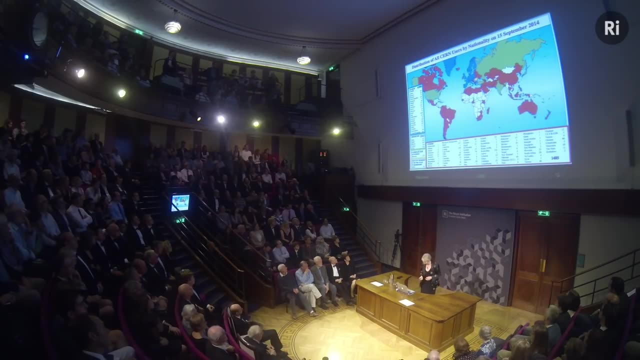 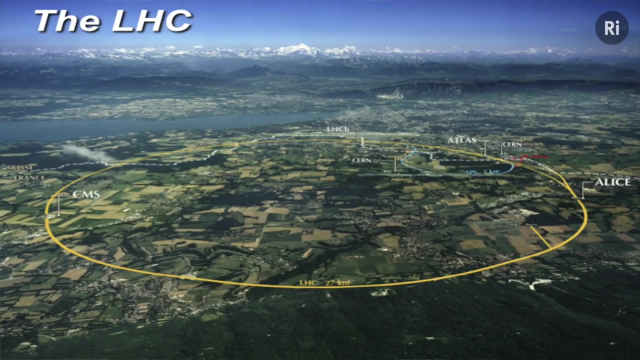 And we have people from across the world. We have Indians and Pakistanis working side by side to do science. We have Chinese and Taiwanese working together on the same experiment. So the LHC is the tool that we're going to be using, If you ever get a chance to see this aerial view. 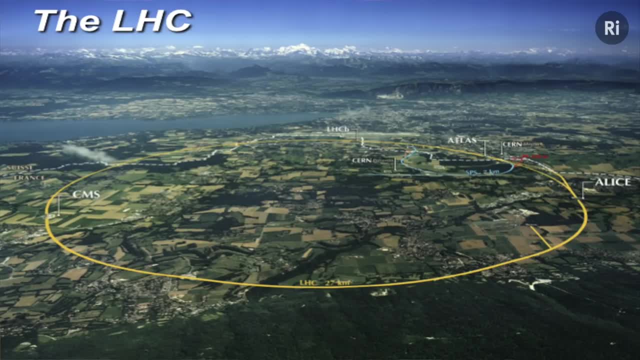 you can't actually see the LHC ring. It's typically 100 metres underground. You can pick out a few of the surface buildings that are associated with the experiments. In the background of this picture, you can see the Alps with Mont Blanc in the middle. 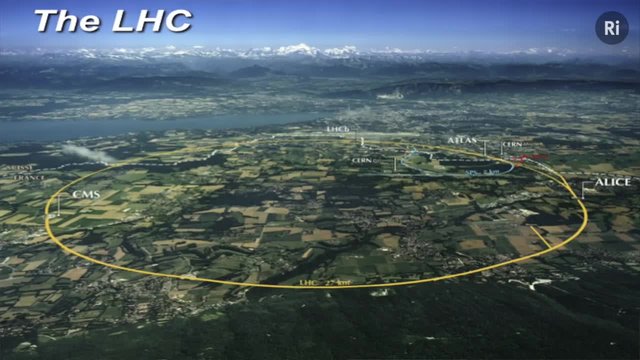 Then you can see Lake Geneva between the Alps and the LHC ring, And you can also pick out the airport runway to get an idea of the scale. So my experiment: ATLAS is close to the CERN main site. ATLAS is a general purpose detector. 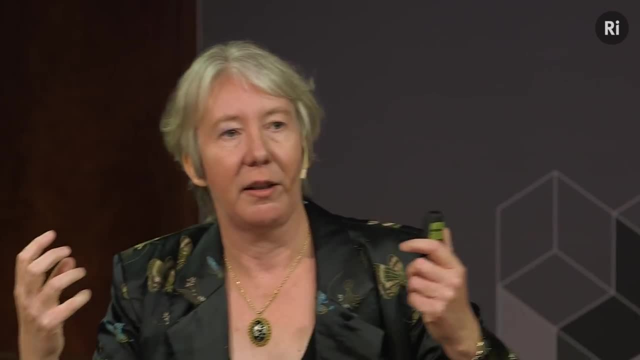 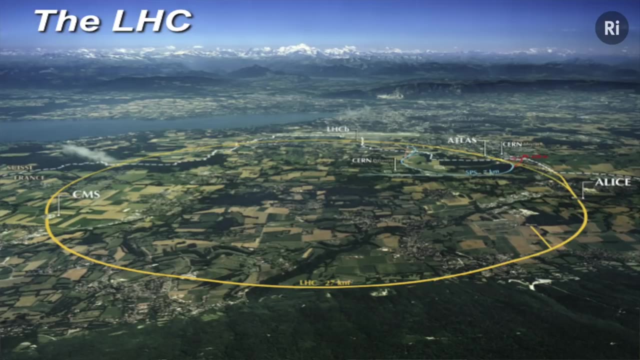 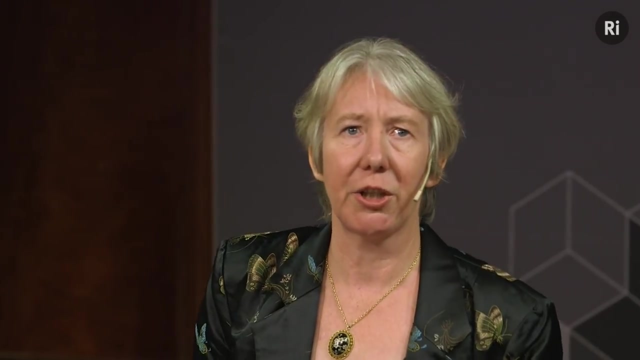 It wants to pick out all the particles that are made in the collisions, And there's a similar general purpose detector on the other side of the ring called CMS, And today I'm mostly going to talk about the work of ATLAS and CMS. There are two other large experiments. 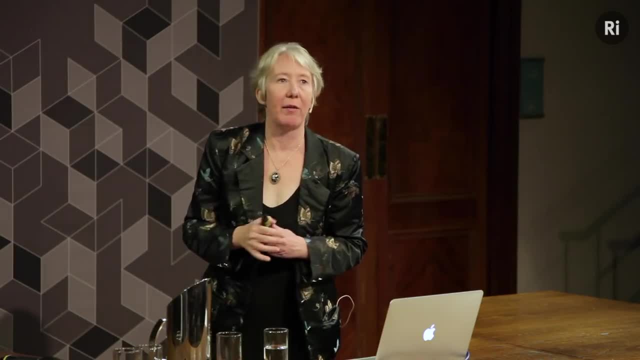 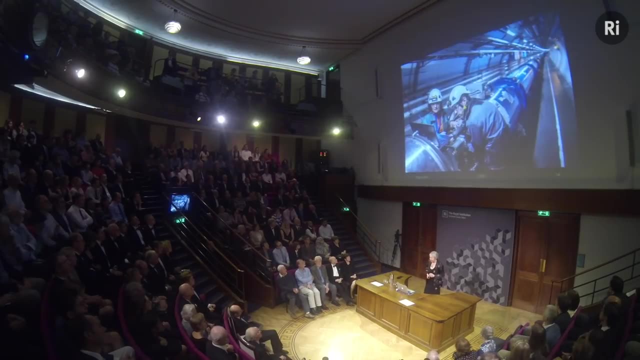 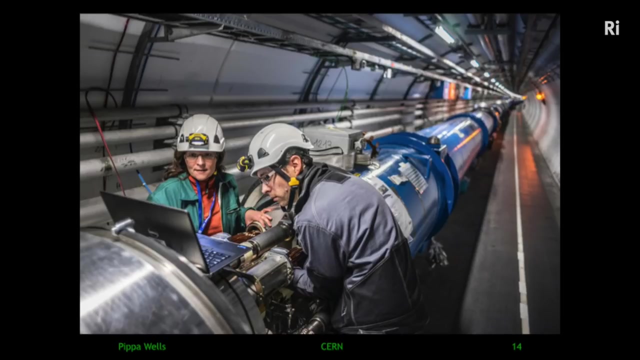 LHCb and ALIS. I will mention them briefly. They have a more specific target in terms of addressing mysteries Inside the LHC tunnel. it's quite a small tunnel. there are these blue tubes, blue boxes, cryostats. 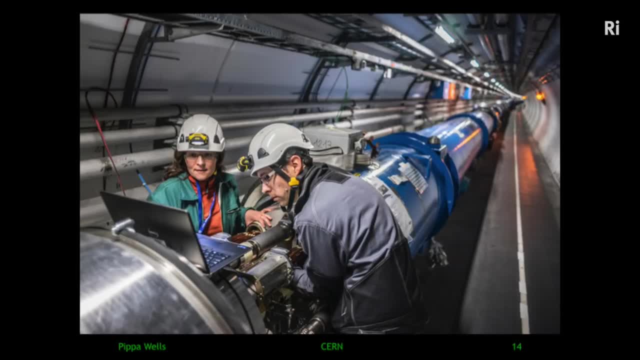 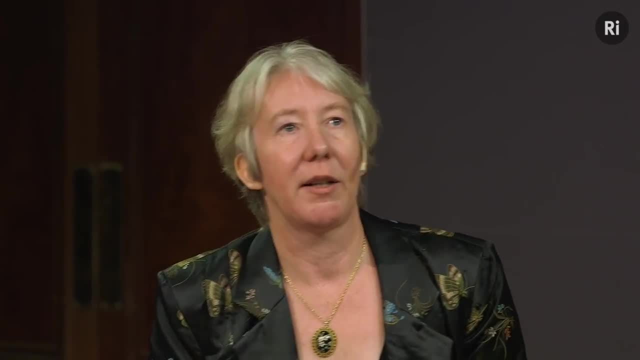 They hold the superconducting magnets that actually bend the high-energy beams around this 27-kilometre pass. Inside each magnet there are actually two tubes not so big a few centimetres across, And these two tubes are on a very, very high vacuum. 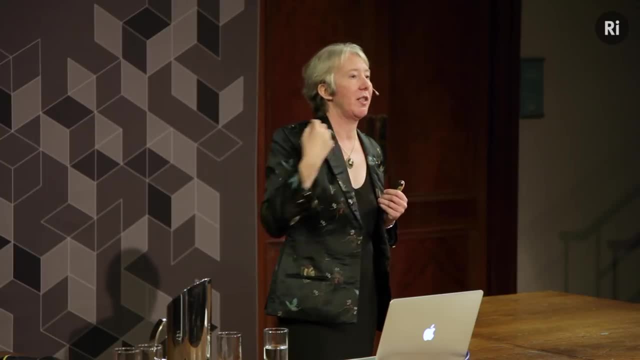 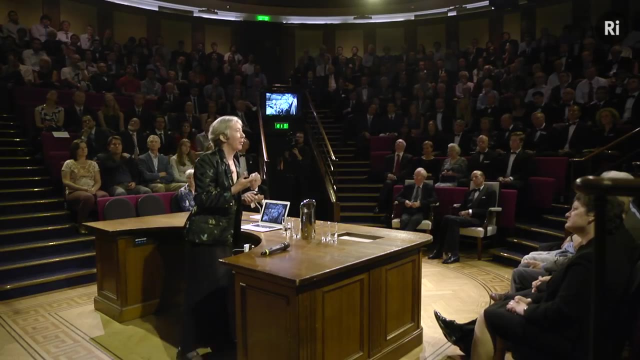 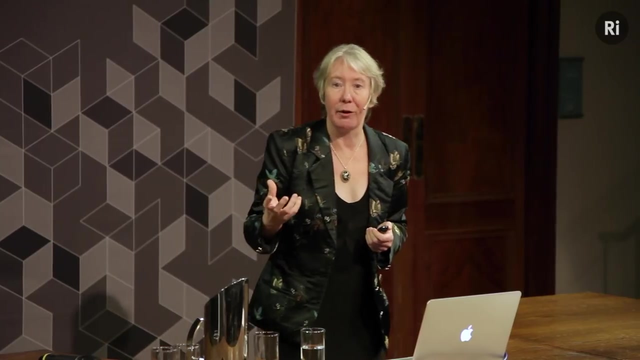 That's the tubes that the beams actually circulate around in. When we started the LHC in 2008, you probably remember there was a problem. There was one of the interconnects between these superconducting magnets actually burned out when we were doing the final stages of testing. And that was a problem. So we did eventually restart in 2009,. but we couldn't run at full energy. The full energy of the LHC collision energy is 14,000 GeV, So 14,000 times the mass of a proton. 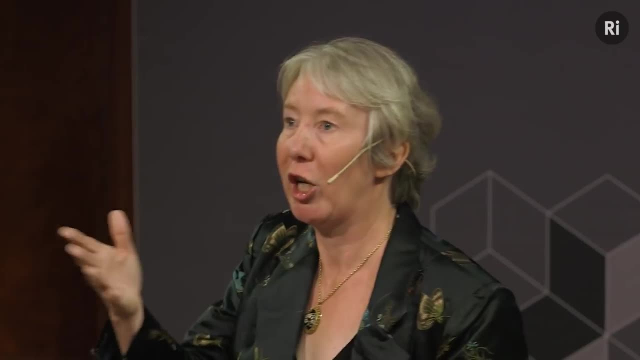 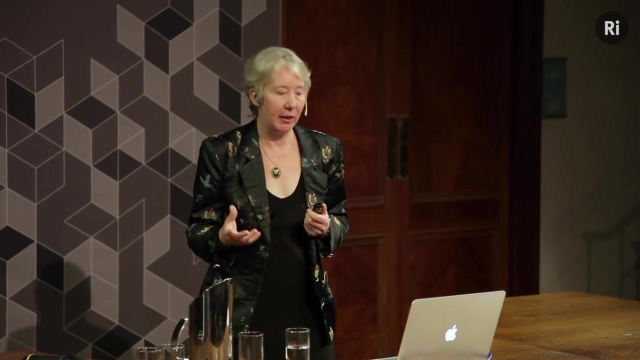 We call it 14 tera electron volts, 14 TeV, But for the last few years we had to run at about half that energy, seven or eight TeV, And now we're in the middle of a long shutdown, One of the things that's been going on. 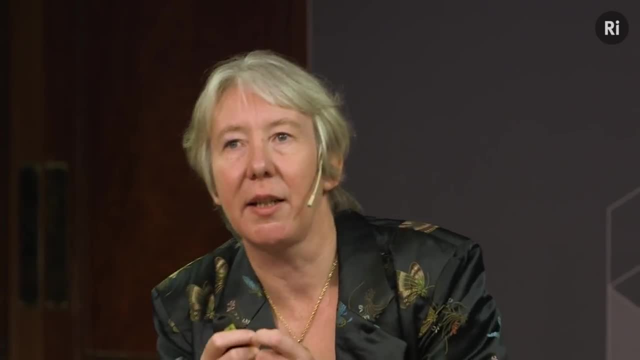 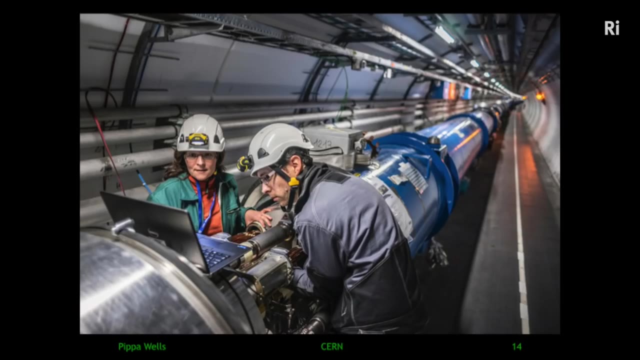 is to repair and strengthen the interconnects between all the magnets. These two people, these two engineers, are checking that one of these repairs has been done properly so that when we restart next year, in 2015,, we'll actually be able to run at design energy. We'll be able to go up to full energy of the collider. The particles in the beams are not coming continuously, They're actually in bunches. The bunches are a few meters apart because the beams are circulating at nearly the speed of light. 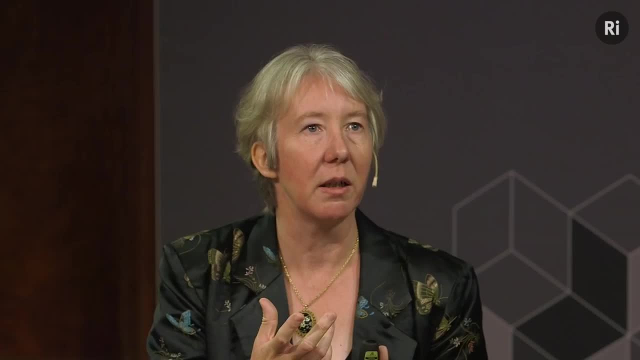 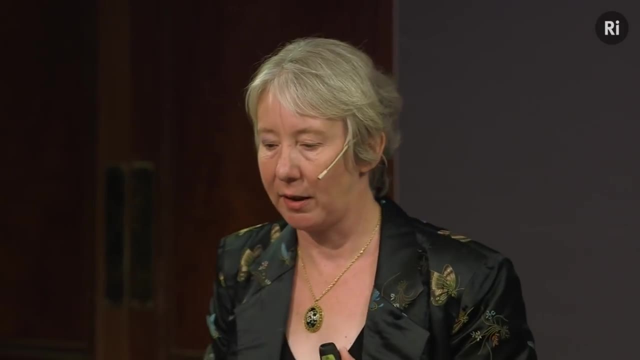 The bunches actually collide every 25 nanoseconds, so that's 40 million times a second. The big detectors like ATLAS and CMS have to take a picture of the collision- 40 million pictures a second- And the experiments also use magnets. 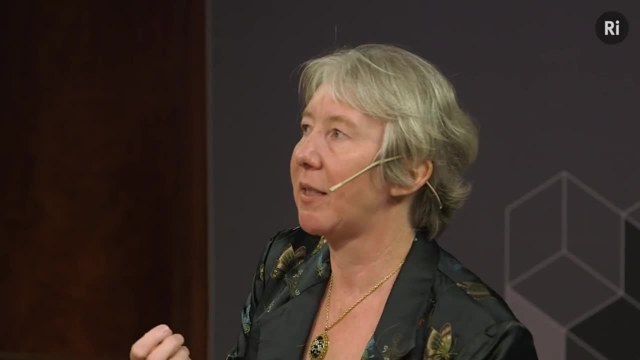 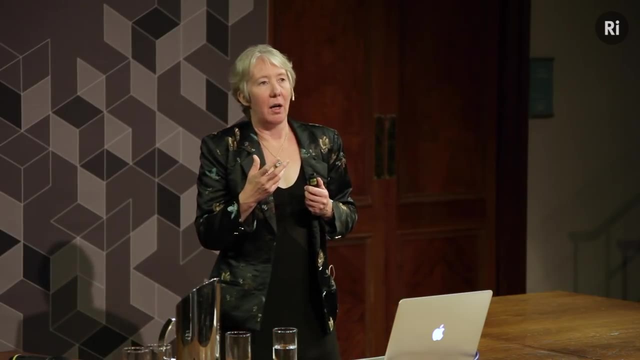 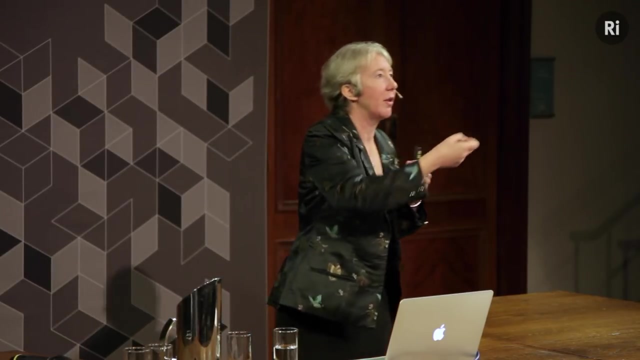 but in a different configuration. The experiments use magnets to analyze how energetic the particles are that come out of the collisions, and the higher energy the particle, the harder it is to bend in a magnetic field. So if a particle has a fairly straight path, 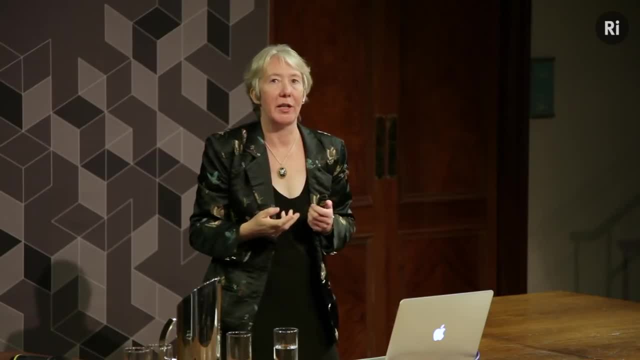 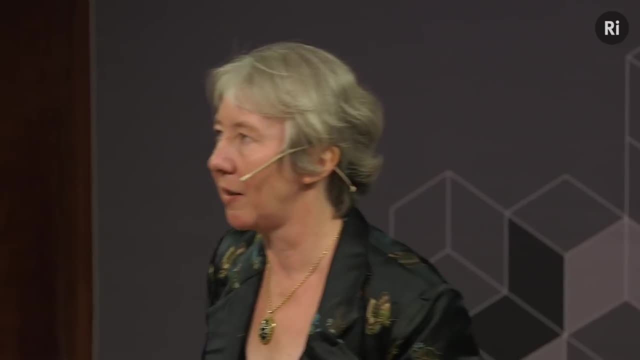 you know, it's a high-energy particle. If it has a curved path it's a lower-energy particle. And the choice of the magnet layout is the biggest difference between the two experiments, ATLAS and CMS. Here's a picture that was taken: 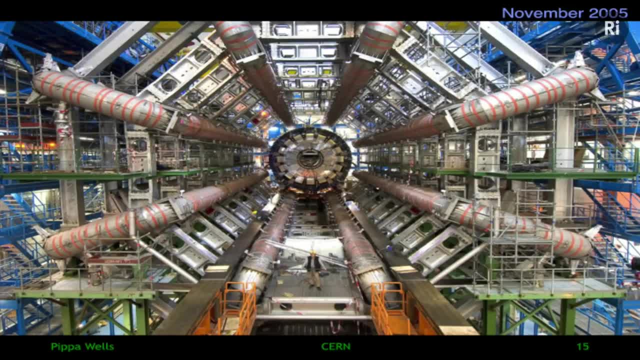 of the ATLAS detector in 2005,, when we were in the process of putting it together. These tubes contain- each one contains- a superconducting coil to make a big toroidal magnetic field that wraps the whole way around the detector- a doughnut-shaped magnetic field. 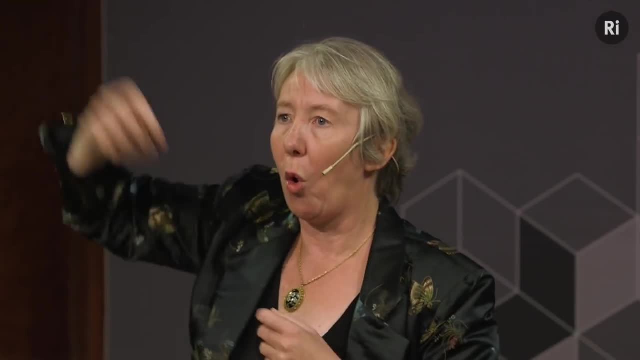 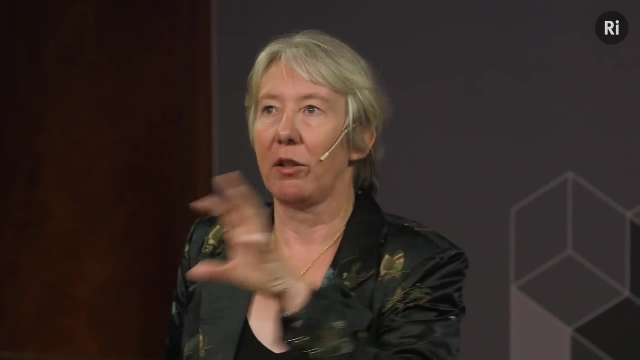 so that we can analyze the energy of particles that emerge all the way out of the apparatus. If you get a chance to visit ATLAS, you won't really be able to see this glorious open space anymore, because we've filled it all with detector elements. 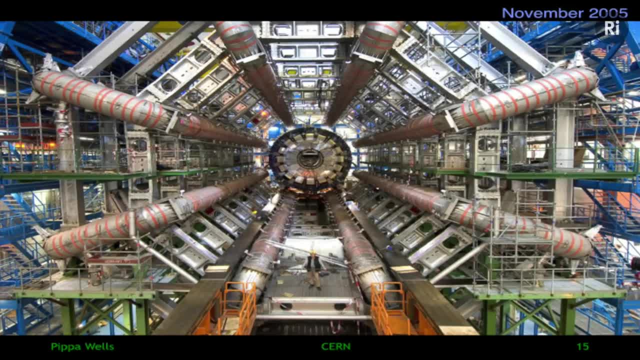 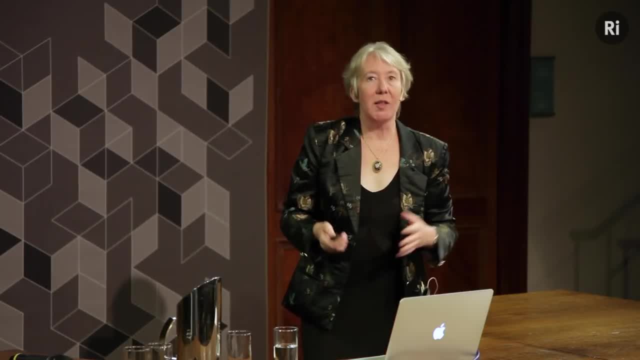 At the back. here you can see a piece that's about to be slid in along the rails to take its place in the center of the detector. So because if you actually take pictures, everything's filled up with the detector elements, I'll actually show you. 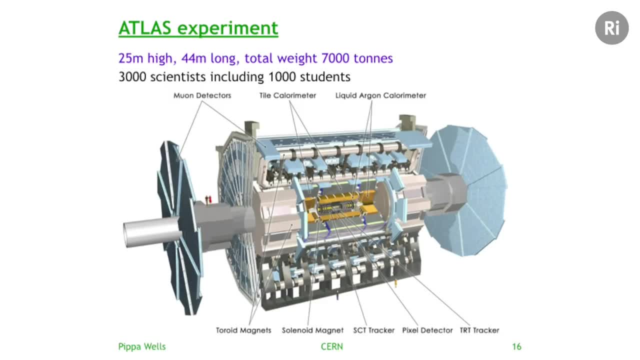 a cutaway cartoon of ATLAS instead, So you have to try and imagine this. It's 25 meters high, 44 meters long, It weighs 7,000 tons And, what's more, it's a collaboration of 3,000 people who managed. 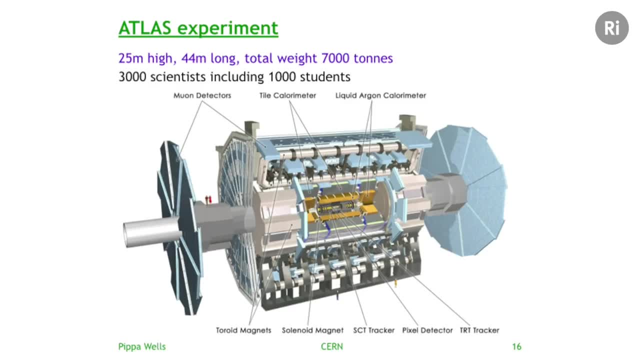 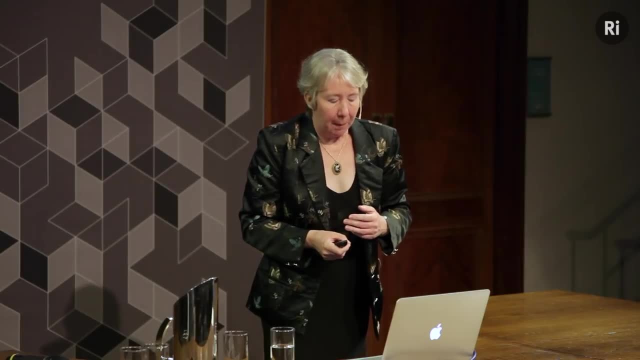 to design this thing, build all the pieces, put them together and have them fit and work synchronized- 3,000 people, 1,000 of whom are actually PhD students. The two beams are coming in from the two sides of the apparatus. 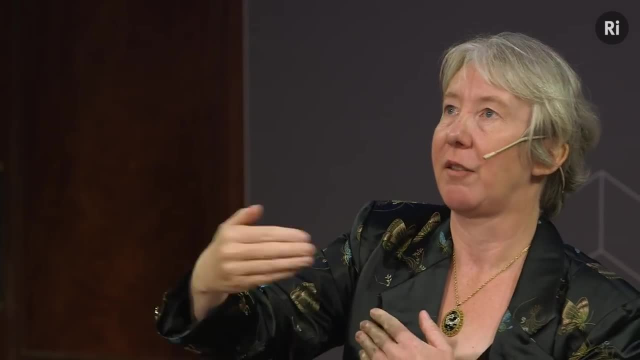 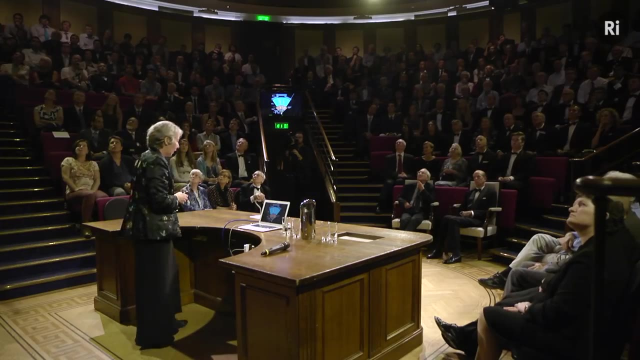 and they collide in the geometric center. And then there are layers of detector elements, And it's easier to explain that in this next picture, which is actually a sort of cutaway view, a slice. So in this view the beam is in the center. 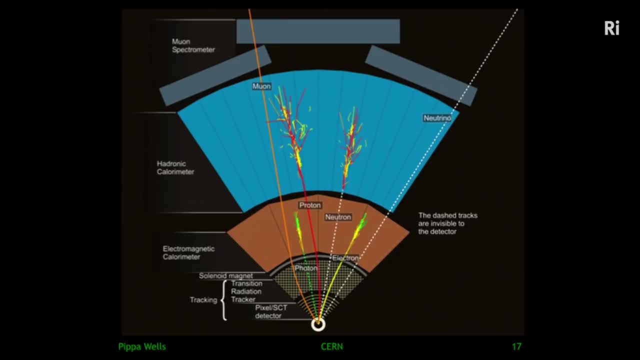 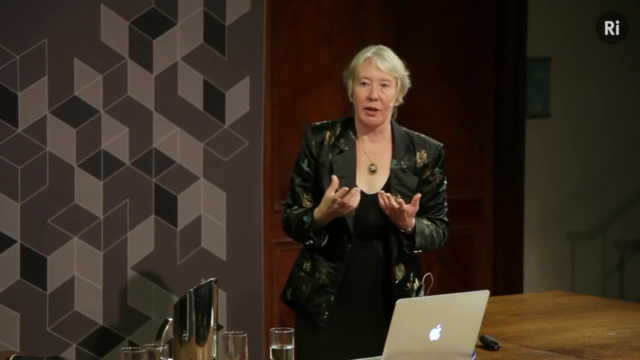 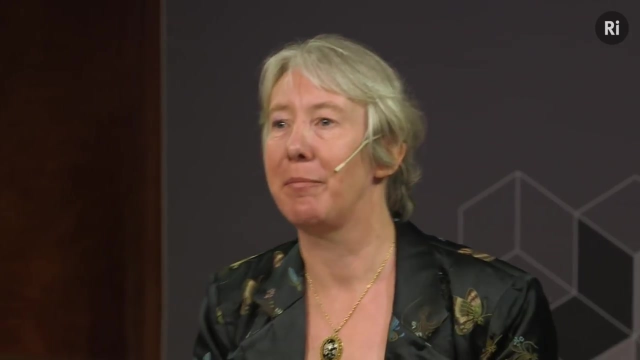 And then there's a pipe to keep the vacuum chamber where the beams are going through, And then the closest detector elements are just a few centimeters away from the collision point, And most of the electronic channels of the detector are actually in that center part. 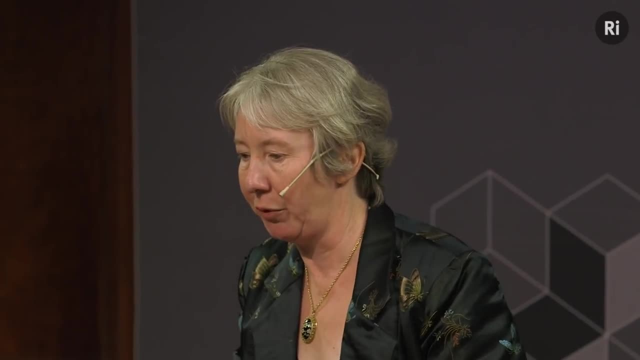 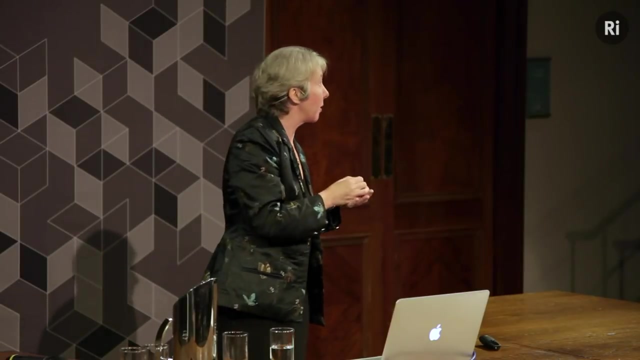 It's the spot I worked on the tracking detector. It measures the tracks of charged particles as they emerge from the collision point And most of the electronic channels of ATLAS 80 million channels. there are 100 million channels altogether in the whole detector. 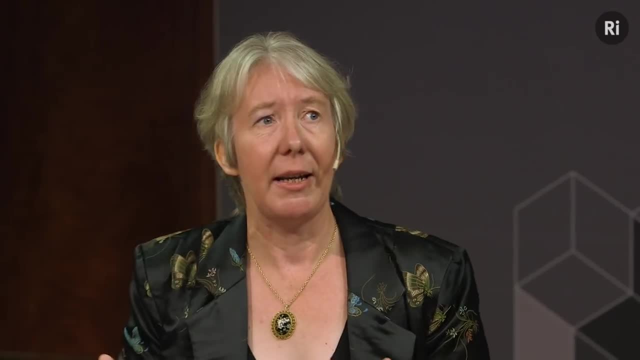 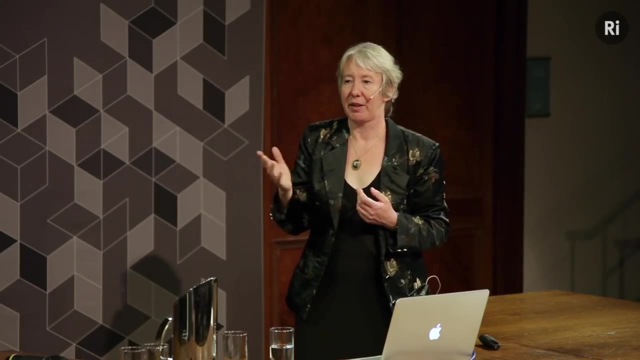 That sounds a lot, but if you go out to a shop you can buy a 10-megapixel camera. a 20-megapixel camera, So 100 million channels. that's actually just like five cameras. But we've got to take. 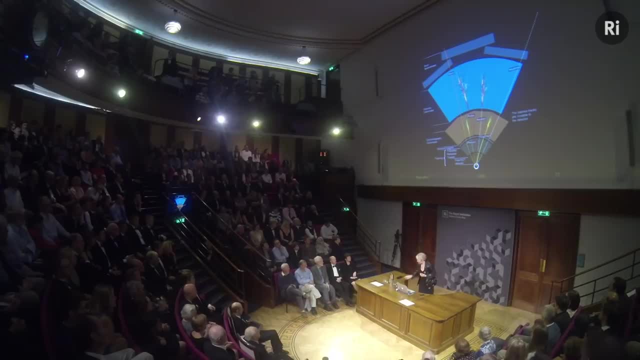 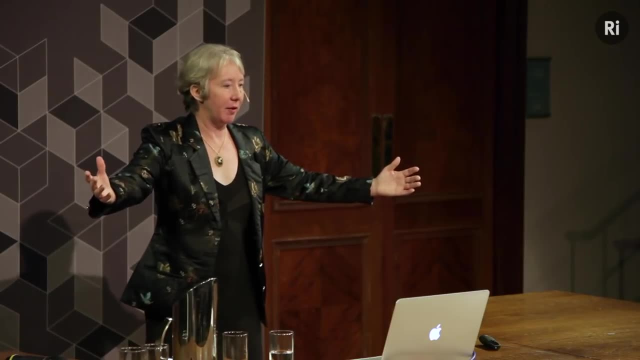 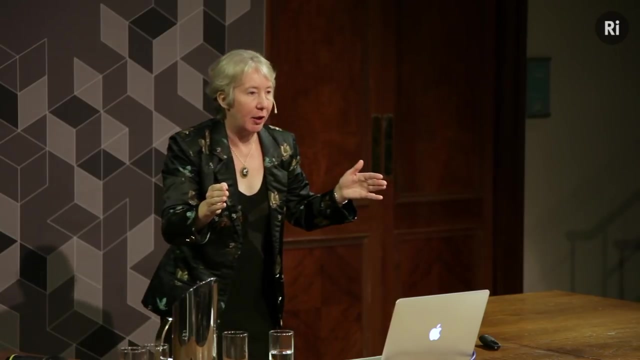 40 million pictures a second. That's where the clever part comes in. So the charged particle tracks are emerging from the center of the detector. We can measure them from the table And the ones that are charged, we can measure a trace from them. 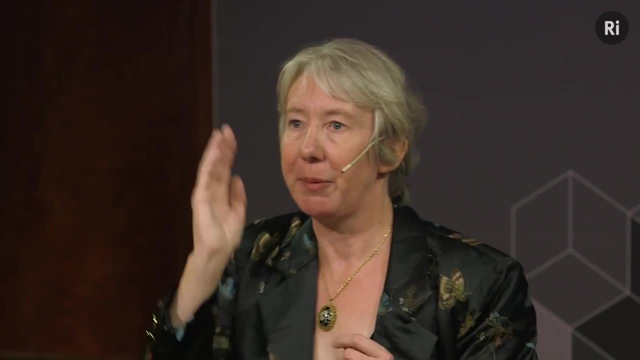 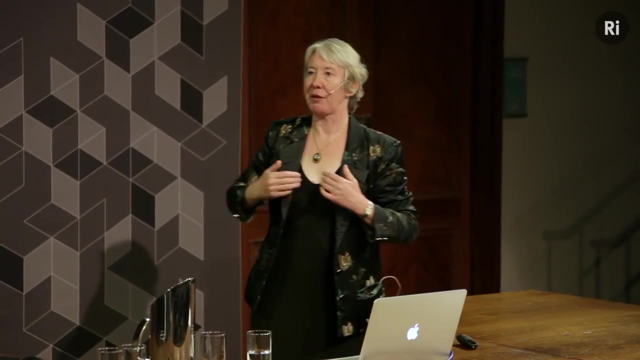 Then there's a magnet, So even in the center part the particles are curving. The high-energy particles are the straighter ones. Then the next layers are calorimeters, That's energy measuring equipment, And that would fill up the space from here. 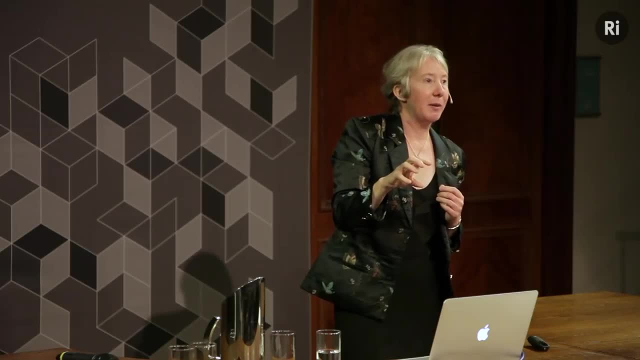 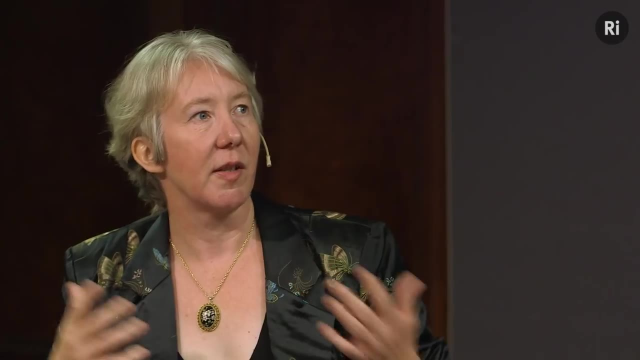 to like the second or third row. That's all. It's very, very compact, very dense. The inner part of the calorimeter measures electromagnetic particles like electrons or photons, Hadrons like neutrons or protons. So you can already start to think. 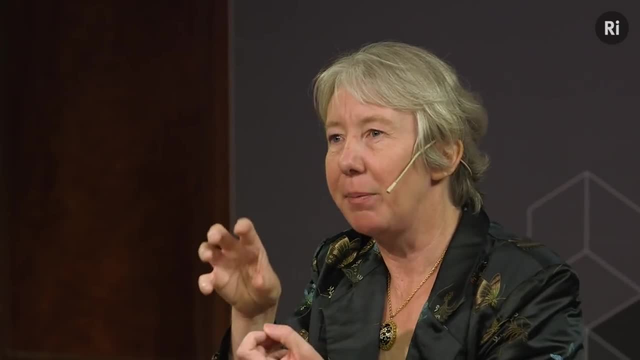 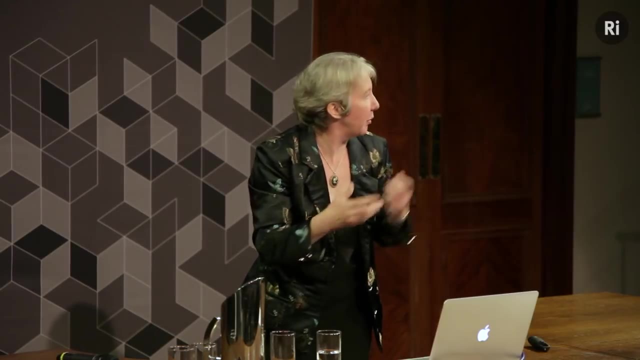 If I've got a charged particle in an electromagnetic energy deposit, that's probably electron, If I don't see any track and I've got an electromagnetic energy deposit, that's probably a photon, We're sort of piecing together. what are the particles? 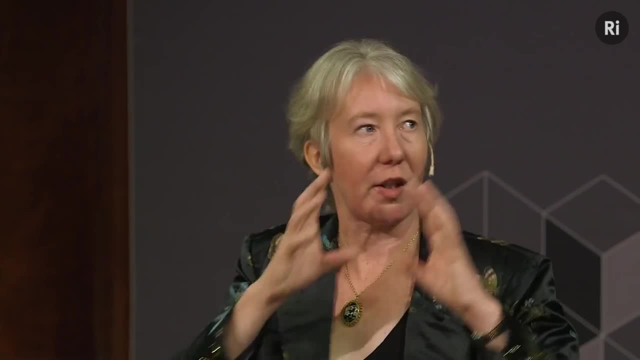 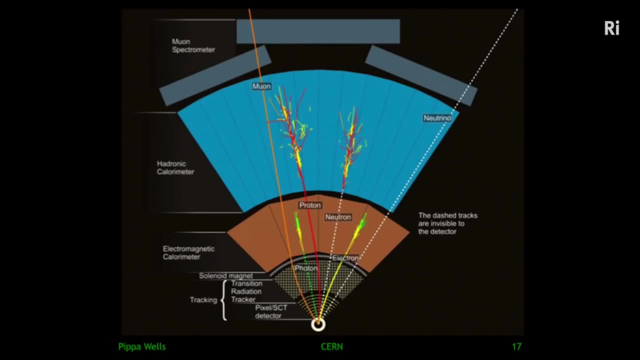 that are coming out. And then there's the last part of the detector which fills those toroidal magnets that you just saw the picture of, And in this sketch it's only showing the first layer of that part of the detector. It would actually reach all the way out. 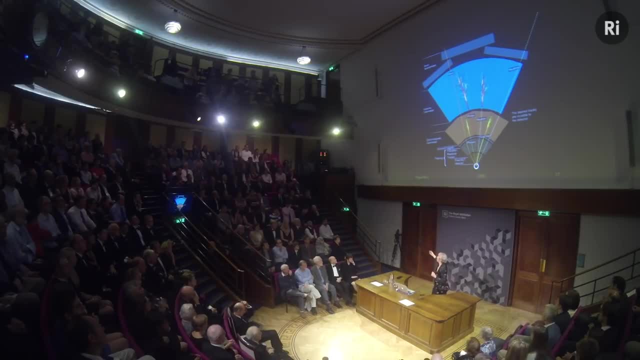 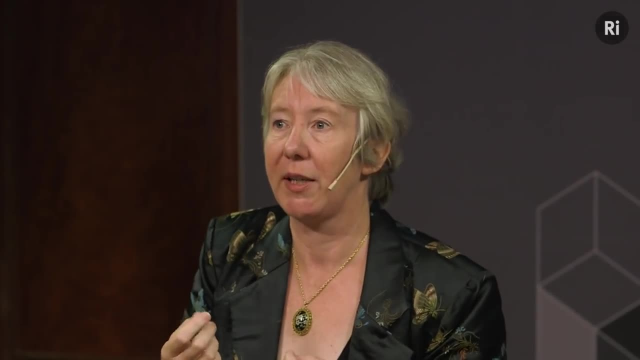 through all the rows of seats. You're all sitting in the part of the detector that measures muons. Now, muons are that heavy partner of the electron And they're sufficiently stable that they can live long enough to fly the whole way through the detector. 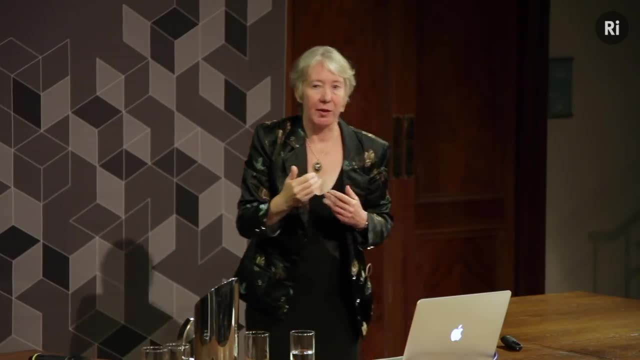 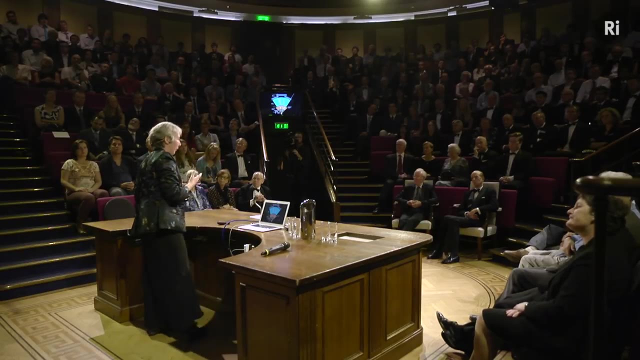 But they only interact weekly So they don't get stopped by the calorimeter. So if we see a particle which makes a track here in my table and then flies all the way out through the audience, that could be a muon. The last particle is the most tricky of all to detect. 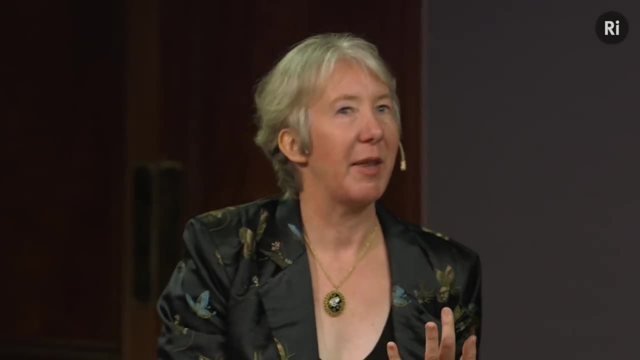 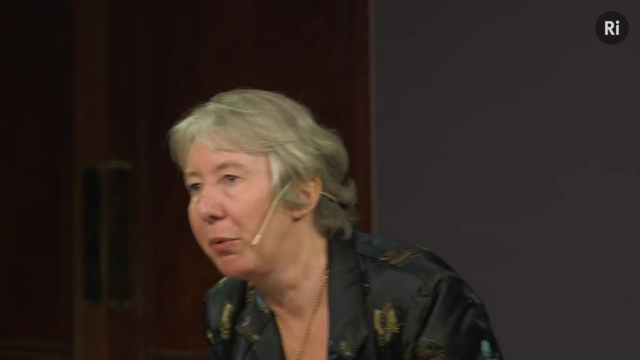 That's the neutrino. It's nearly massless. It doesn't interact with anything, It just escapes from the detector. That's why we have to try and surround the interaction point completely. We need to measure everything that comes out, because then we can add up the energy. 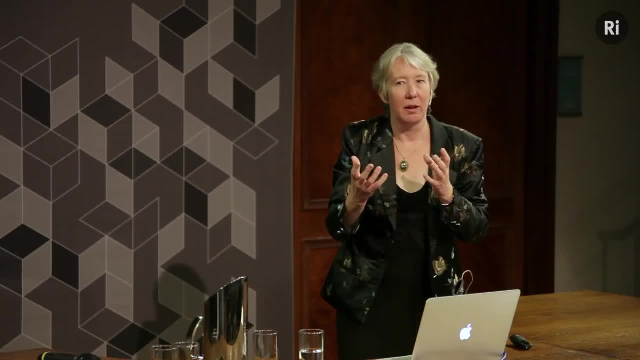 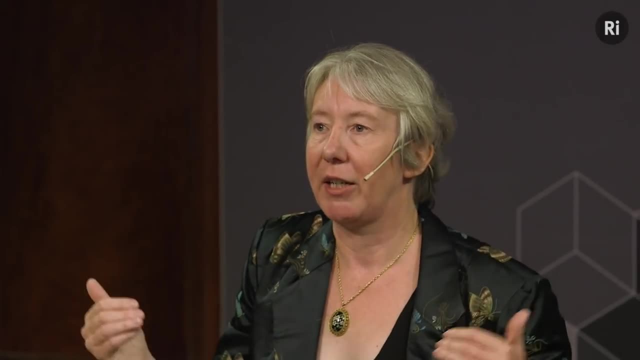 and see if it balances. Is there some missing energy? Is there more energy coming out? There's more energy coming out one side than the other. If there's an energy imbalance in the transverse direction to the beam, that's an indication that an invisible particle 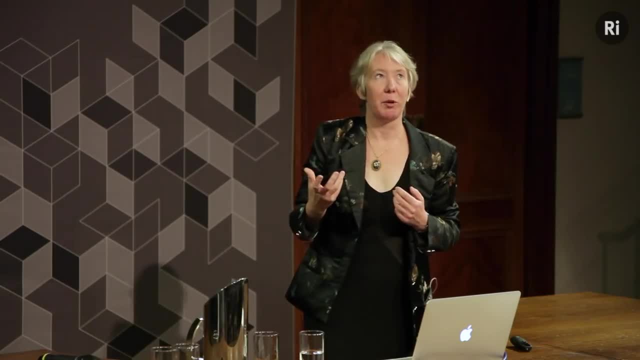 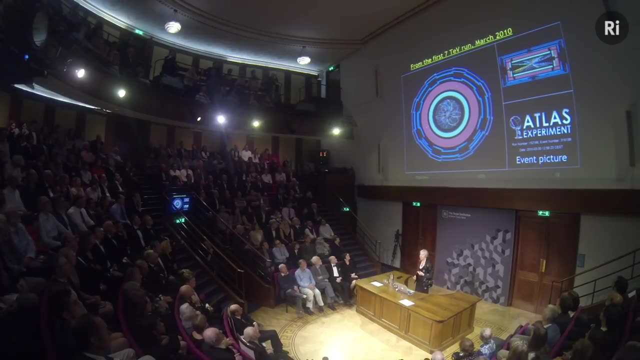 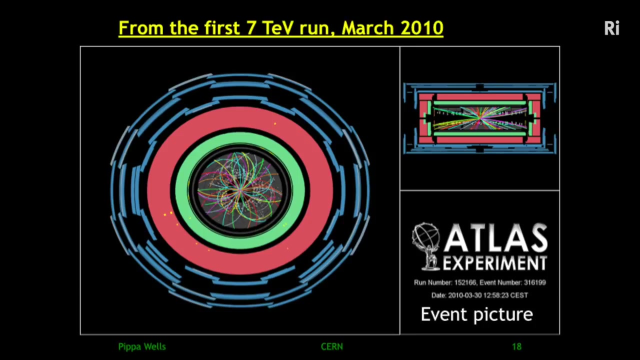 is being created So we can even measure invisible particles. So you're now ready to look at a real event picture. This is one of our 40 million pictures- a second that we've taken- And this was in the very first running when we cranked up the LHC. 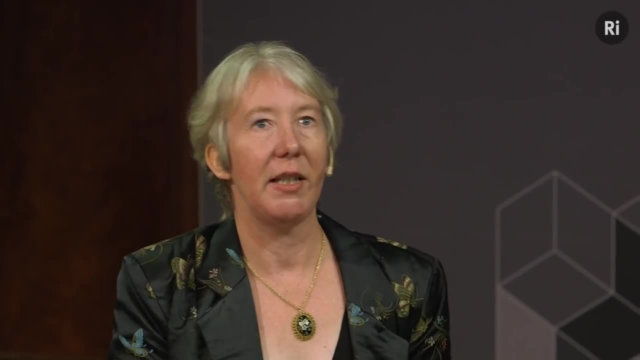 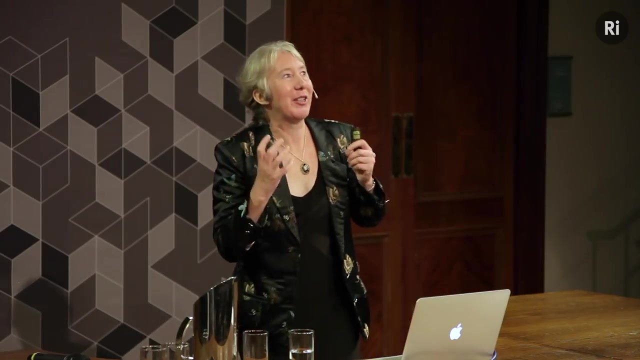 to half of its design energy. So seven TV computers and one collision energy: 7,000 times the energy you need to make a proton. We were so excited We'd got our first collisions In this event. you can see quite a lot of tracks. 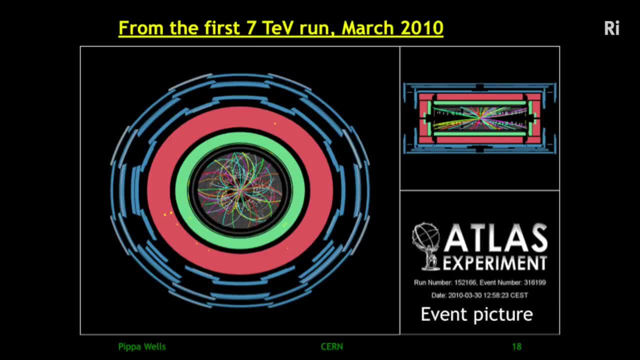 in the central part of the detector. They're all quite bendy, They're all curved, They're actually quite low energy tracks. And then in the calorimeters you can see a few yellow blobs in that red part of the calorimeter. They're the size of the blobs. 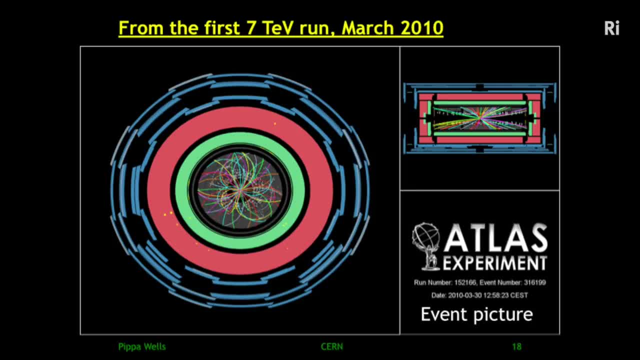 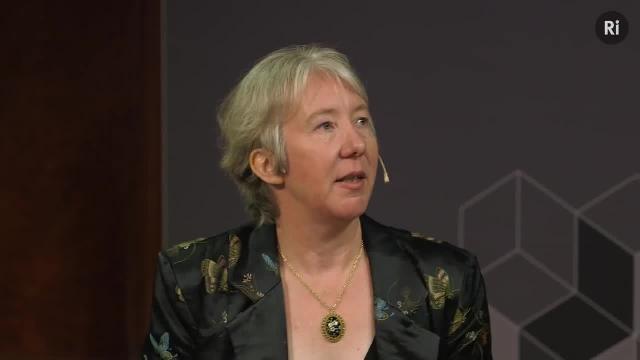 in this event. So it was really exciting We were seeing our first collisions, But it's a fairly ordinary event. The number of events you see in a collider depends on two things. It depends on the energy that you're running at. So here we're running at half design energy. 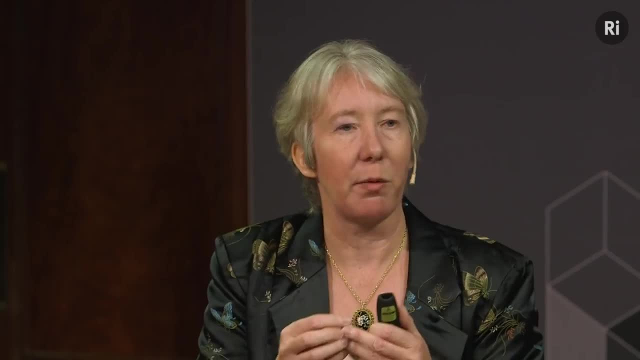 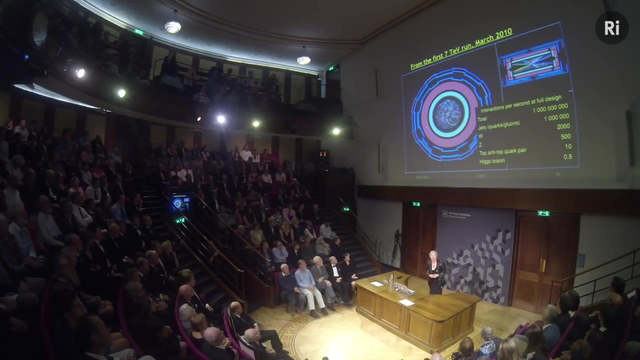 And it depends on the number of actual potential collisions. So that's what we call the luminosity, The rate that collisions are happening in the detector And at full design. energy and luminosity, given that we've got lots of protons, 100 billion protons. 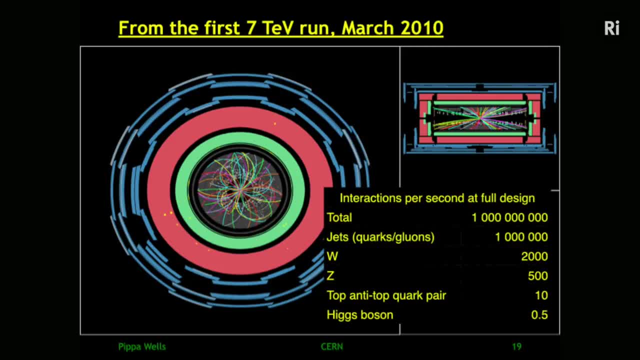 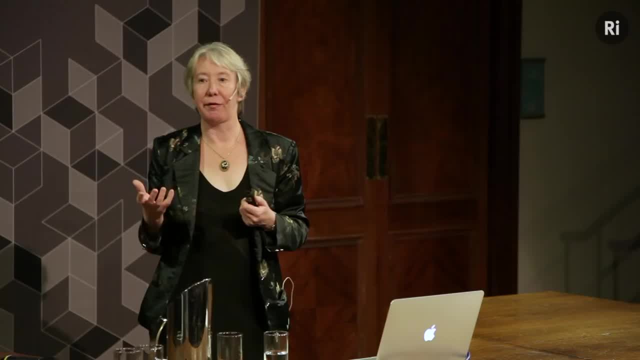 in each bunch And we've got bunches colliding 40 million times a second. You'd actually get a billion of these ordinary events every second. Now we can only record a few hundred events a second, so we've got to pick out the ones. 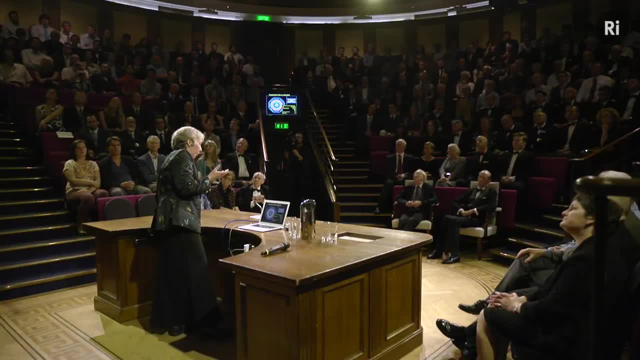 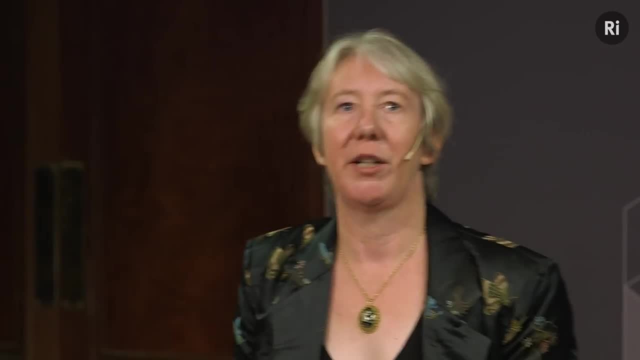 where something more interesting has happened. So, for example, quarks and gluons. what you see in the detector, if there's an energetic quark or gluon, is a sort of spray of particles. We call that a jet- An energetic jet of particles in the detector. 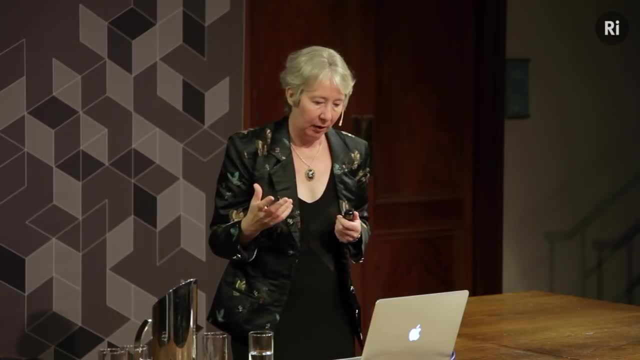 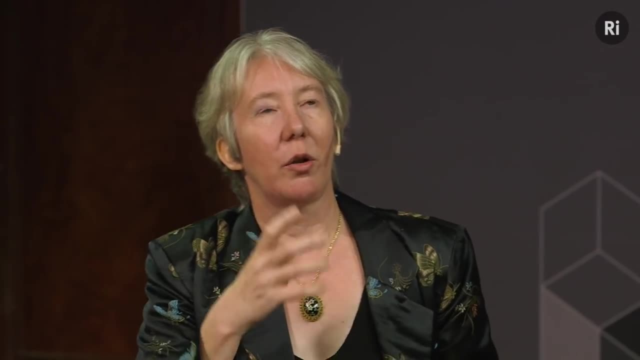 You can already cut the event rate by a factor of a thousand. You're only getting a million. a second It's still far too many, Those W and Z bosons that cause the weak force. you're getting a couple of thousand Ws. 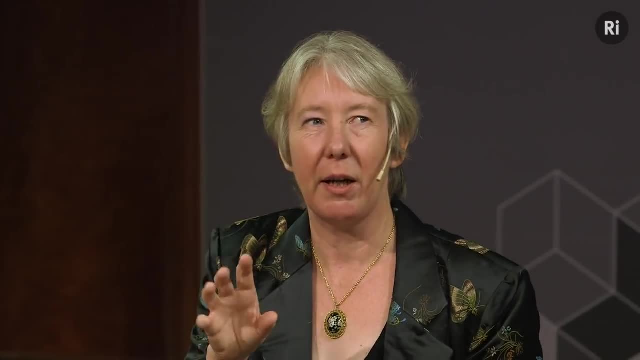 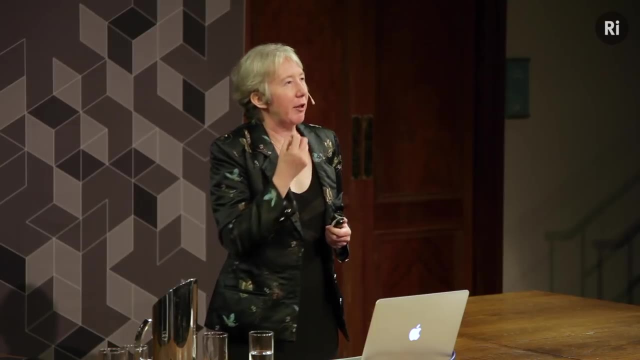 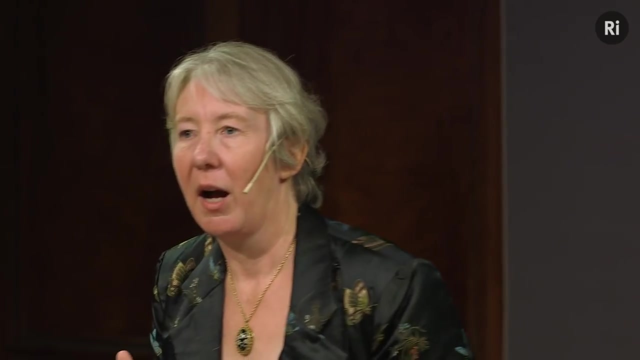 a second and 500 Zs, So that's starting to be a much rarer process than these billions of ordinary events. If you create a top quark-antiquark pair- a top quark and a top antiquark- you only get ten of those a second. 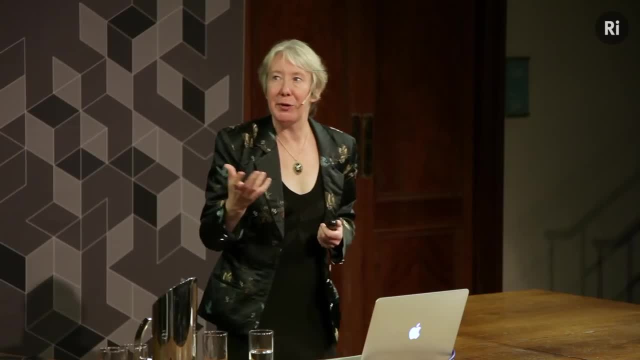 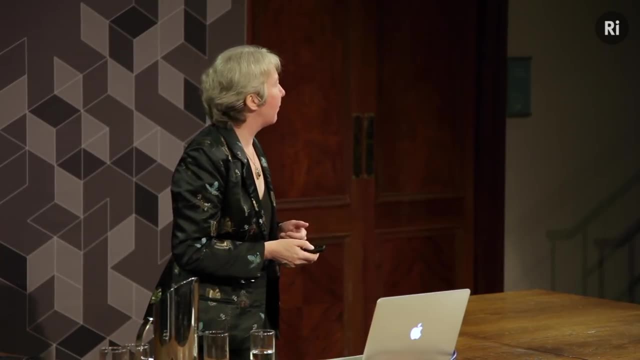 And then this elusive Higgs boson, our first mystery. you only get one every two seconds. It's an incredibly rare process compared to those ordinary events. So can we see these rare processes Just a month later, by April 2010,? 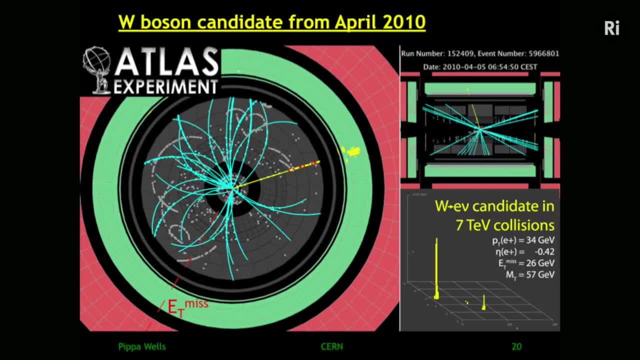 we started getting some events like this. This is an event that looks like a W boson decay. This is why we say candidate. It looks like a good example of a W boson decay. The W boson's quite heavy 80 GV particle. 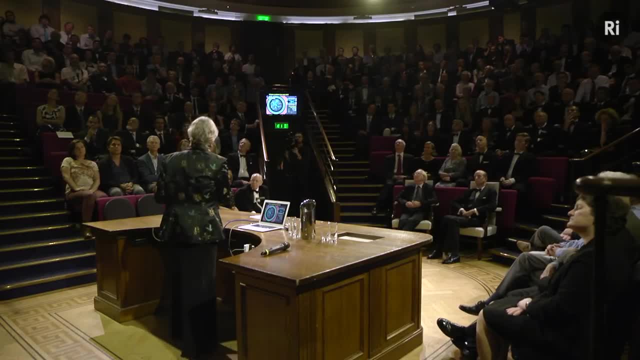 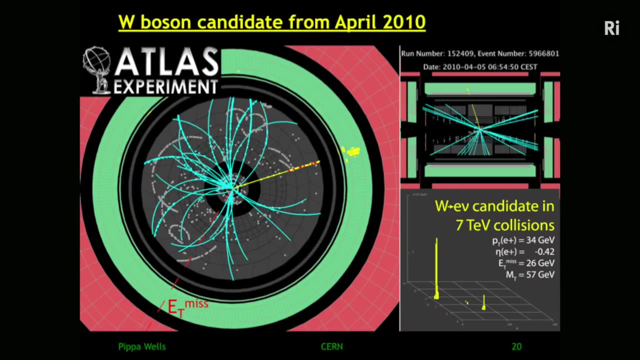 and it's charged, So it can decay to a charged lepton and one of those neutrinos- In this case it's an electron candidate. There's a very straight track pointing to a large deposit of energy in the calorimeter, And then the other tracks. 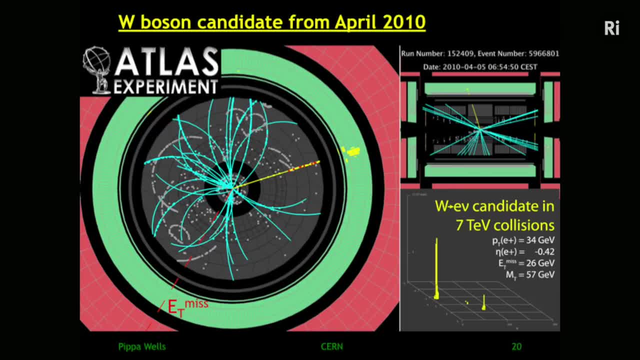 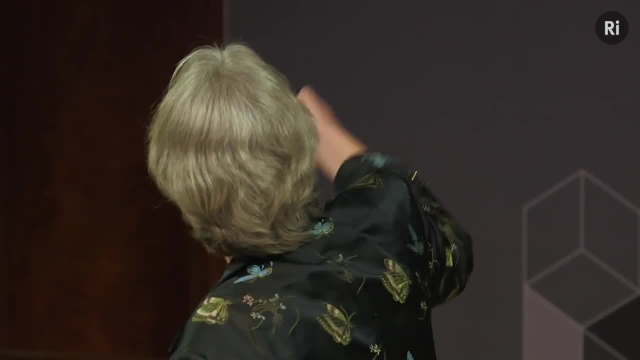 in this event, are quite curly. They're quite low energy tracks. So if you add up all the rest and balance, there's a significant amount of missing energy marked by this red dotted line. So that's missing energy. transverse to the beam direction. 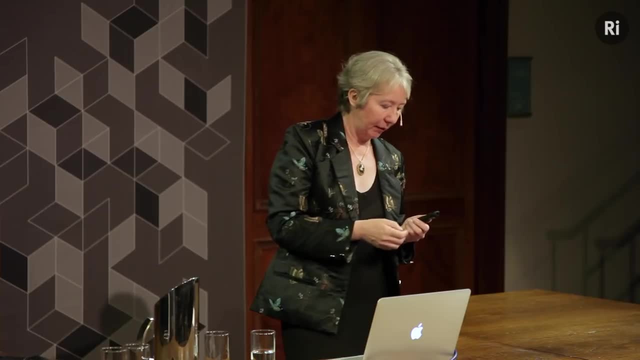 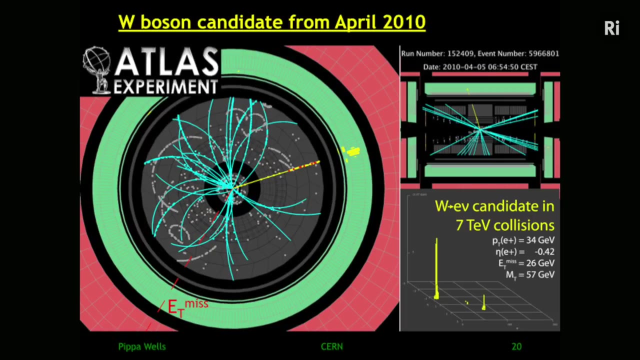 So it's probably a neutrino that's gone there. So this is a good candidate for a W boson event. In this view the beam's going down the centre. This is the side view of the detector, And then in the third panel. 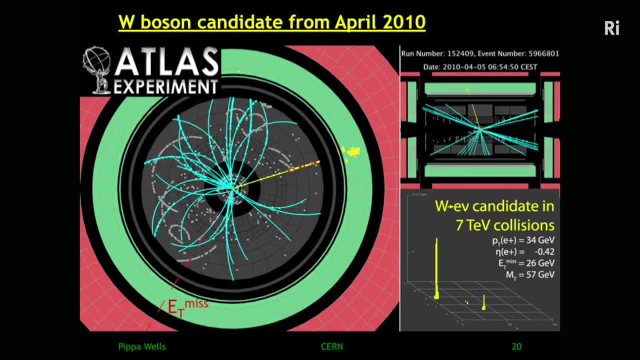 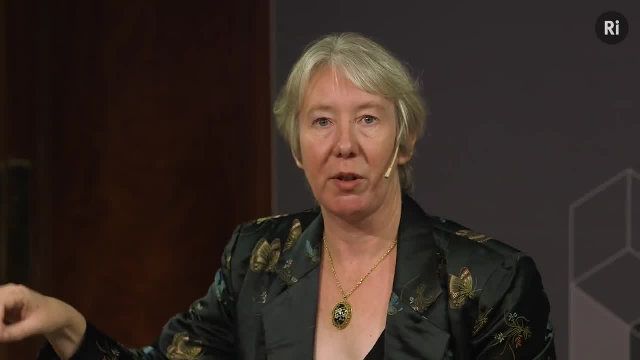 the bottom right panel. that's as if you'd unwrapped the calorimeter just to kind of make a map of where it's going to go. So that's why you see this one really tall tower. that's the electron. one other small deposit: 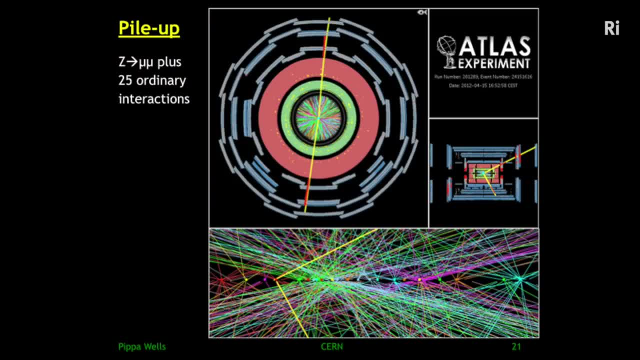 that doesn't balance it. We can also find events that look like Z boson decays, the other weak force particle. Now the Z boson is neutral, but we can pick out the events where it decays to an electron and a positron. 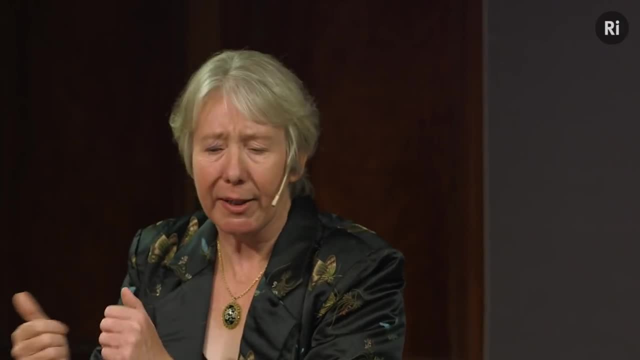 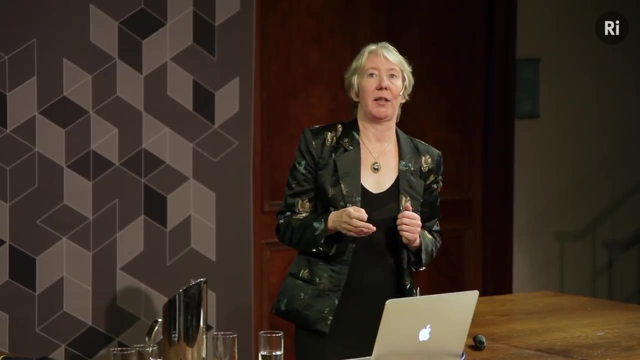 or to a muon-antimuon pair, a mu plus, mu minus pair. This event is from much later in the running, So as well as the two muon tracks, those are the ones going out through the audience. there are lots and lots. 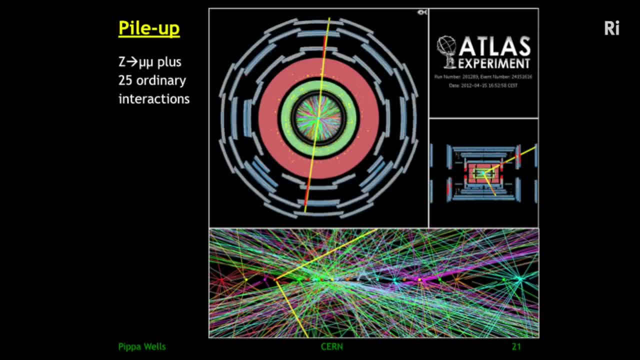 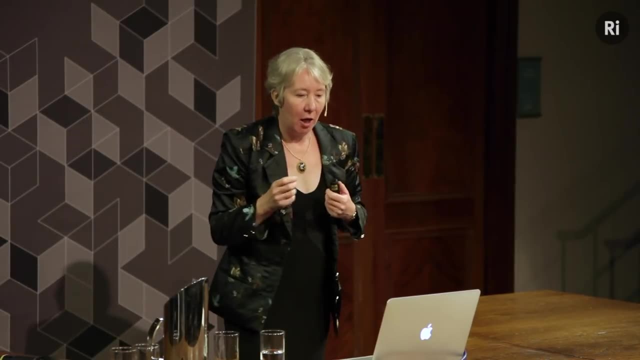 of other tracks. in the event, In this bottom panel this is a zoom-in- well inside the first detecting elements of the detector. That length of that panel is a few centimetres along the beamline where this one bunch of protons, with 100 billion protons in each bunch. 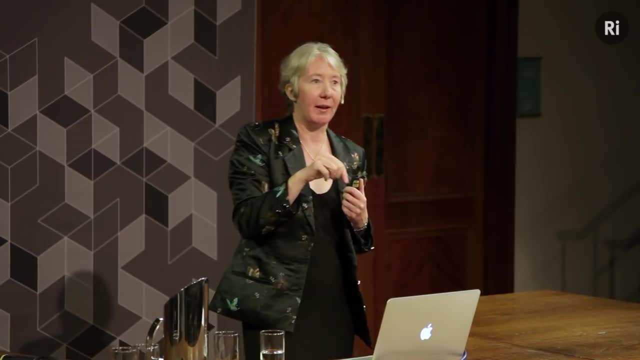 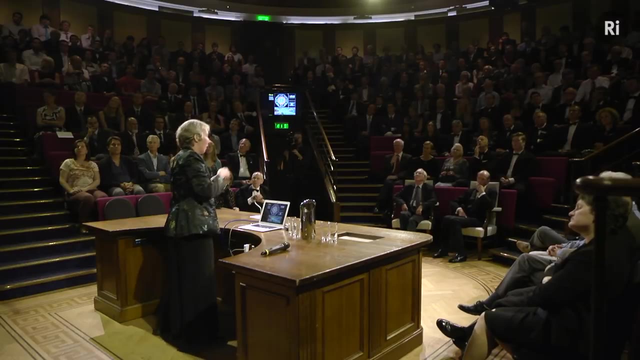 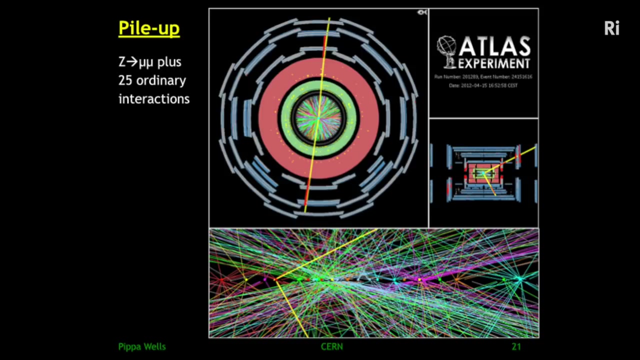 has collided. If we look at the yellow track, we can actually point back and pick out that there are 25 different events. There are 24 of those ordinary events and then both of the muon tracks. the yellow tracks project back to the same point. 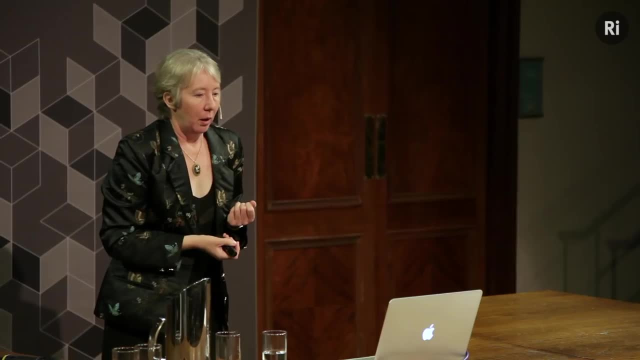 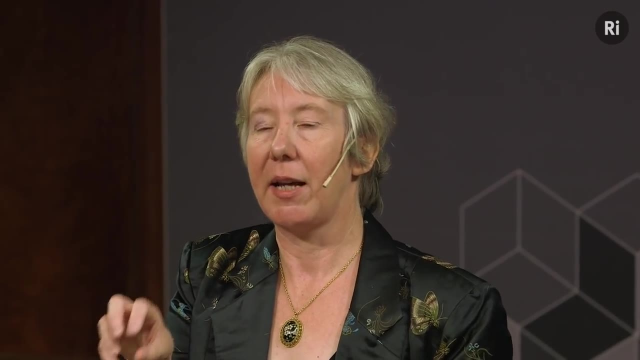 So these two very energetic muons have come from the same interaction. Now, if we know the direction and the energy of those two muons, we can work out the energy of the thing that decayed into them. That might be a Z boson. 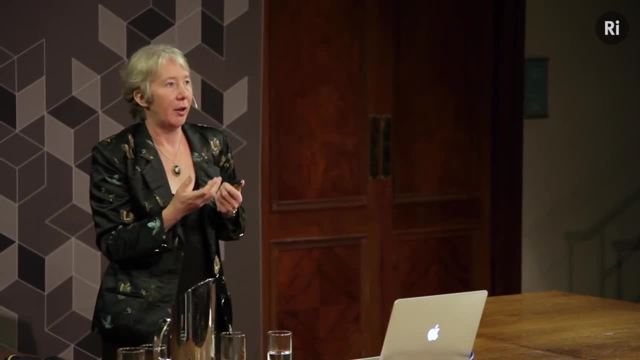 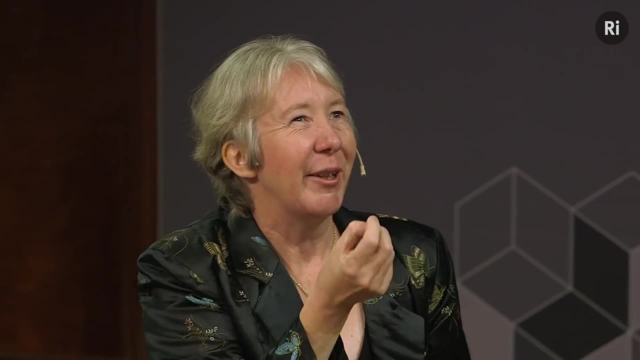 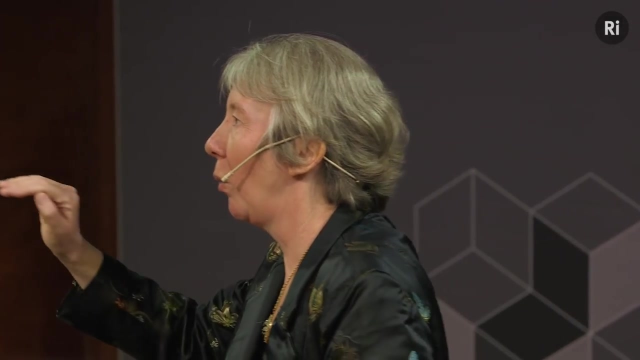 in this case, But lots of different processes can give two muons in the final state. But in each case, by measuring the two muons and reconstructing the mass of that object that decayed or that quantum fluctuation that happened, you can gradually try to work out. 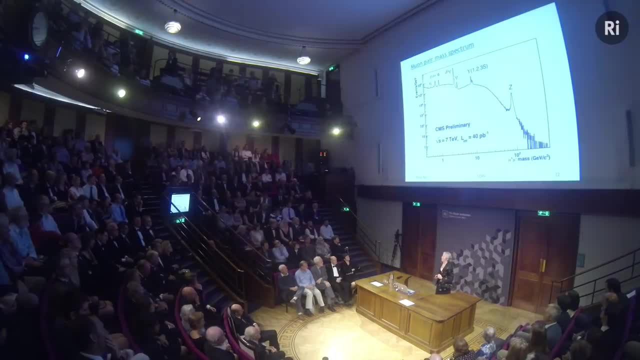 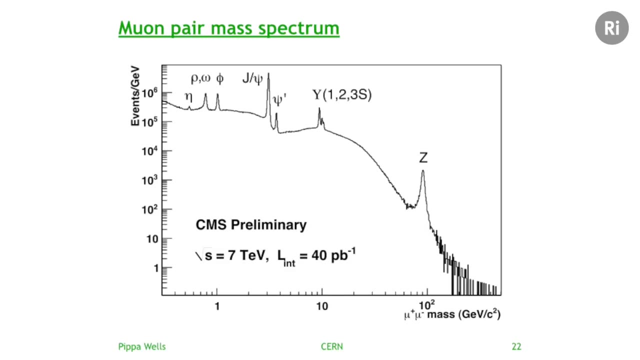 what's going on in all these different kinds of events that decay to mu plus, mu minus. So this is what happens with two high-energy muons. You can see a fairly smooth distribution with peaks. So this peak, for example, that lines up when you've just got 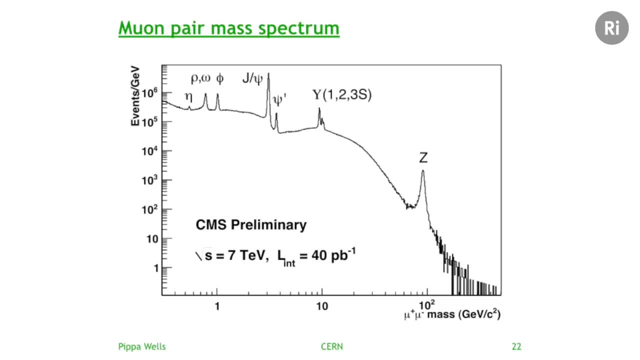 enough energy to make a charm-anti-charm pair. The next peak is if you can make a bottom quark and an anti-bottom quark, And here at 90 GV. that's when you've got enough energy to make Z bosons. 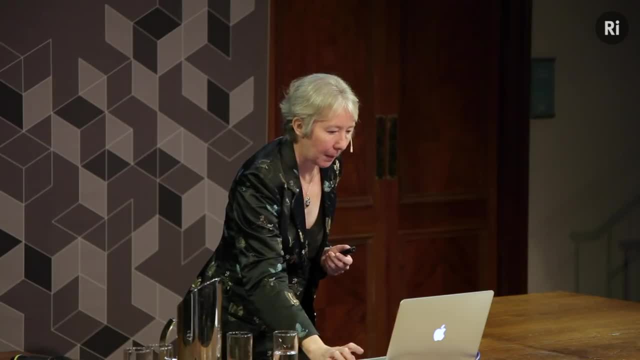 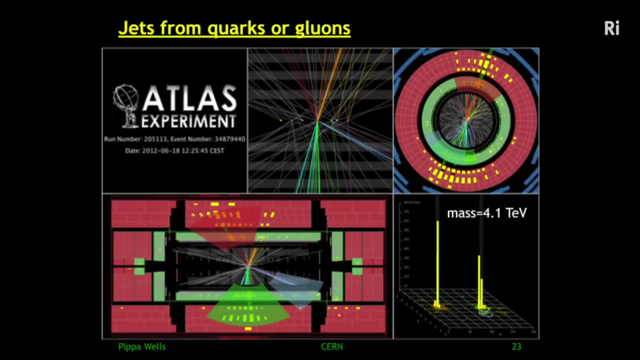 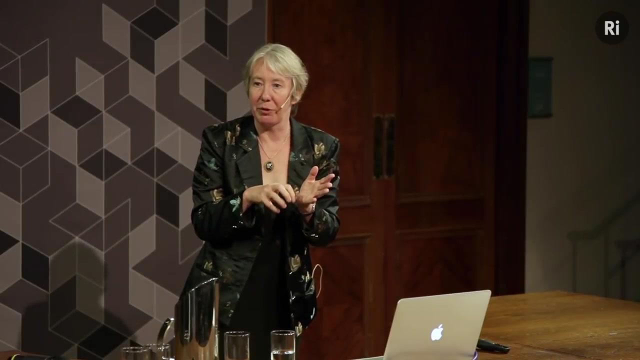 It's like several orders of magnitude to make it. Quarks and gluons in the detector make a jet of particles, a spray of particles, And you can do the same thing. You can measure the energy in the direction of those jets and try and work out. 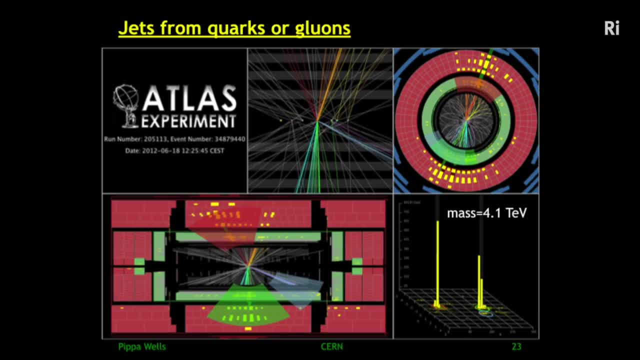 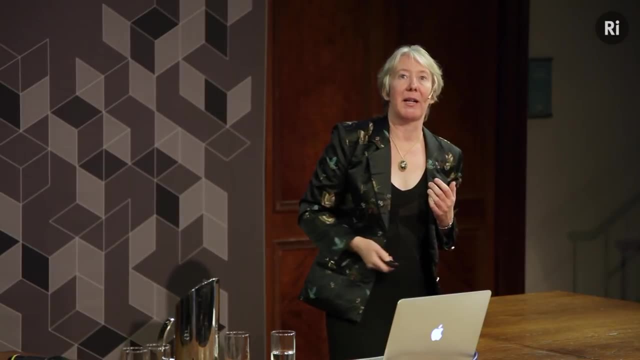 what mass object decayed. But in this case you can go incredibly high in energy. This event display here. this picture shows two jets of the mass of the proton, So half of the collision energy has gone into these two jets. So this is a very rare event. 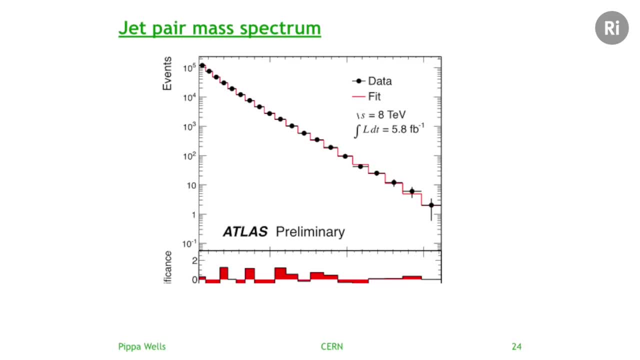 If we plot the mass- not of muon pairs this time, but of events with two jets, it's falling off quite smoothly. Now in this plot, the black points are the number of events we've seen in data. The red line shows what we predict. 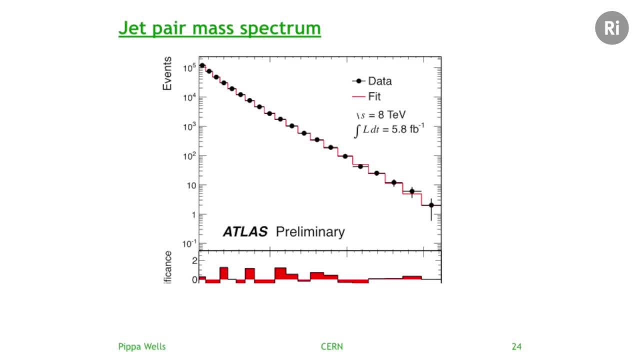 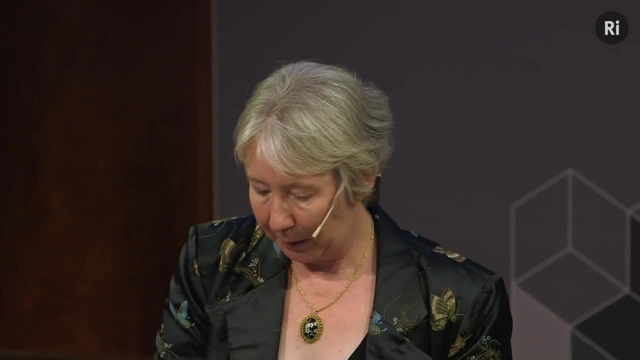 in each bin from just a fit through those data points, a smooth fit In this mass spectrum. So what about the Higgs boson? If we want to look for Higgs bosons, one of the ways they can decay is to two photons in the final state. 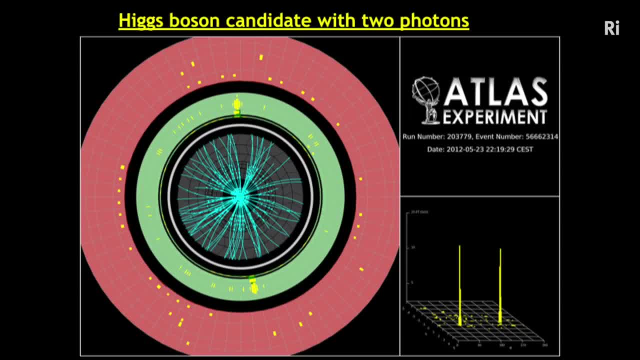 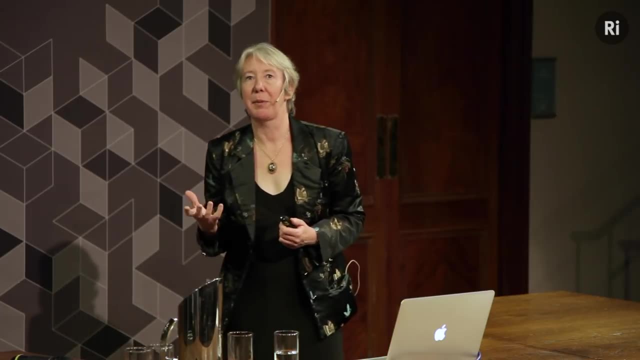 So in this event display the photons are neutral particles. There's no track particularly pointing to these two large energy posits. There's one very soft track, maybe to the lower one, but it doesn't actually line up in the other view. So this is a candidate for a Higgs boson event. 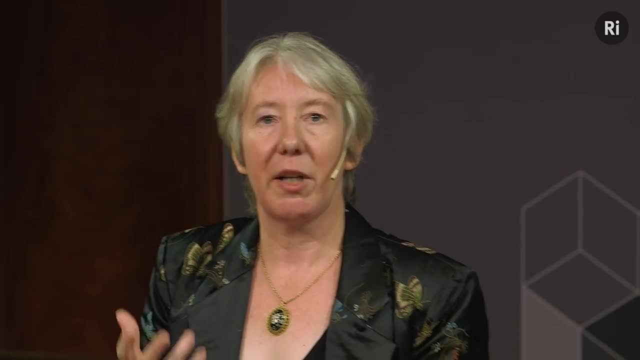 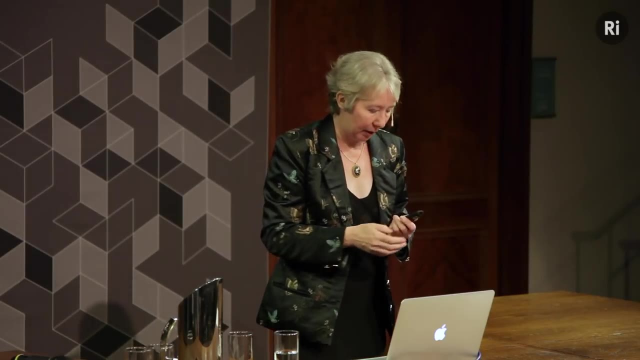 This is the kind of event where there's been a process that decays to two photons, But again, there are lots of processes that can do that. So we're going to have to do the same thing. We're going to have to plot the mass. 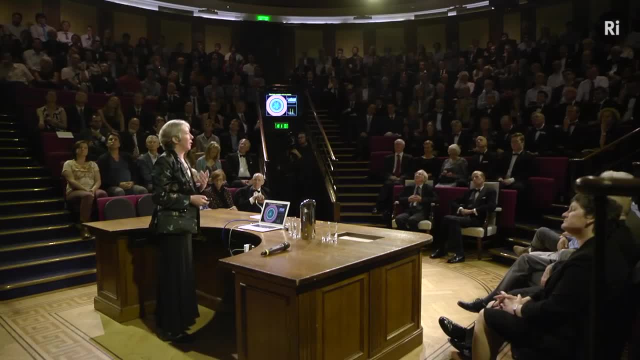 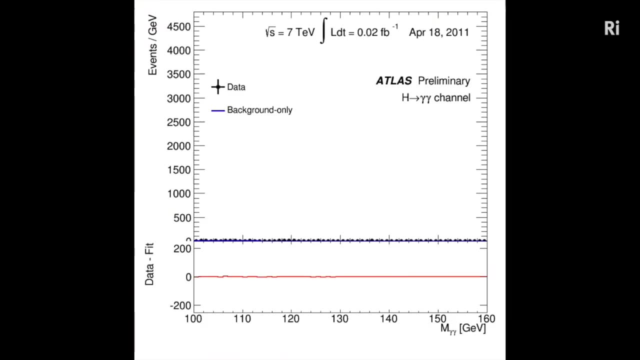 and see if a bump starts to appear By the end of 2011,. we were starting to see some kind of hint, some tantalising hint. Was there a Higgs boson signal emerging? And this is what happened. as we added up the 2011. 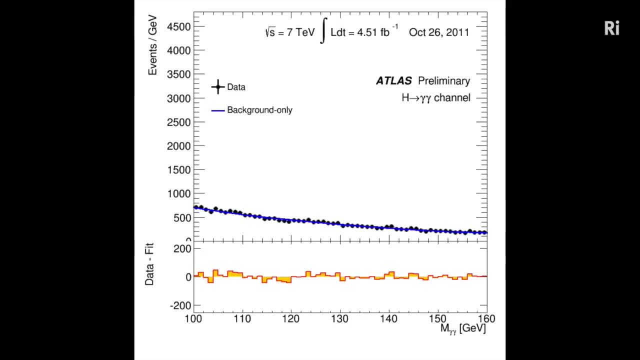 and 2012 data. So by the end of 2011,- you can see the date clicking up in the corner- There was a hint of a bump that we could sort of pick out, And by the middle of 2012,, there was really quite a bulge. 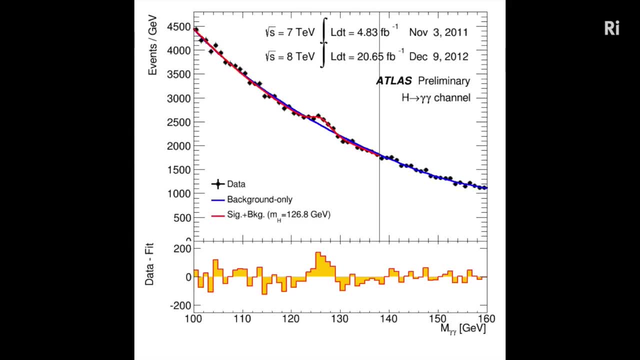 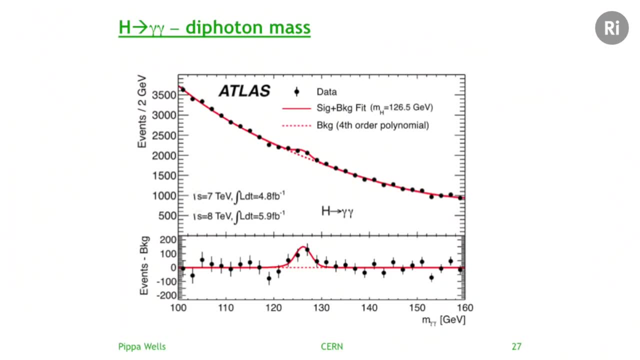 appearing on top of that smooth blue background curve, And the bump had a mass of about 125 GV. This snapshot is what it looked like on the 4th of July 2012,, when the ATLAS and CMS detectors had a joint seminar. 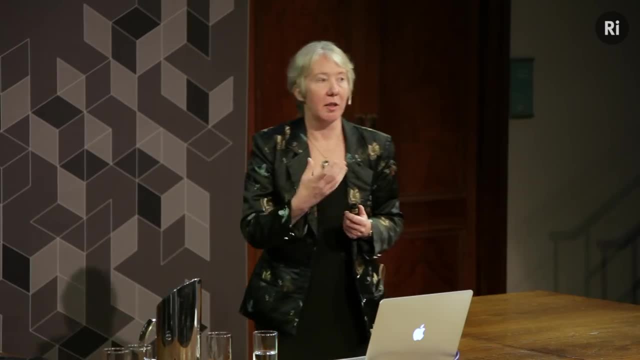 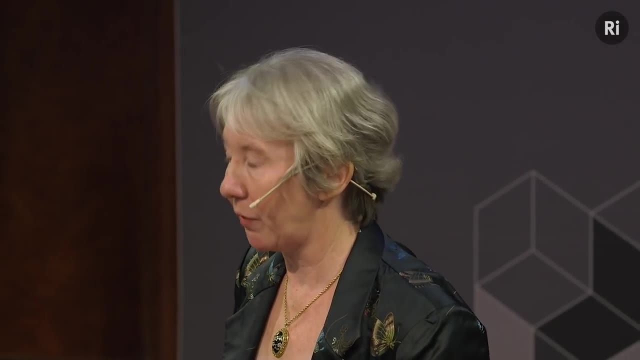 to say what they'd found. So in just the two photon events there's really quite a strong bump there saying it might be a sign of a Higgs boson being produced. But the Higgs boson can decay other ways. It might decay to two Z bosons. 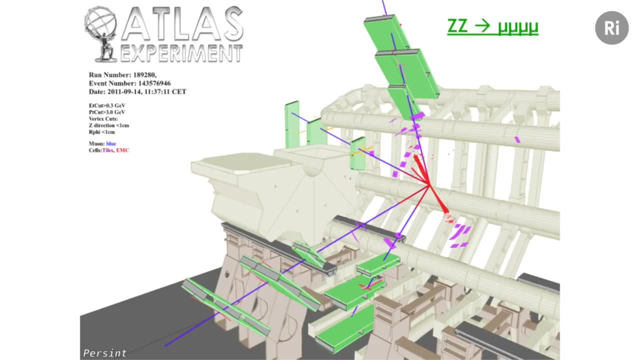 each of which then in turn give two muons. So this is an event with four muons. but you can do the same thing. You measure the muons, you work out the mass of the object which decayed. Now this is a lot rarer process. 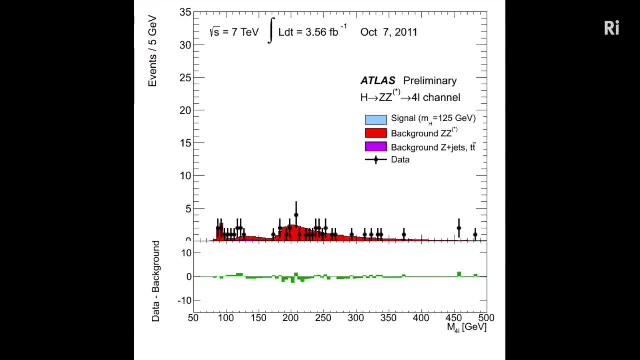 But all the same, you can accumulate the data And the background processes. this time they're not smooth. It's actually got a shape. We actually have to use the theory to predict the red curve. The red curve is what you expect to see from theory. 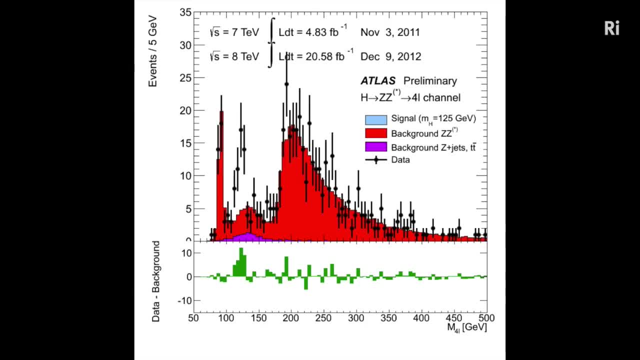 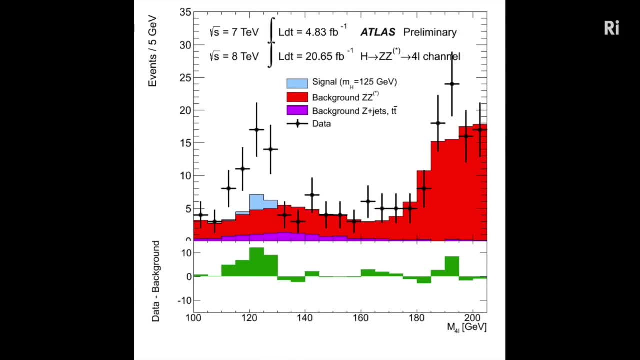 But there's this other bulge appearing in between the two peaks. There's another excess of events in these ZZ events. So this is again at around 50 and it could be consistent with making a Higgs boson. So again, there's the snapshot. 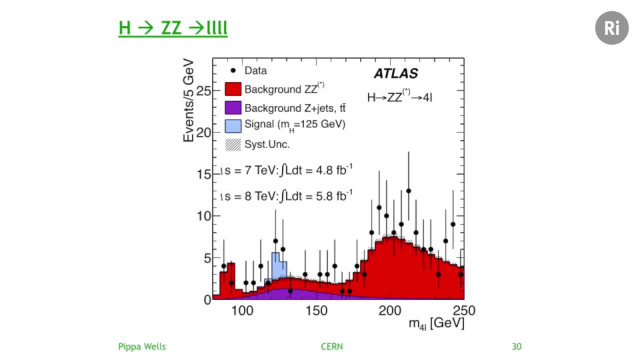 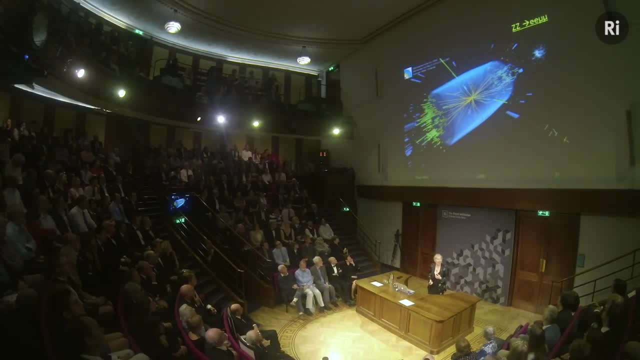 from July 2012 when we had this big seminar- I work on ATLAS. I knew what we were going to show, but I didn't know what the colleagues in CMS might have found. They also had spectacular event displays with two Z bosons decaying. 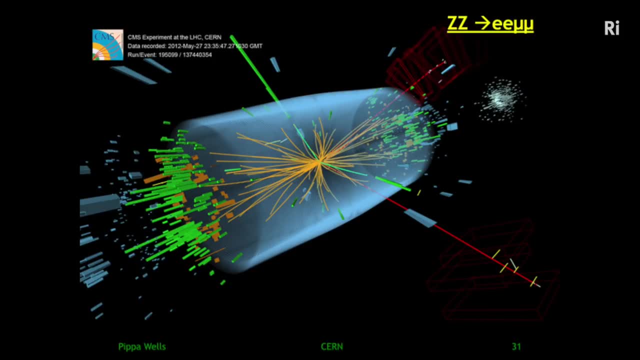 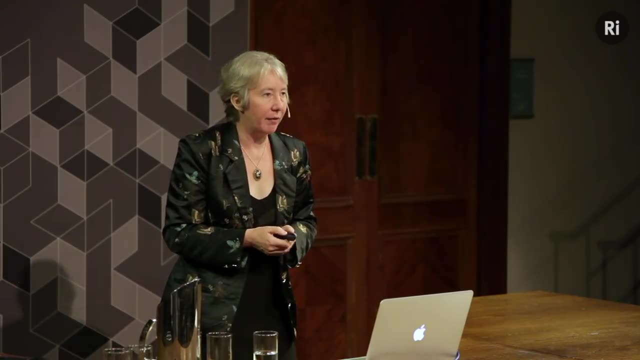 In this case it's an event with two Z bosons, One's decaying to two electrons and one's decaying to two muons. They were spotting the mass, They were looking for extra events And the CMS speaker went first. There was a big seminar at CERN. 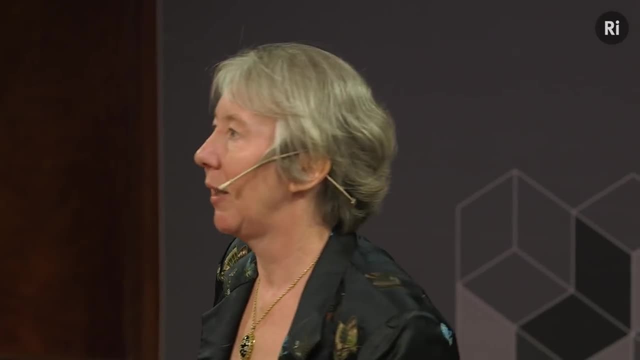 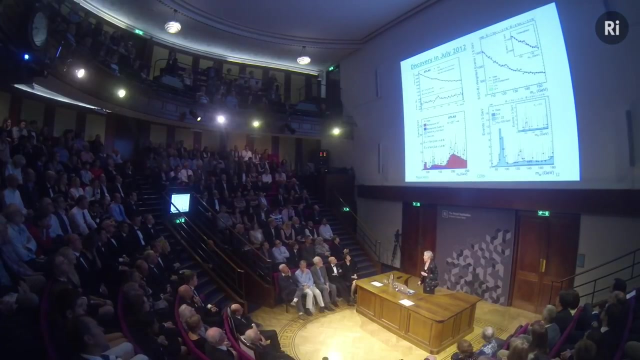 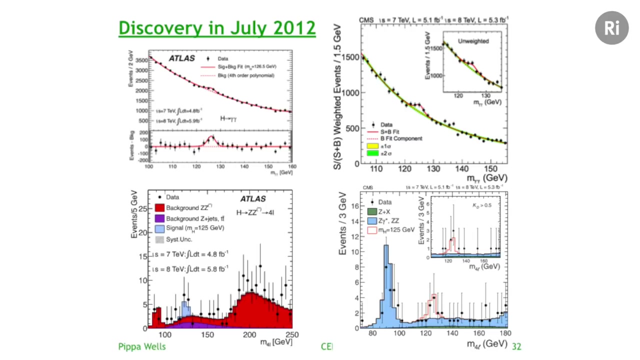 It coincided with the big summer meeting in Melbourne. People were queuing overnight. People stayed up overnight to get a seat in the auditorium. CMS also had a significant signal. They had enough data to be able to announce a discovery. They saw a bump in the two photon spectrum. 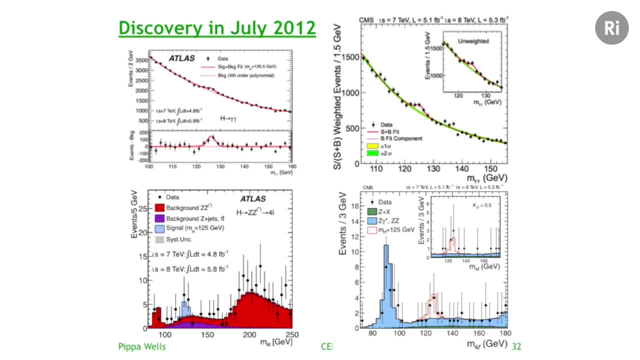 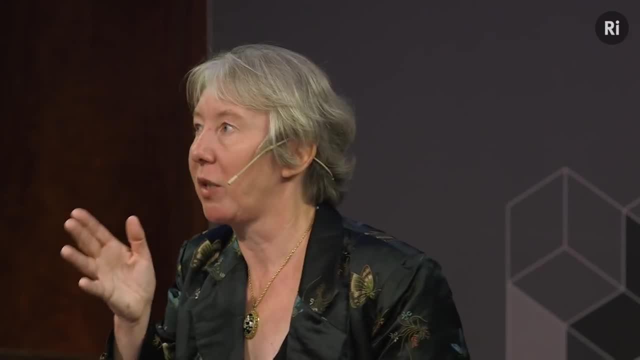 They saw the same characteristic excess of events in the four-lepton mass spectrum. So not only were both experiments announcing a discovery, they both saw the particle at the same mass. So we were sure we'd found a new particle, a new boson. 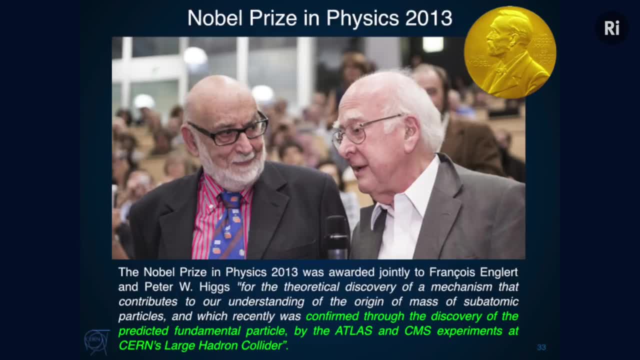 And a year later, we were delighted when two of the theorists that had predicted the mechanism, Francois Englert and Peter Higgs, were awarded the Nobel Prize. Now, this photo is actually from that July seminar, July 2012.. And this is a photo. 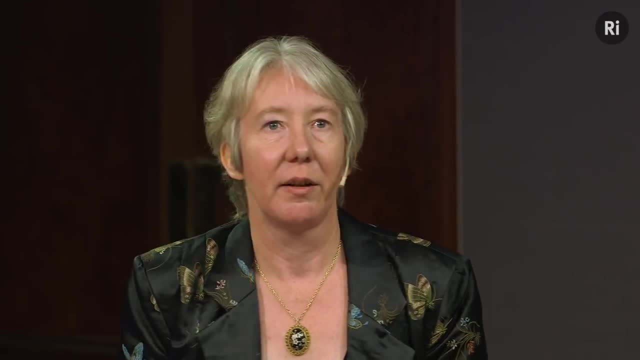 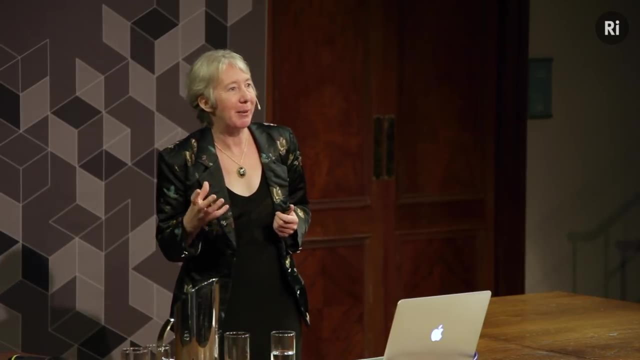 of a large Hadron Collider, And the other thing we were pleased about was, of course, they had done the work to elaborate the theory. but the Nobel Prize citation actually measured the achievements of the ATLAS and CMS experiments in the Large Hadron Collider. 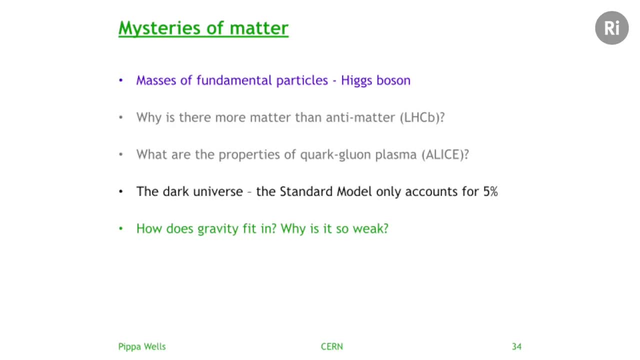 But it's certainly not job done. There are still some mysteries to solve. I'm just going to kind of list them and then we'll go through them in a bit more detail. So the first question is: the masses of the fundamental particles. The masses of the fundamental particles. 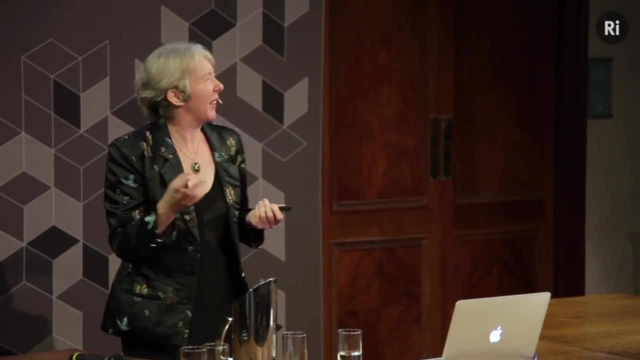 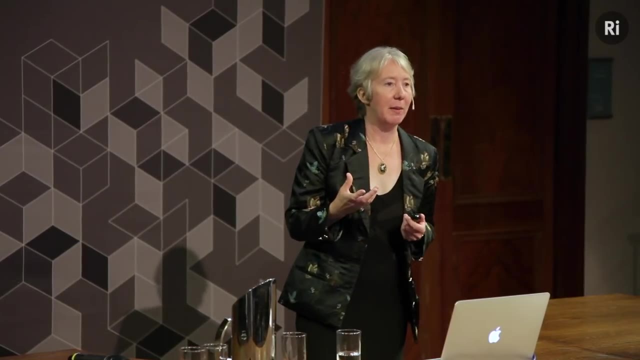 We understand. there's this mechanism, there's a field, there's a boson, but the actual details still leave some things unexplained. So we've got to understand the masses of the fundamental particles better. Then there's the question of why is there more matter? 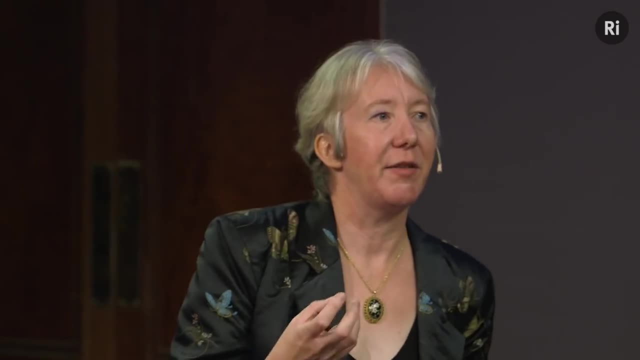 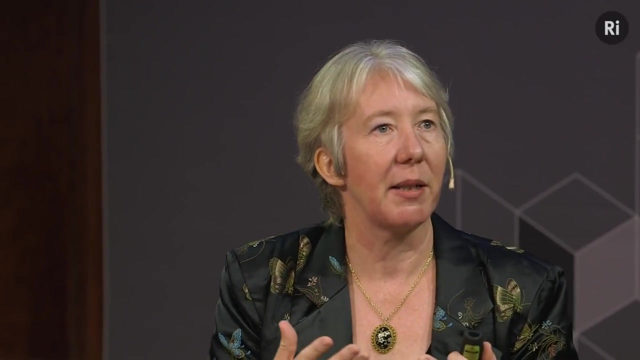 than antimatter in the universe. This is really the speciality of the LHCb experiment. At the Big Bang, there should have been equal amounts of matter and antimatter created, which is good. We're here. It's a good thing. But we don't really understand why. Also, in the early phase of the universe, there was a time when the universe was so dense that the gluons and the quarks, they weren't trapped in nucleons, They were actually moving around freely. That's called quark-gluon plasma And that mysterious state. that's the speciality of the ALIS experiment. They actually take advantage of the fact that if you collide lead nuclei with 208 protons and neutrons in each lead nucleon. 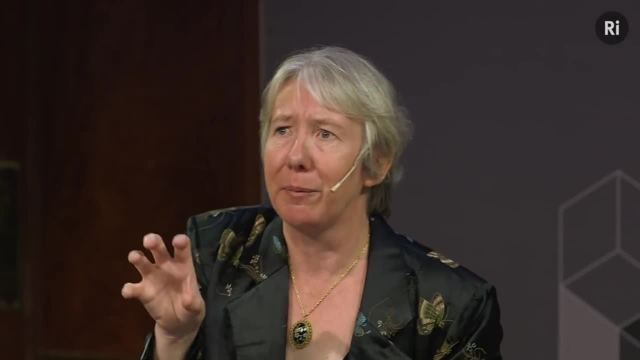 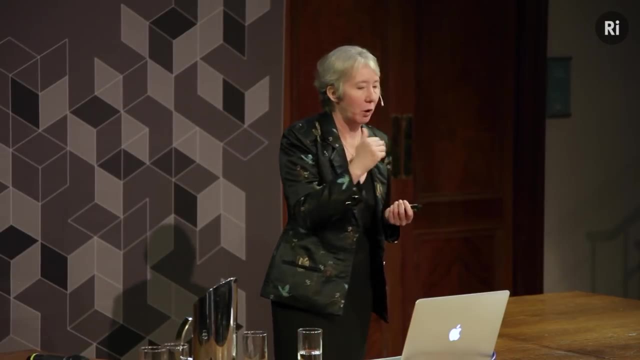 you can create a little droplet of quark-gluon plasma. It decays very quickly. You don't see the plasma itself. But again, by measuring the decay products you can try to work out what's in the plasma. And then there's my favourite mystery. 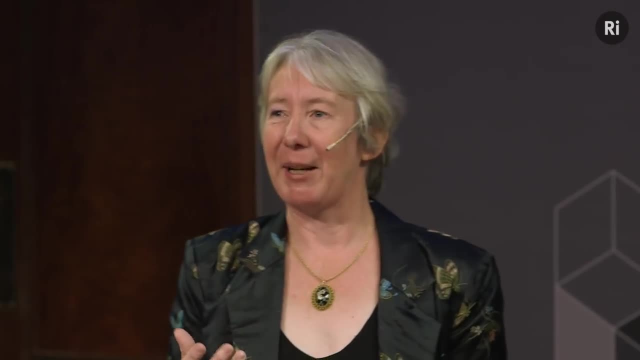 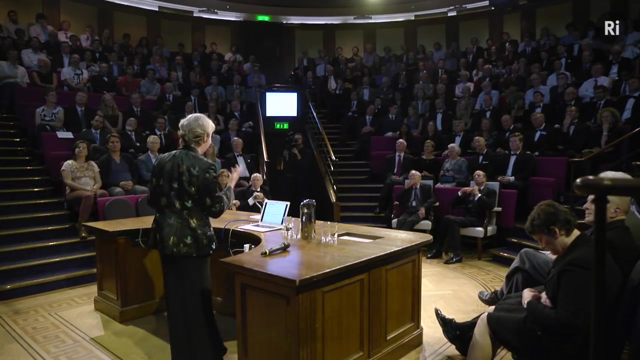 The Standard Model works beautifully, and it explains 5% of the universe, which means we've got 95% still to go. So that's great. We've got lots to do. And the last thing of all, then, is gravity. How does gravity fit in? 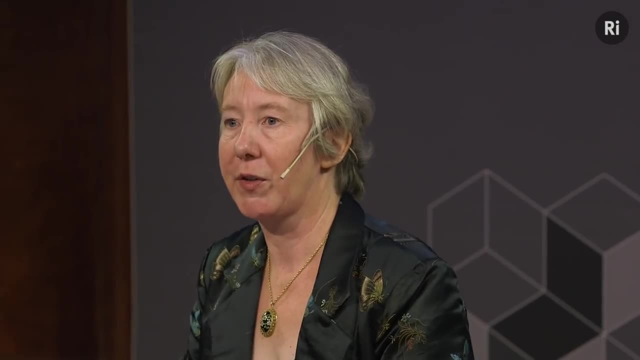 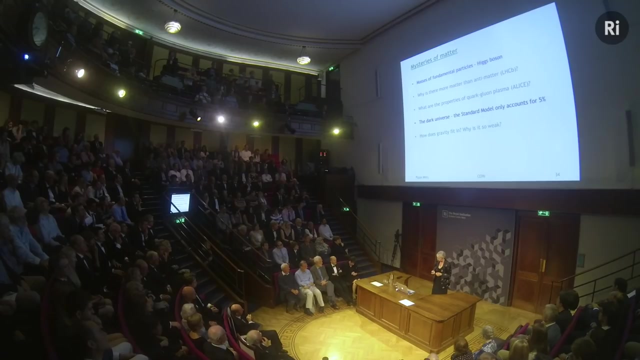 The Standard Model explains the three forces, The strong force, electromagnetism and the weak force, But it has nothing to say about gravity. Can we get a model where we can fit gravity in? So we have a plan. This is the plan. 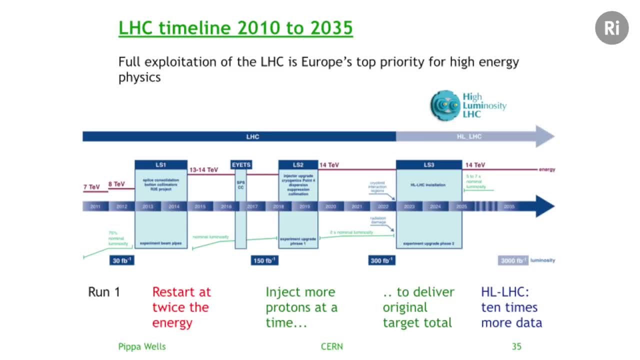 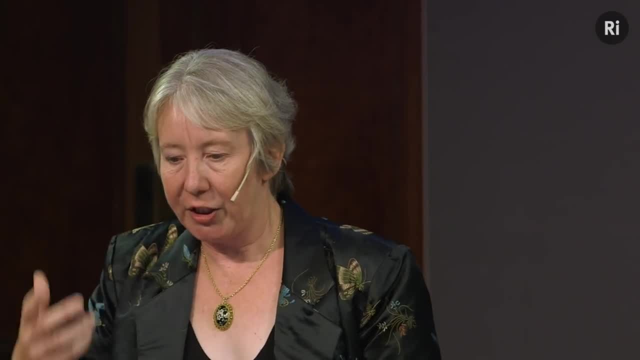 And this is one of the things I've been working on the last few years. How much data do you need to fully exploit the LHC? And the strategy for particle physics in Europe is a kind of policy document that gets updated every few years. 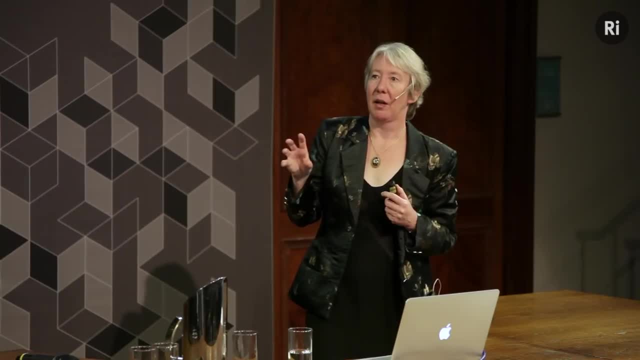 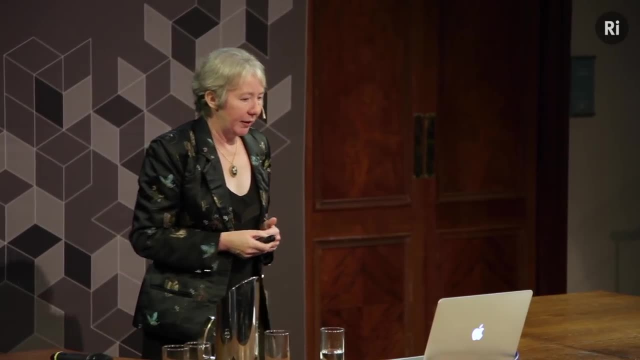 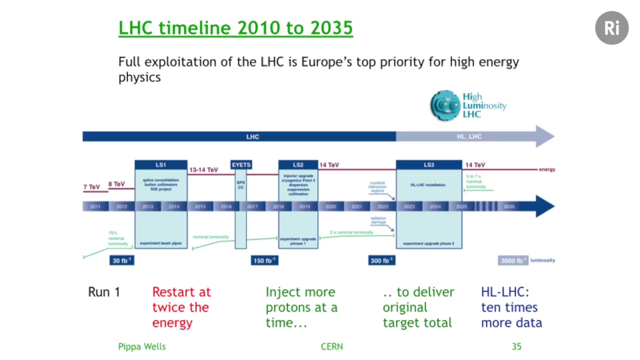 And this new plan was approved in the last policy update And it's Europe's top priority for high energy physics. So we're in the middle of this first long shutdown, LS1.. Long shutdown 1.. Run 1 was very successful. 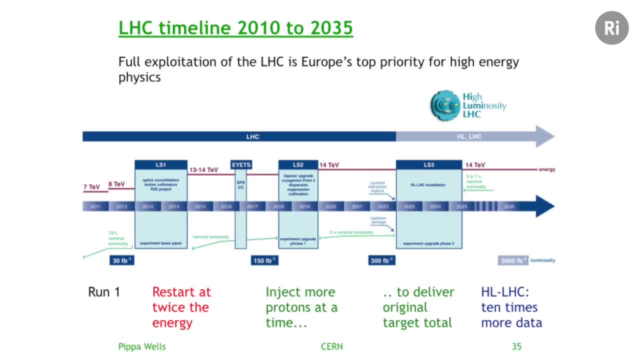 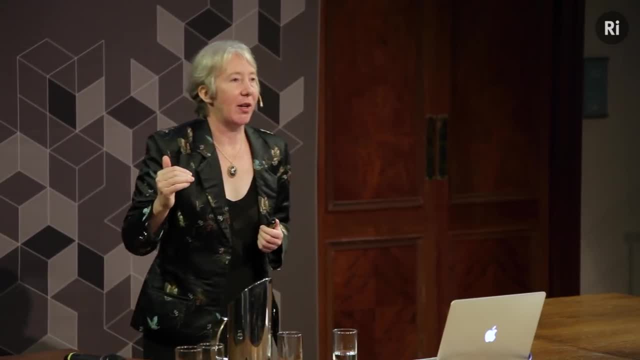 but only about half the design energy. So we're repairing the magnet connections now in this long shutdown. When we restart next year we'll be running at twice the energy, So that's going to give us a lot more sensitivity to try and explore new processes. 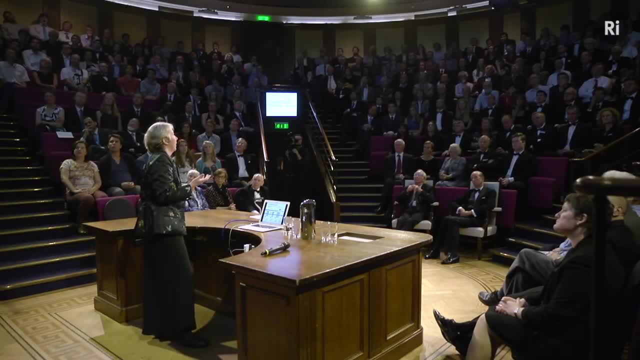 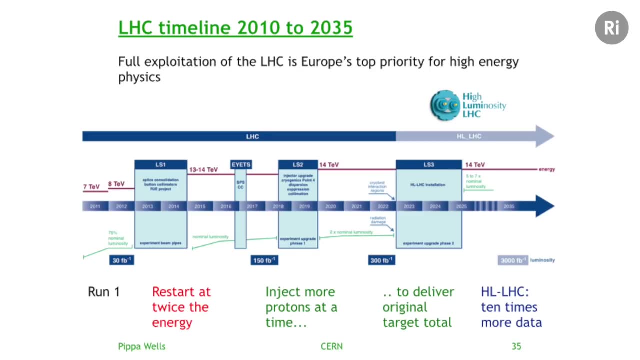 We will run for a few years and then we'll have another long shutdown, LS2, where there the focus is going to be on improving the accelerators that bring the beams into the LHC, So the other accelerators at CERN. 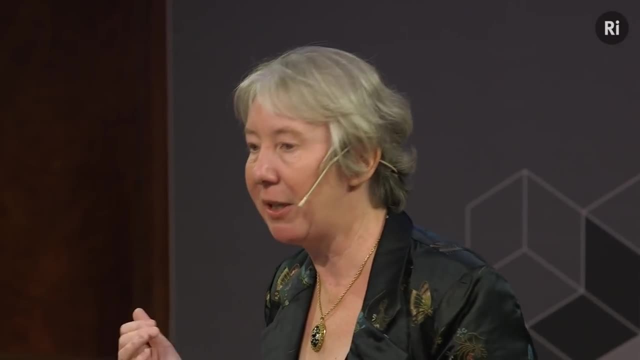 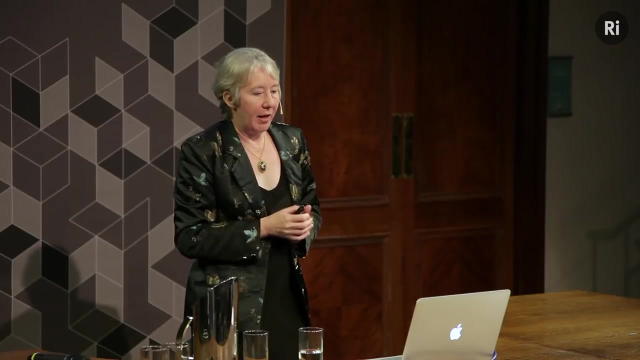 Then we can inject more protons per bunch, even more than this 100 billion per bunch, And we can maybe get up to twice the number of collisions going on. And then we'll achieve, with a few more years, data taken with the original target data set. 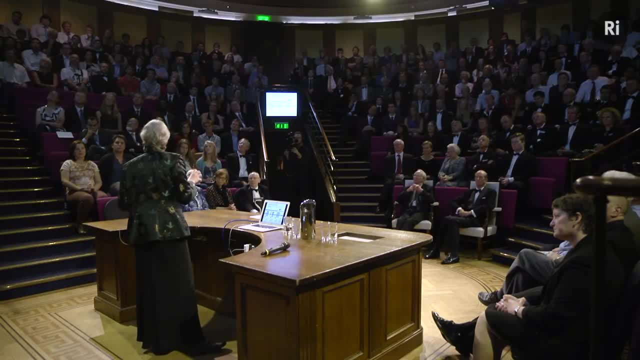 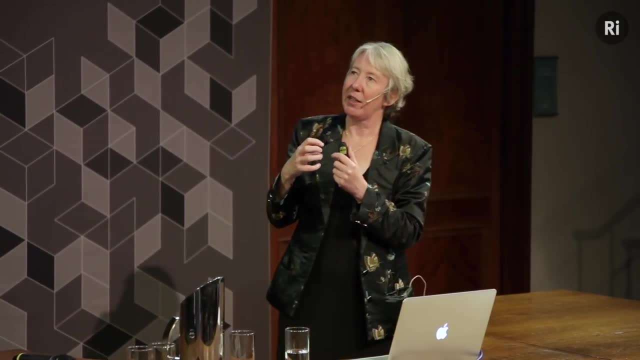 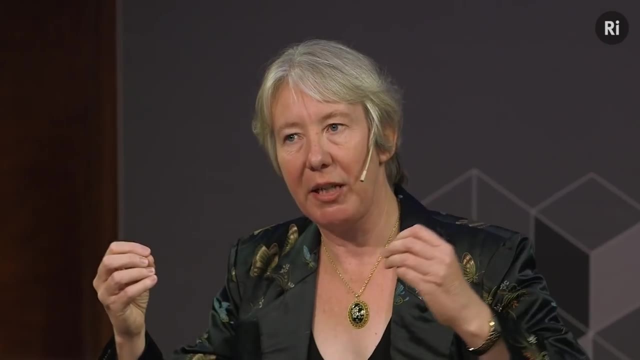 of the LHC. But we know now, we need more than that if we're really going to measure all the properties of the Higgs boson, for example. So the plan, then, is to upgrade the magnets which squeeze the beams just before they come together. 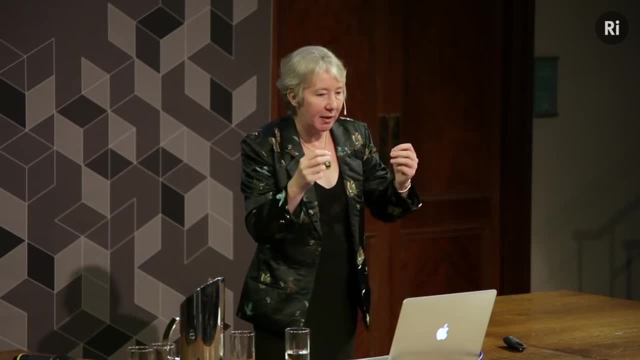 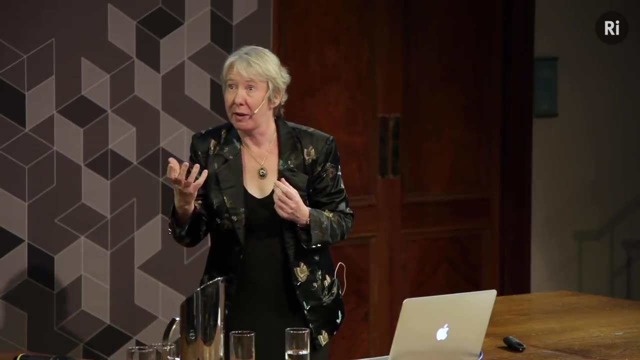 in the experiments. We're going to put more protons in, but we're going to squeeze the bunches more tightly and that will increase the chance that protons collide. So we'll be running at more like five times the nominal luminosity. 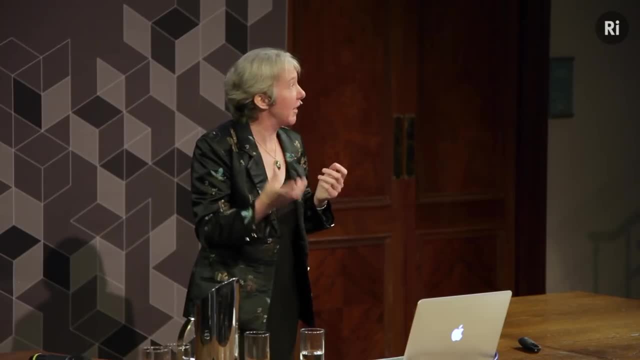 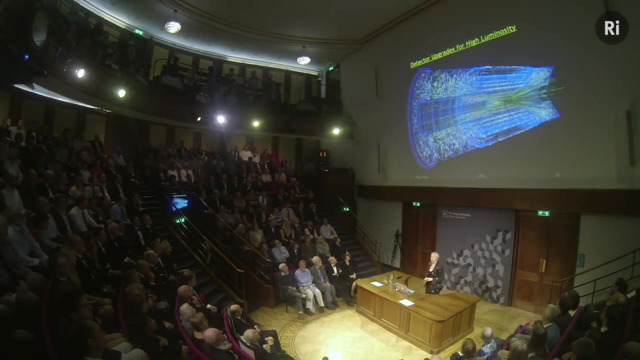 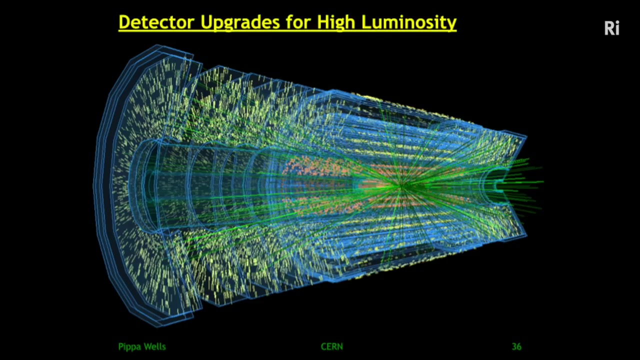 five times the number of collisions, And so that way in another decade we could collect ten times more the original design data set. If we're going to run at five times the nominal luminosity, we also have to upgrade parts of the detector. 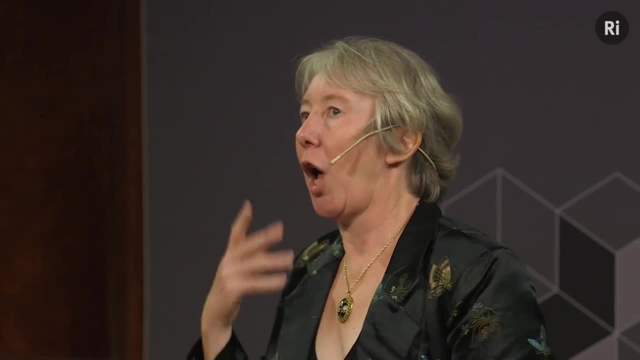 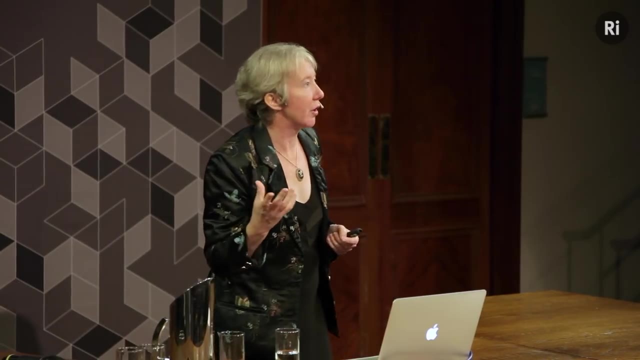 So if we have a cracker that fits on the table, it can cope with 20 or 30 collisions in the same bunch crossing. It can't cope with 150 or 200 collisions in the same bunch crossing. So we're working out what we need to do. 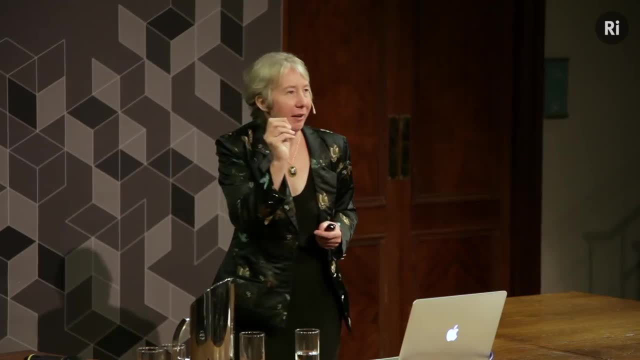 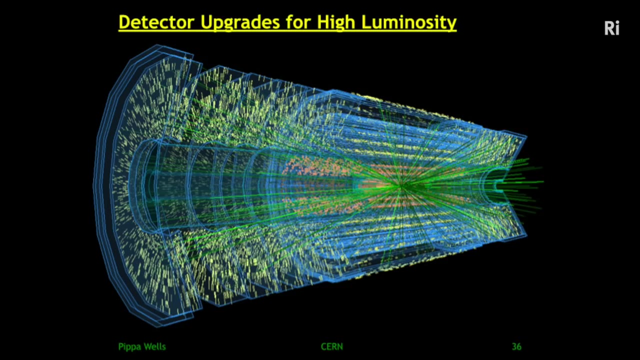 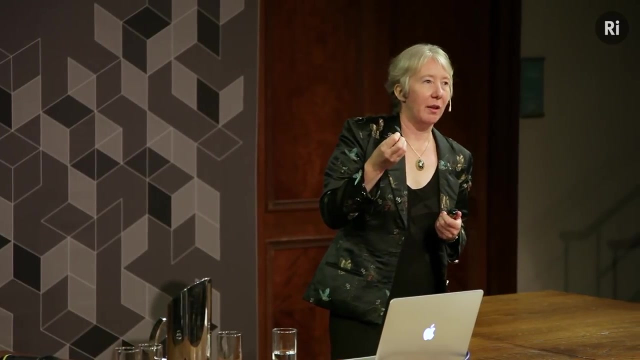 We need to make a new detector with finer granularity detector elements. This is a simulation of the new detector we're planning to build, where we're validating that indeed it will work with 200 collision events going on, So we can still pick out those straight tracks of interest. 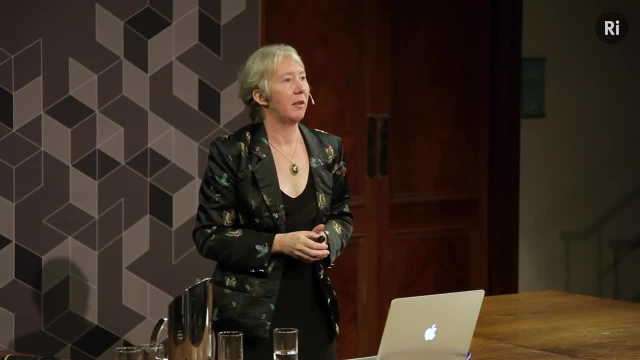 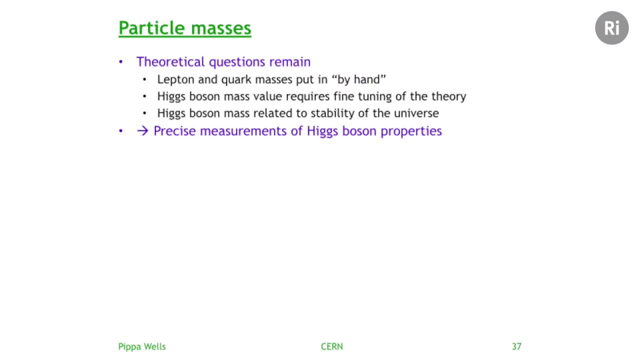 the high energy tracks from amongst all those other softer tracks coming from the ordinary events. So, coming back to the mysteries of the Higgs boson and fundamental particles, there are theoretical questions that still remain. So the mechanism for giving mass to the particles, 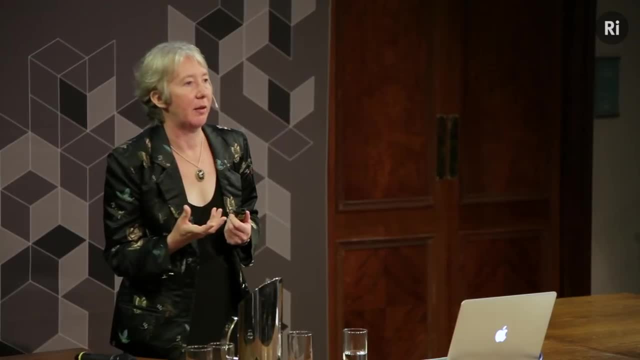 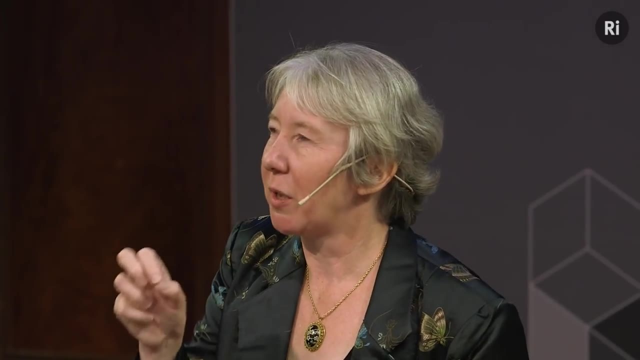 it's really rather elegant than the Higgs boson, the O and Z boson, those force-carrying bosons, But the lepton and quark masses, the masses of the matter particles, are just put in a bit by hand. 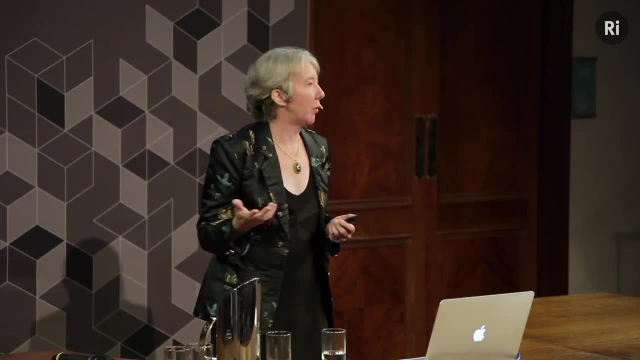 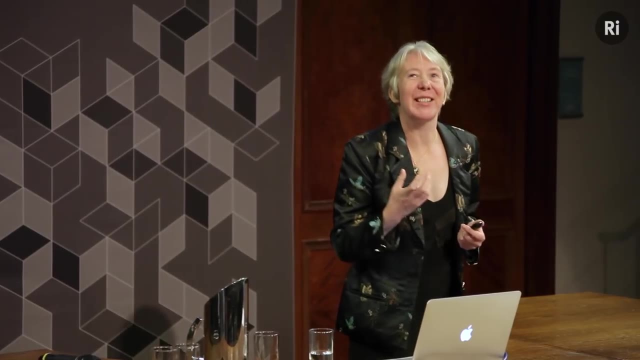 We don't really understand why the top quark should be so massive, 170 times more massive than a proton. Then there are a couple of even more subtle theoretical questions. So it's a quantum theory. All these quantum processes are going on. 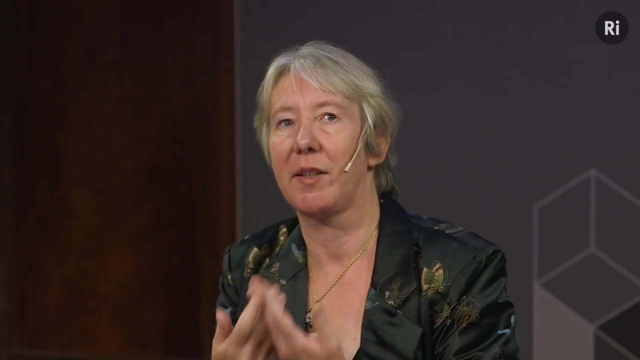 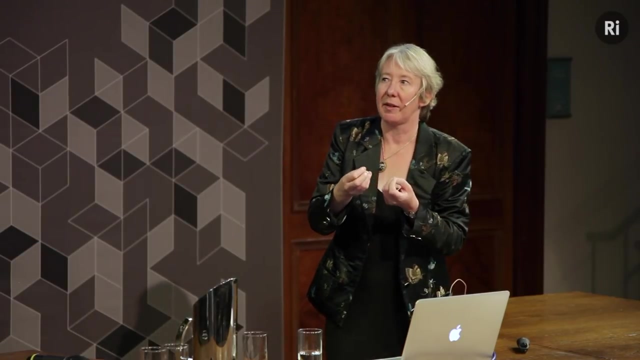 Particles are winking in and out of existence And these quantum processes actually affect the mass of the Higgs boson. The Higgs boson mass that we measure has been influenced by all those quantum processes And in trying to calculate the Higgs boson mass, it's really tricky to get it to stay small. The contributions tend to pile up on top of each other, So it requires a bit of fine-tuning of the theory for the Higgs boson mass to come out small, And the Higgs boson is going to cause. 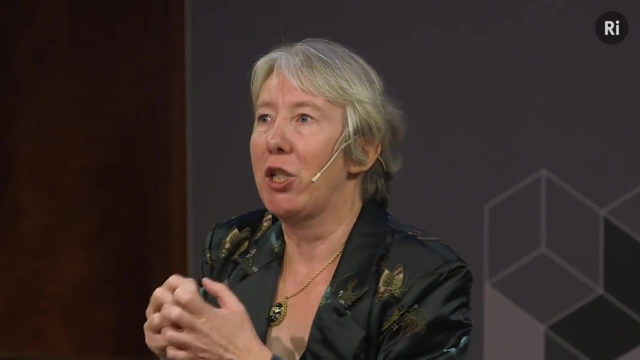 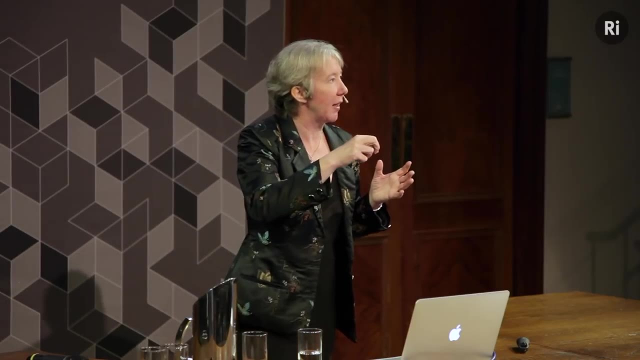 the universe to be unstable. So that's to do with the amount of potential energy locked up in the Higgs field. The Higgs field's really unusual because its preferred value isn't zero. That's how it's giving the mass to the other particles. 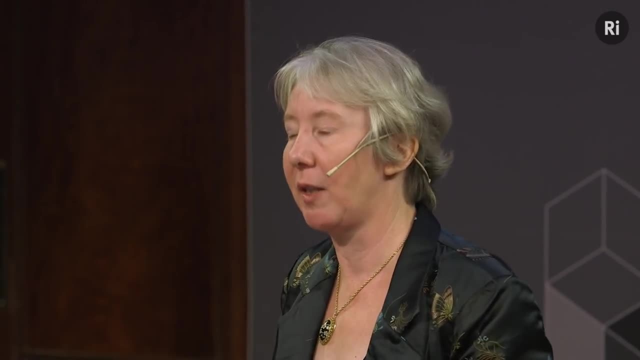 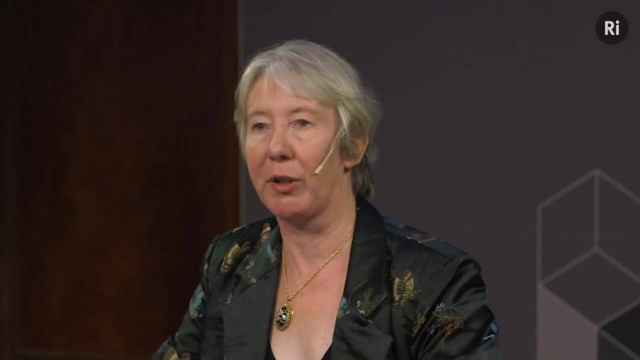 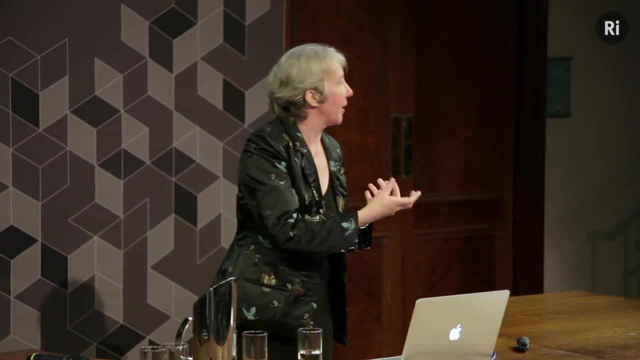 Its lowest potential, energy is actually away from zero, And that's described as a sort of Mexican hat-shaped potential. There's a peak in the middle, then it drops off, but depending on the shape of that potential, that tells you something about the Higgs mass as well. 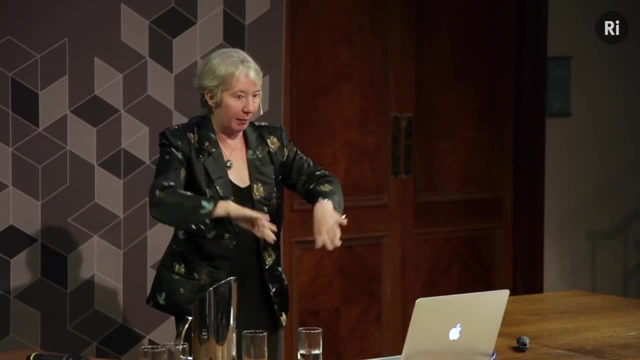 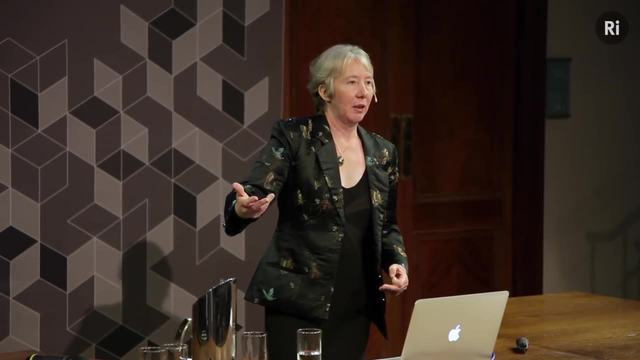 And where the Higgs mass is sitting. it's not quite clear if the brim of the Mexican hat actually flops over again, and there's an even lower point further out that the universe might prefer to sit in. On the other hand, it's a quantum process. If I'm sitting in a valley and there's another valley further along that's even lower, I've still got to climb that mountain to get over there. It's been here 13.8 billion years already. It seems fairly stable, So we can make precise measurements. 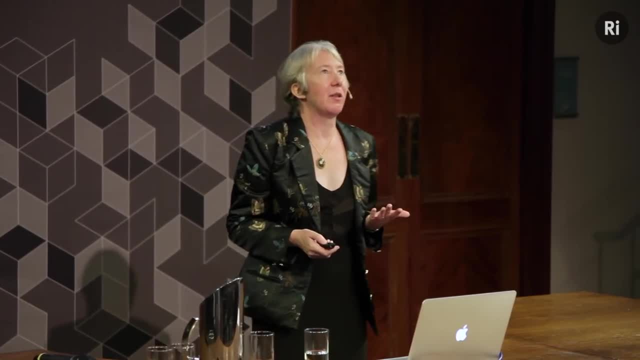 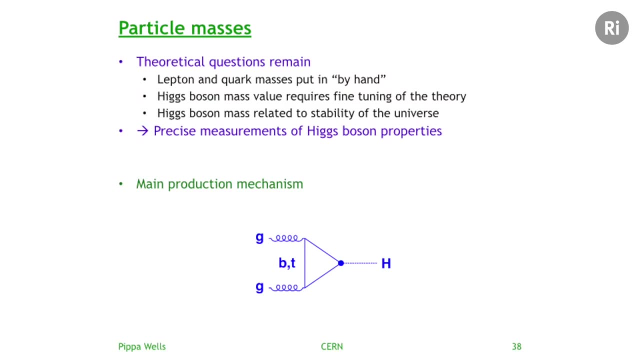 of the Higgs boson and that can give us maybe an insight into these tricky theoretical questions. The main way of producing a Higgs boson is through collisions of gluons, So it's a gluon from each proton that gets picked up. 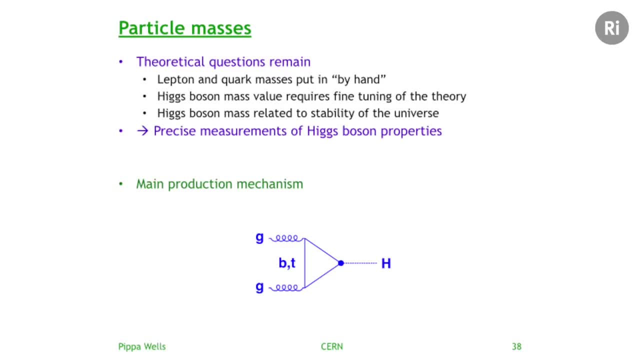 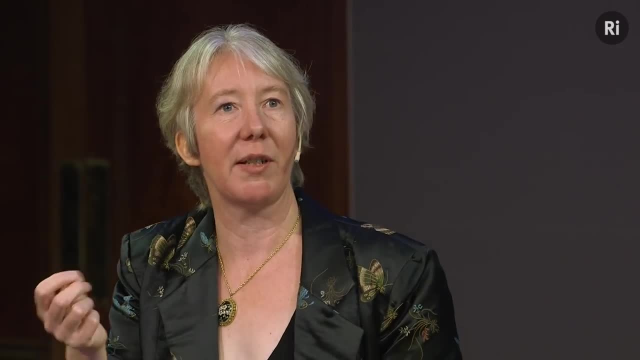 But the gluon is a massless particle. So actually the gluon can't connect straight to a Higgs boson. It's a massless particle. It requires one of these tricky quantum mechanical processes where the gluons themselves wink out of existence. 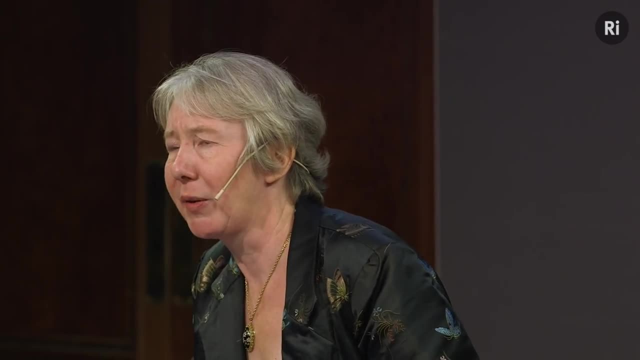 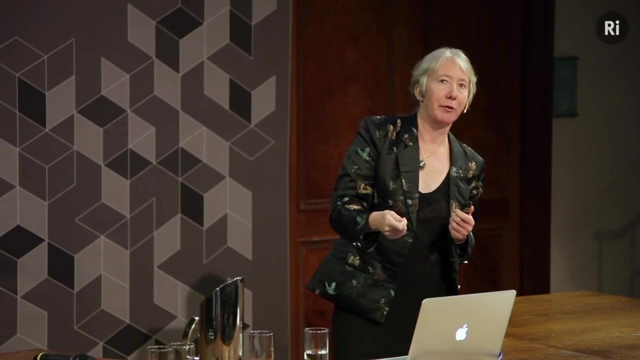 and go via some heavier particle to make a Higgs boson. So that's actually a very rare process. That's why we only get one Higgs boson every two seconds, even when we're running at full tilt. Then there are rarer processes. 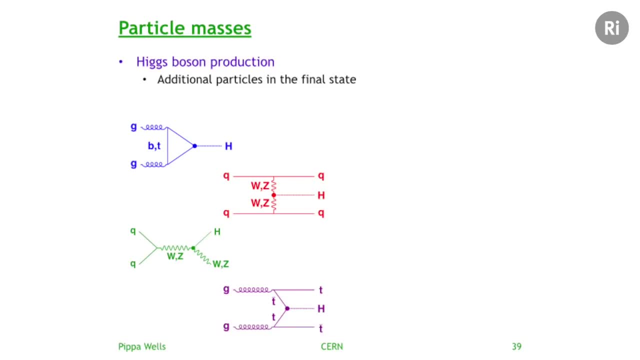 even more complicated processes where, as well as the Higgs boson, you get some extra particles. So in this kind of process I've just got one Higgs boson. If you look at the Higgs there's something else, Some extra quarks. 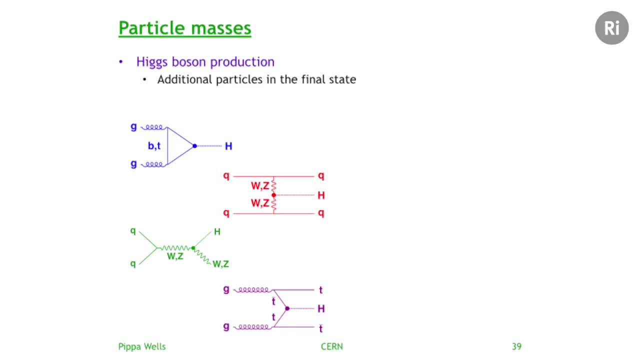 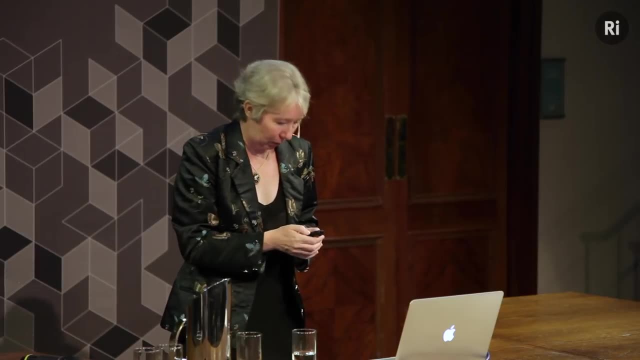 or a W and Z boson, or even a top quark-antiquark pair, Really heavy particles. So if we double the machine energy, we're more likely to be able to see all of these processes, especially the ones with the top quarks. 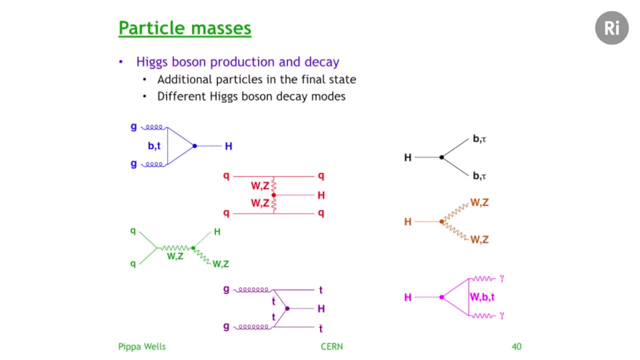 And then we also need to look at the way the Higgs boson is decaying. So it might decay to these particles from the third family, the B quark or the tau lepton. We saw that in the discovery plots The Higgs boson can decay to Z bosons. 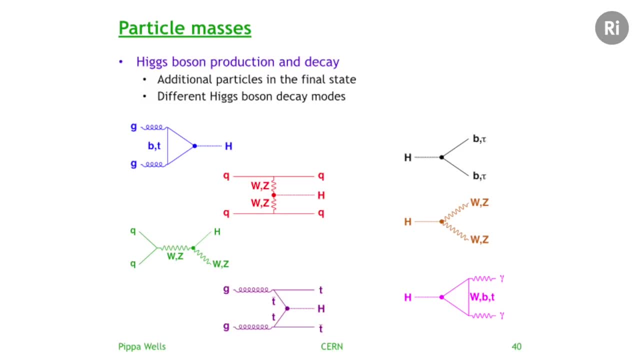 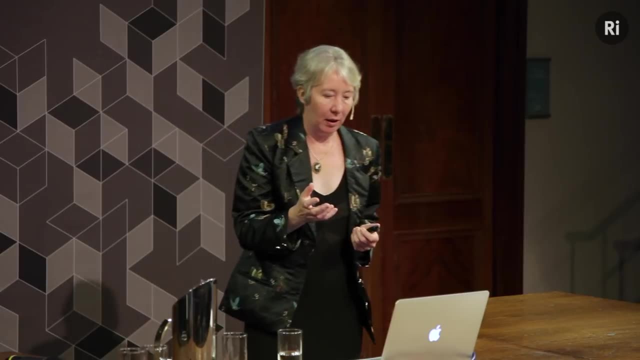 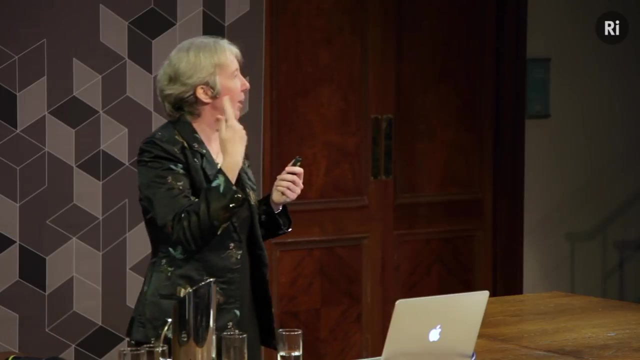 Or it can decay to two photons again via one of these mysterious quantum processes. So if we can measure all these processes very precisely, then it might give us an insight into. does the Higgs boson really just fit exactly into the standard model or is there something a bit new? 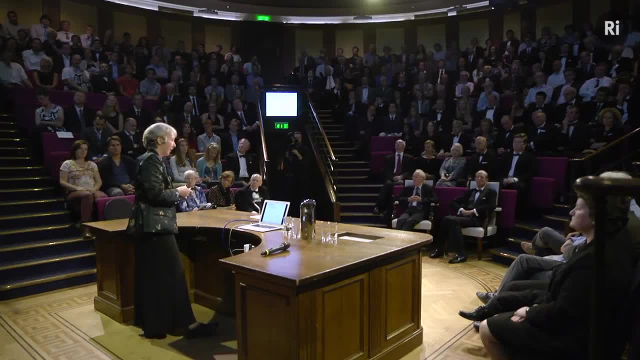 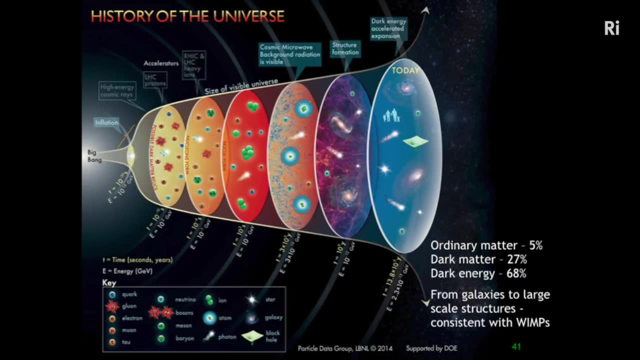 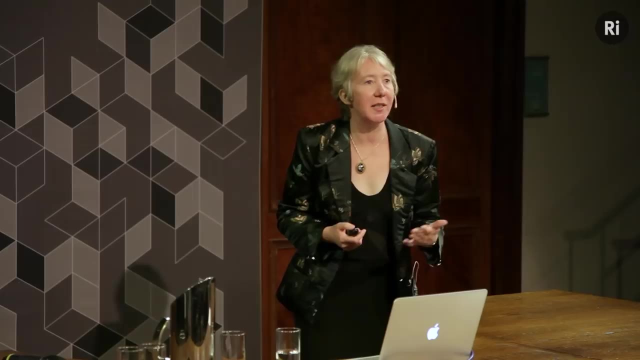 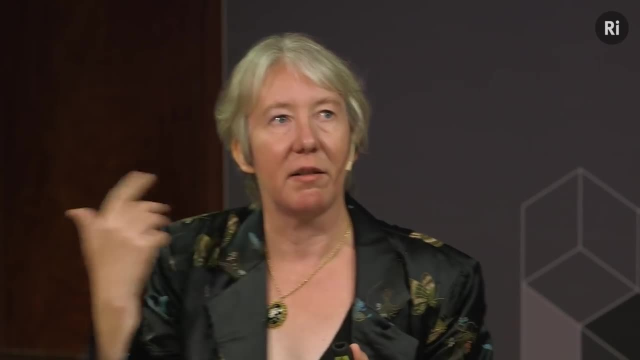 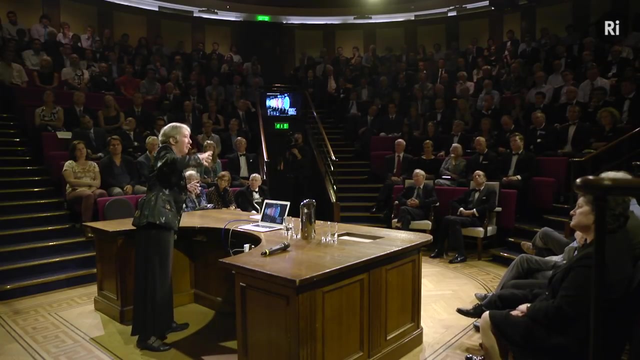 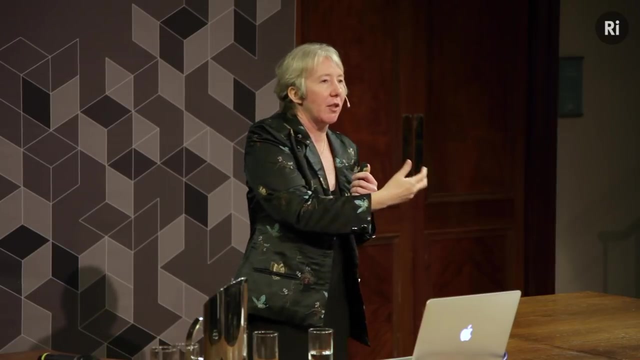 of the galaxy, but the way they rotate it's clear they're actually more like a solid disk. There's a lot of dark matter in the galaxy as well that's not accounted for by the visible stars. The shape of big structures in the universe also needs. 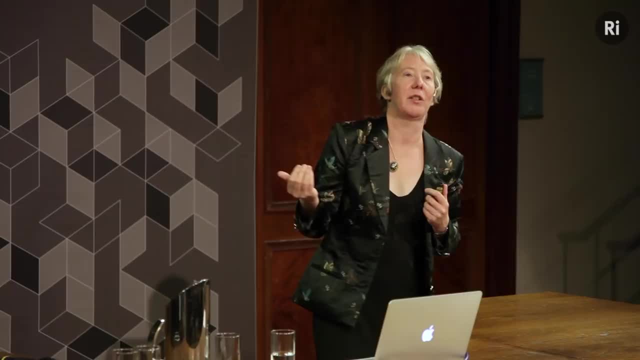 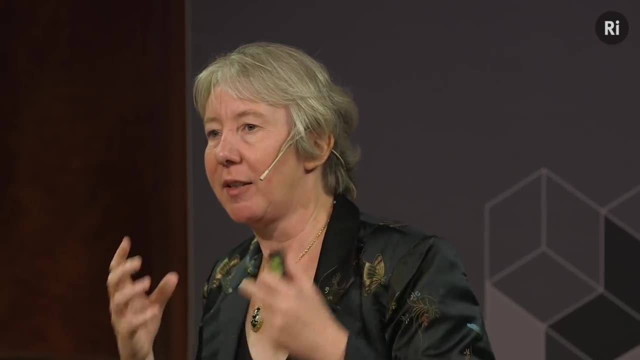 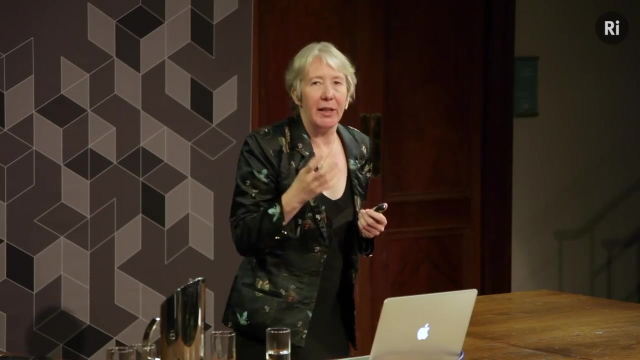 a bit of dark matter and even the fluctuations in the cosmic microwave background. they don't really fit in a model, because you can build a self-consistent model of how the universe has evolved with just one type of dark matter. It can't be neutrinos. They're really too massive. There's not enough matter in neutrinos to be able to say: oh, it's not dark matter, it's just lots of extra neutrinos. That doesn't work, And it can't be bricks or small planets. big chunks of dark matter. 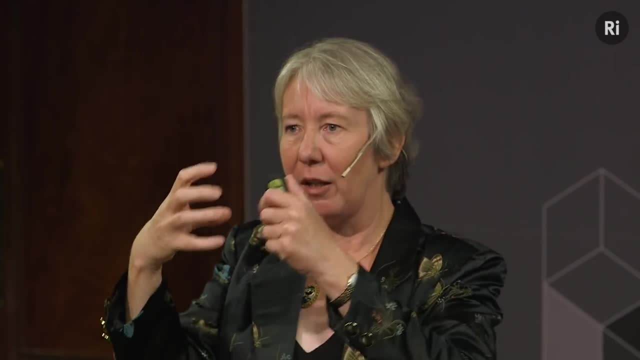 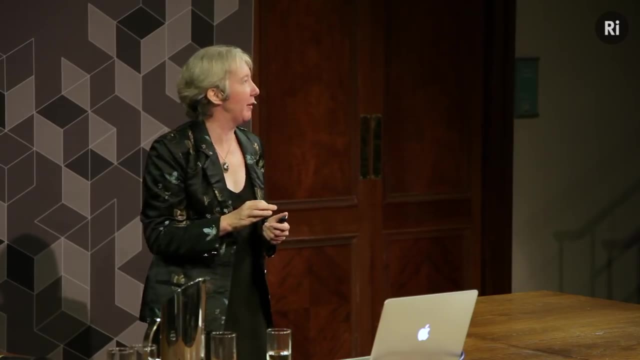 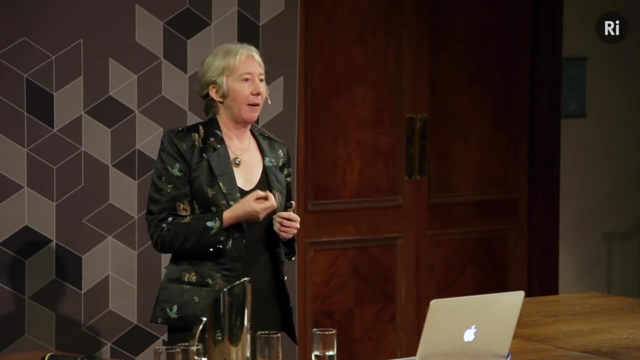 that you just it's ordinary matter, but you don't see it in a project to turn into a star and to shine. No, you need something just right, something in the middle, which is what we elegantly call a WIMP. A WIMP is a weakly interacting. 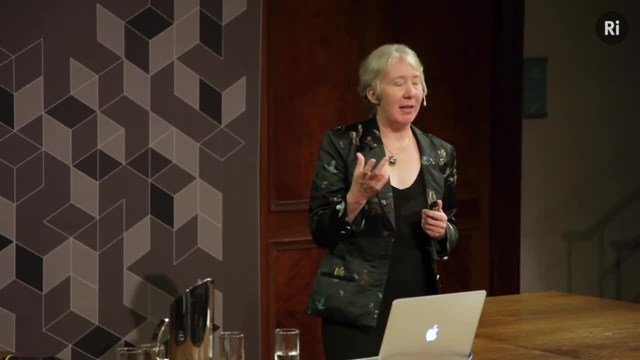 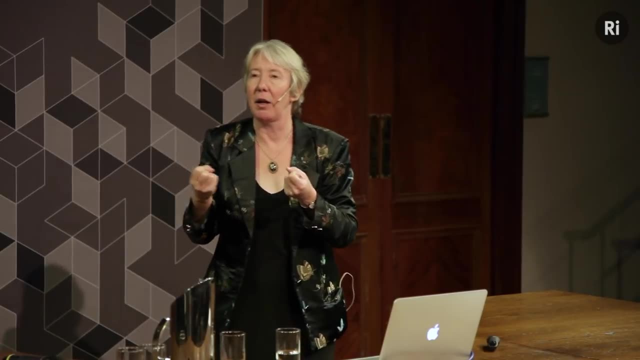 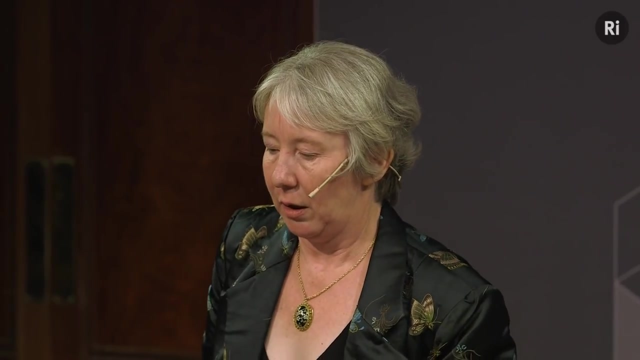 massive particle. So what does that mean? Weakly interacting, meaning it's dark matter, it's drifting around but we see no evidence of it, So it can't be interacting too strongly. It can't have electromagnetic interactions or strong interactions. It's hard to detect. 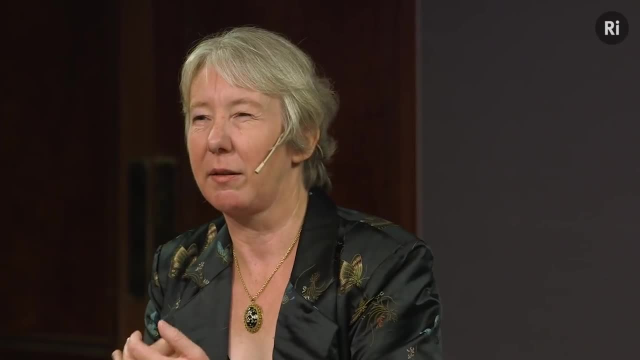 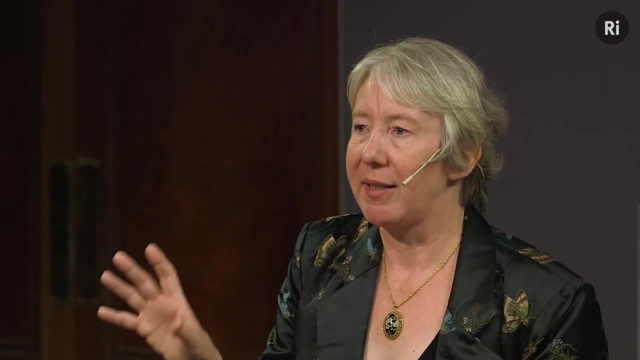 And it's massive in the sense of it's not a neutrino, It's got a mass a bit more like a Z boson or a W boson or a Higgs boson, Some kind of mass in that region. So that's great. 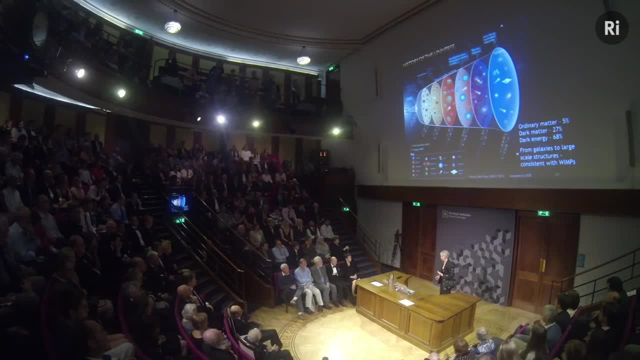 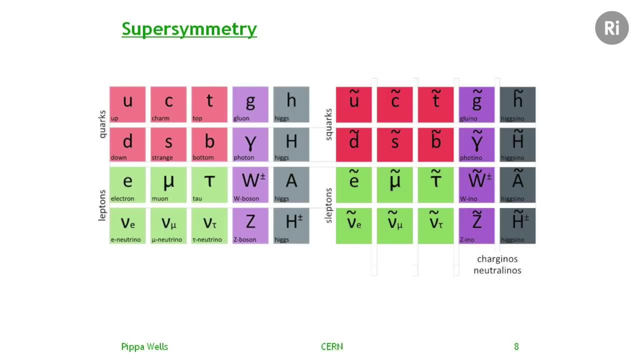 That means we might actually be able to make these particles in the LHC. Now, supersymmetry is one possible theory for helping to explain dark matter. But it's not just dark matter. Supersymmetry has two or three really quite useful features. 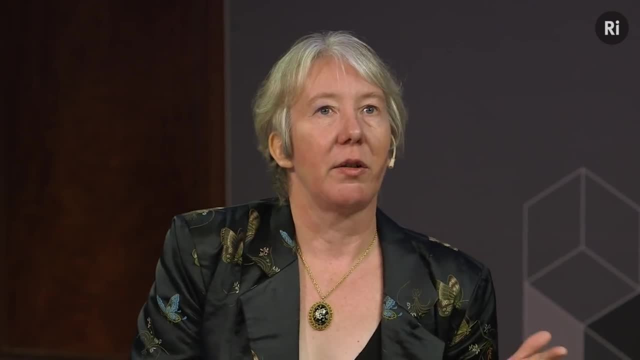 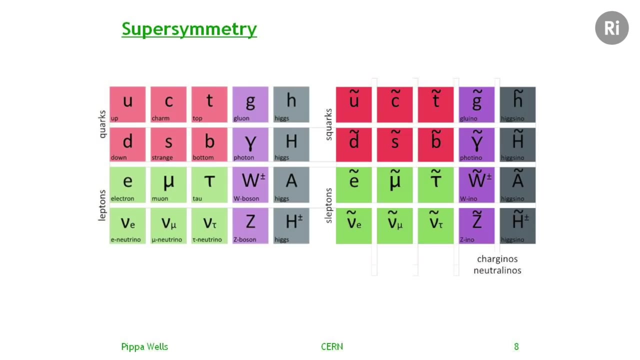 What does supersymmetry do? Well, we've got our standard fundamental particles of the standard model that we've already been introduced to on the left, And then all of those have a supersymmetric copy, So it's a heavier copy. And what's happened in the supersymmetry? 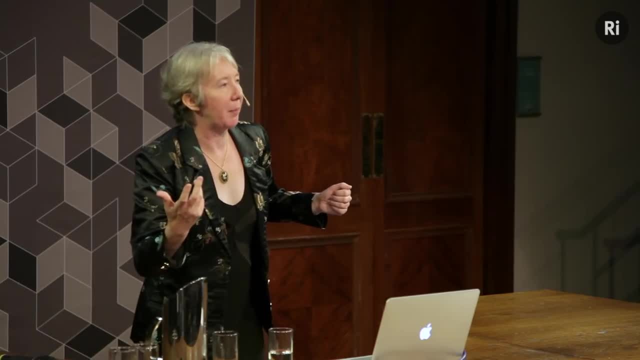 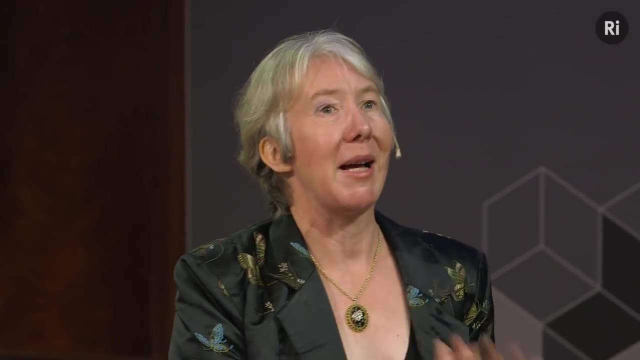 is the force particles and the matter particles have sort of got mixed up. There's a particle that looks a bit more like a matter particle. I've also sneaked in some extra Higgs bosons If you're going to give mass to all of these extra fundamental particles. 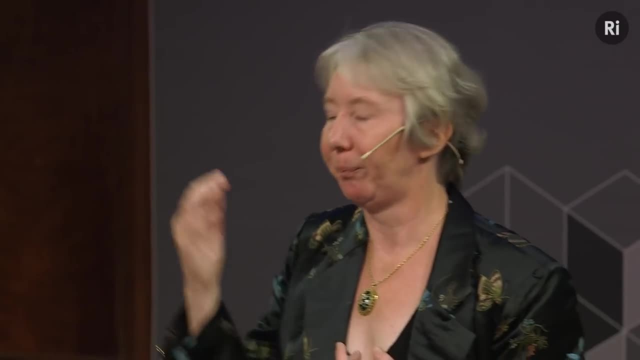 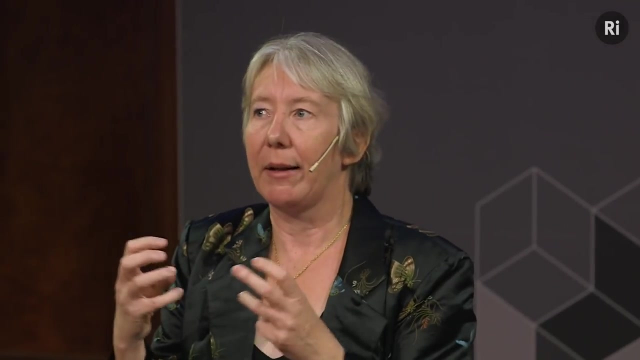 you actually need a slightly more complicated Higgs sector. You need five different Higgs bosons. So one advantage of supersymmetry is now all these quantum mechanical corrections to the Higgs mass which I told you were really hard to keep under control. 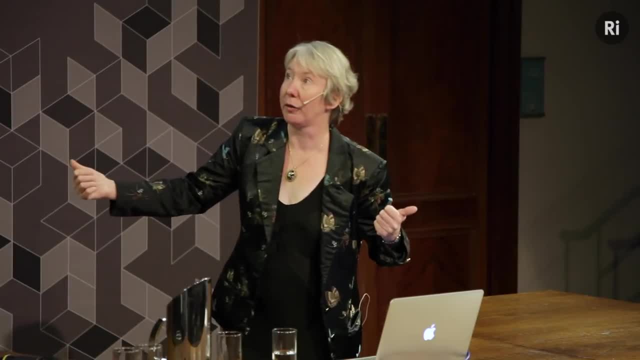 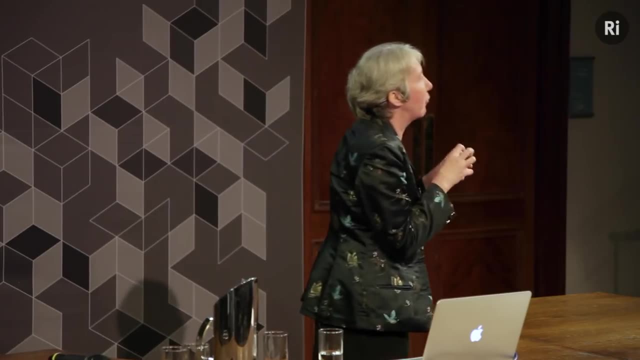 they start to cancel out because the contribution from the normal particles and the contribution from the supersymmetric partners- And it's also quite a convenient theory if you're trying to fit gravity into the picture- A lot of the theories trying to bring in a force particle. for gravity that you'd call a gravitino. they need supersymmetry. They only work if you've got a supersymmetric universe, But best of all, is that one of these supersymmetric partners of the force particles, if you choose a neutral one. 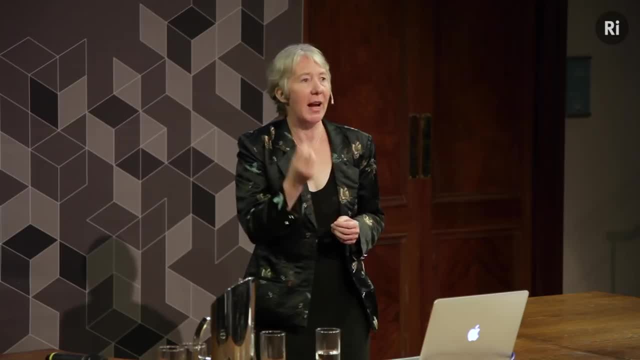 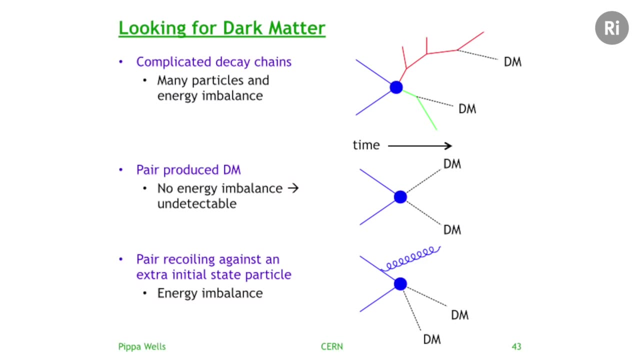 the lightest neutral supersymmetric particle, it's an excellent candidate for dark matter. So how do we look for dark matter? at the LHC There are lots of new supersymmetric particles. It could be quite a complicated decay chain. Two particles collide. 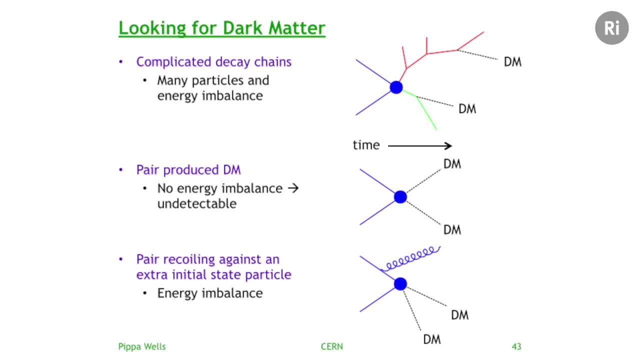 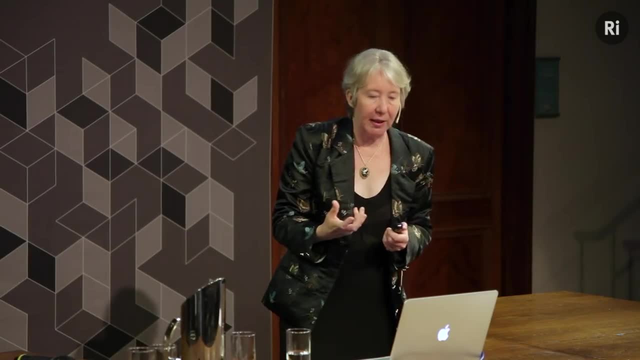 You have to keep in mind, time is running from left to right in this picture. So two things collide- quarks or gluons- and they make a bunch of supersymmetric particles. But whether it's a simple decay chain or a complicated decay chain, 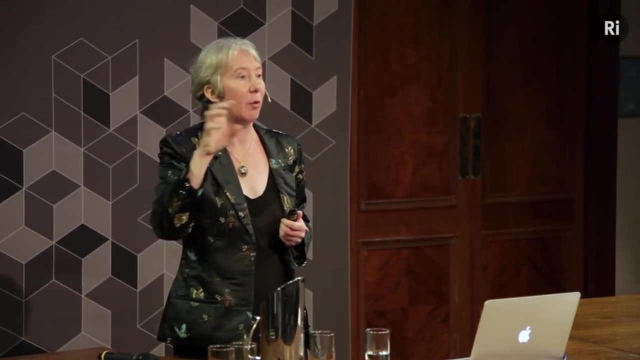 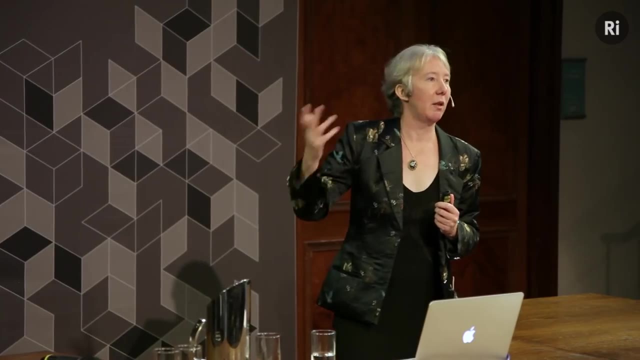 there are some dark matter particles left over at the end that we can't detect. So as far as we're concerned, it's missing energy in the detector. So we can look for events with jets or leptons and some missing energy, more missing energy than we have expected. 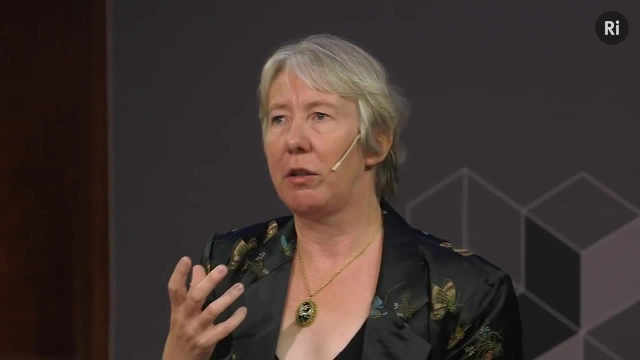 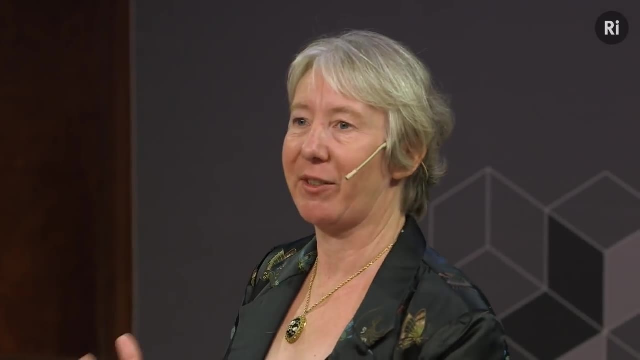 But what about if it's just dark matter, if you can't make any supersymmetric particles or it's a different process? All you're making is pairs of dark matter particles. Well, that's great. You can't see them. They're completely invisible. 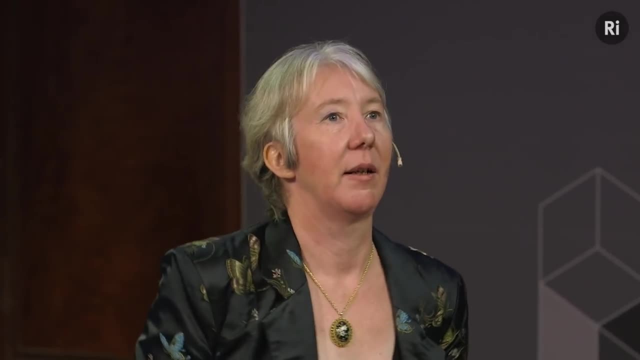 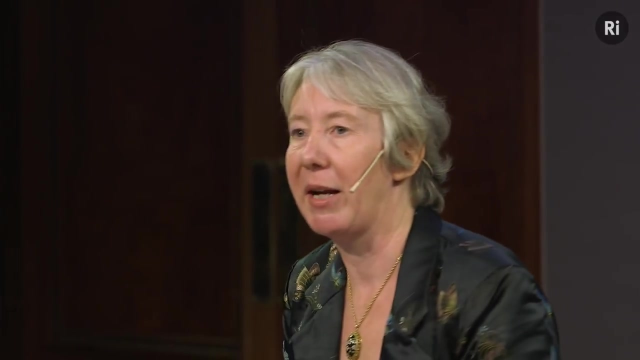 No way of picking them out. All you've got is missing energy. There's nothing balancing it. But then we've got a trick we can play. We can look for events where, before the two dark matter particles were made, something else has been spat out. 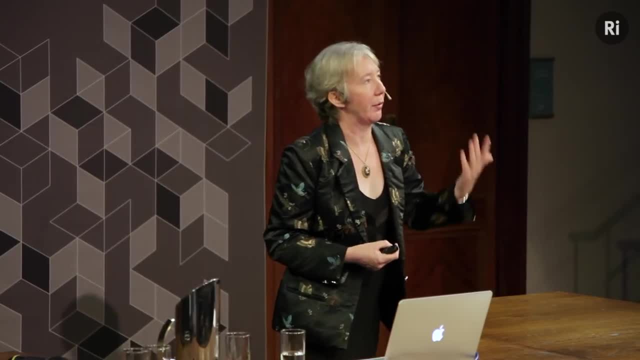 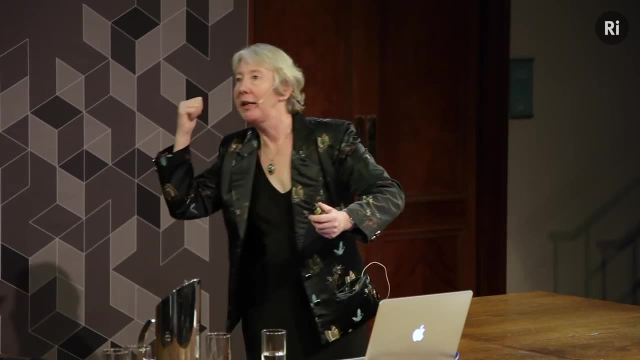 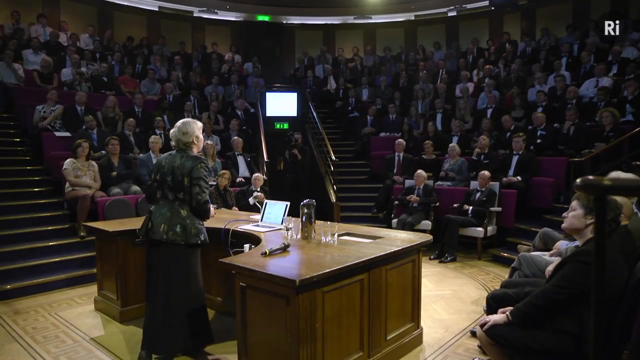 like a high energy gluon or quark or lepton. So now we've got one normal particle in the event that we know how to detect and recoiling against it, these two dark matter particles that are invisible. So here's an example of such an event. 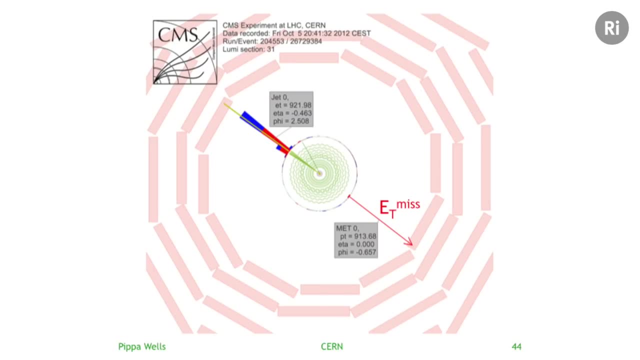 This is from the CMS experiment. There's a very energetic jet going up to the top left and it's balanced by invisible energy. There's nothing balancing it. Whoa, Does that mean we've discovered dark matter? Well, unfortunately no, because there are. 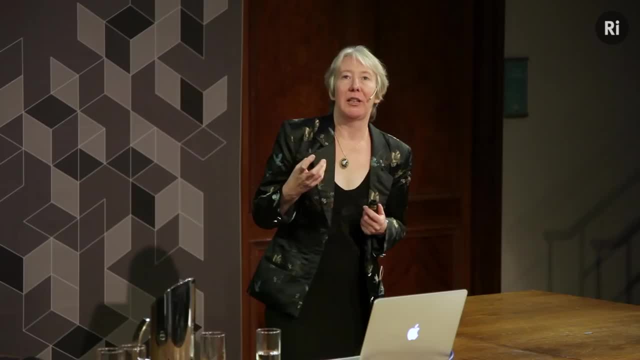 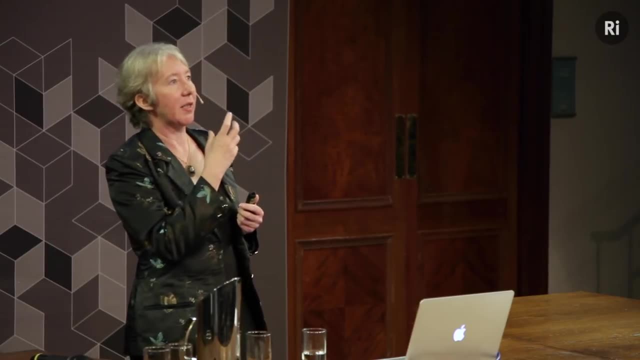 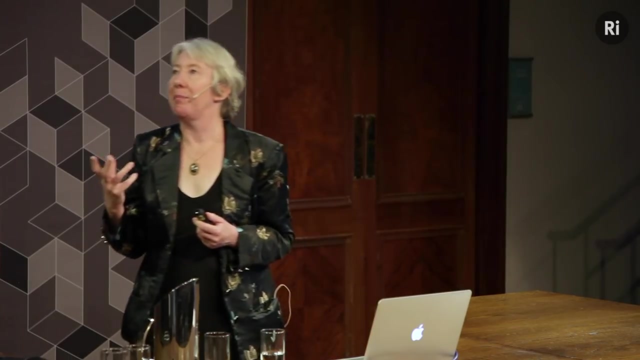 other processes that can also mimic this signal. The most likely is that a Z boson is being produced And, as well as decaying into charged leptons, a Z boson can decay into a neutrino and an antineutrino, So that would be the Z boson. 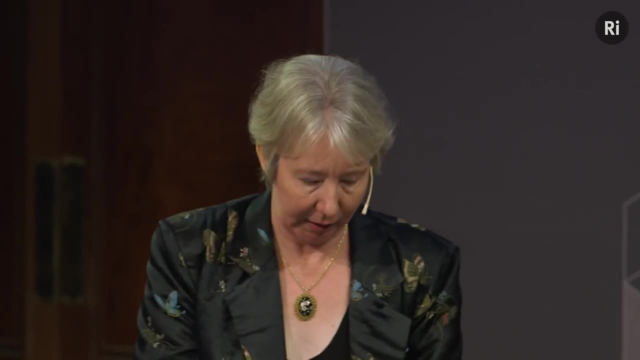 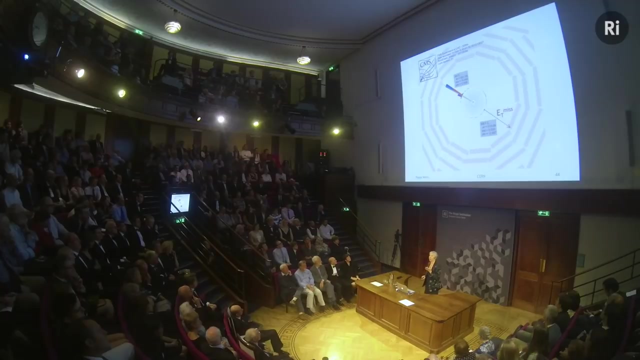 decaying into invisible particles and it would give a signature just like this. So we play a similar game. We plot the distribution of events with a single jet and missing energy, And this is what it looks like. This is from a real physics paper. 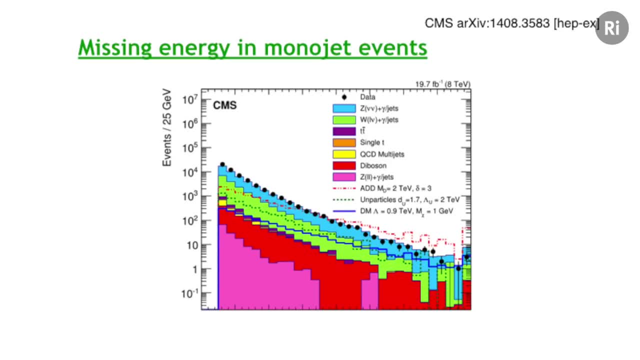 a recent physics paper from CMS, So it's a bit crowded. They've put all the information into this plot that the physicists might want to know about, But you can see that there are black dots. that's the data, that's the rate of events. 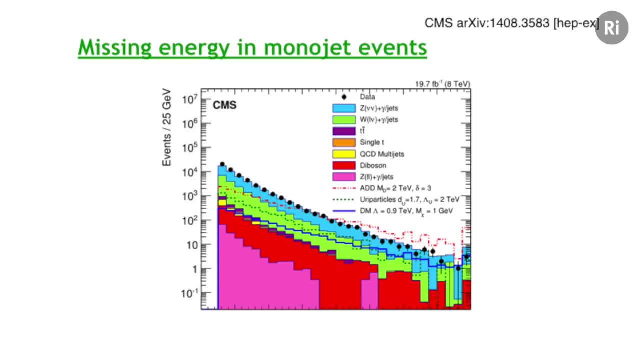 the number of events they've seen with just a single jet and missing energy. And then all the different colours are all the other processes. they could think of the blocks of colour that might make that signal. Now it's a logarithmic scale. 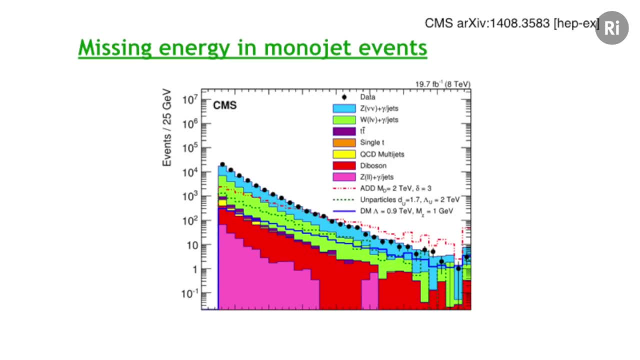 so by far the biggest one is the light blue one at the top. That is events with a Z boson decaying to two neutrinos: One jet, one Z boson that you can't see missing energy. So the dotted lines, 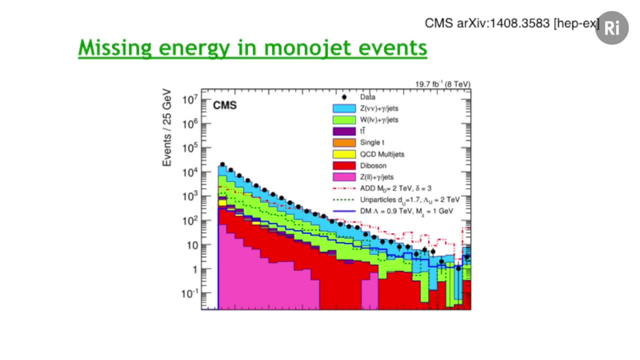 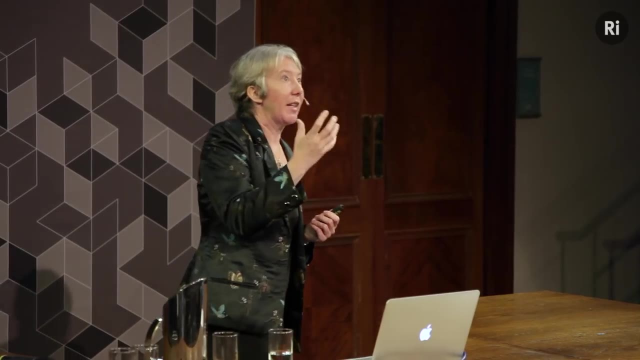 or the solid lines. those are the predictions of various models. So if dark matter particles were being produced, you'd expect to see extra events at the high energy end of the spectrum. So next year, 2015,- if we start running double the energy. 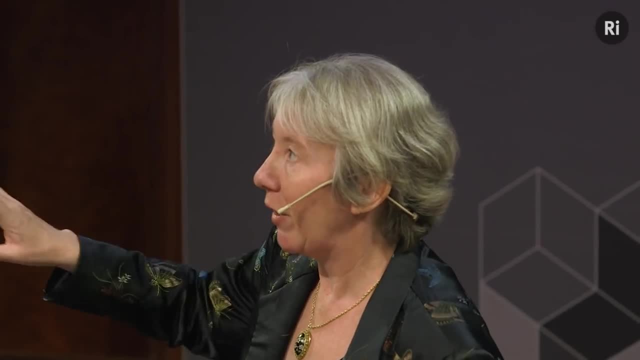 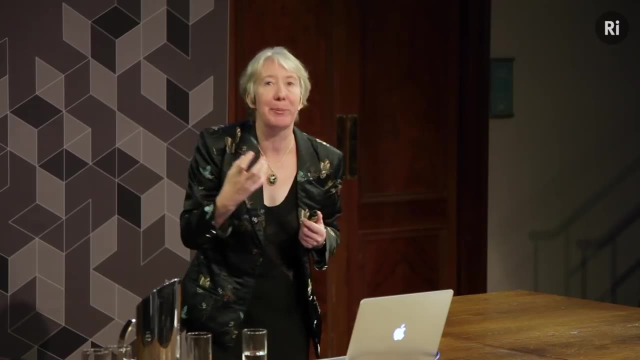 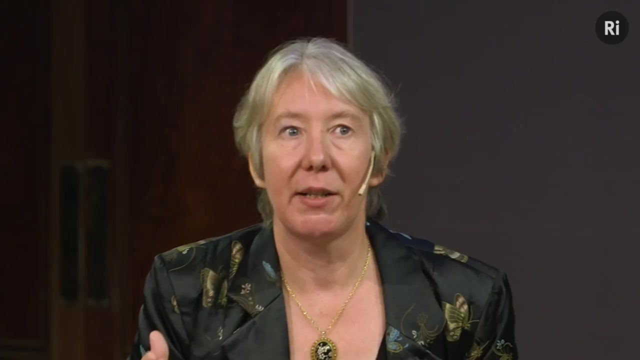 that's going to make it easier to make these events. with very high missing transverse energy, We'll be able to probe this distribution even more. Will some excess of events actually start to appear in this high tail? And if we can collect 10 times more data? 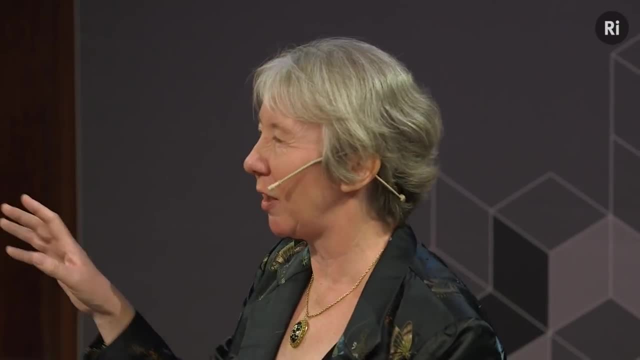 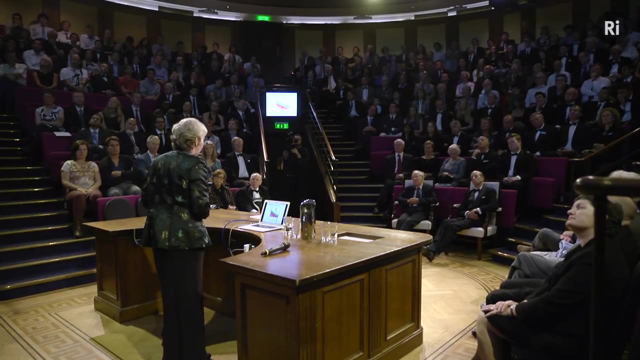 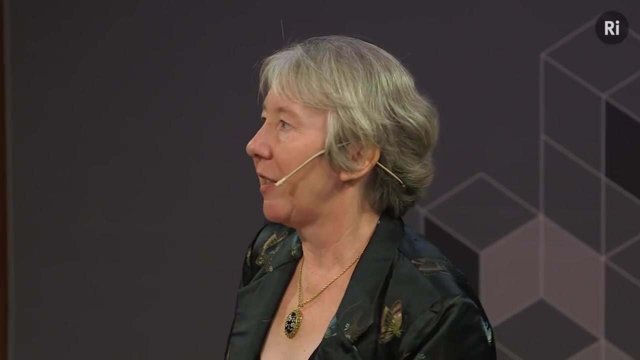 or 100 times more data again, we can really be sure. does it just look like standard processes, or is there really something new starting to emerge Now? the last mystery of all is gravity, And there are a few theories that can try to explain. 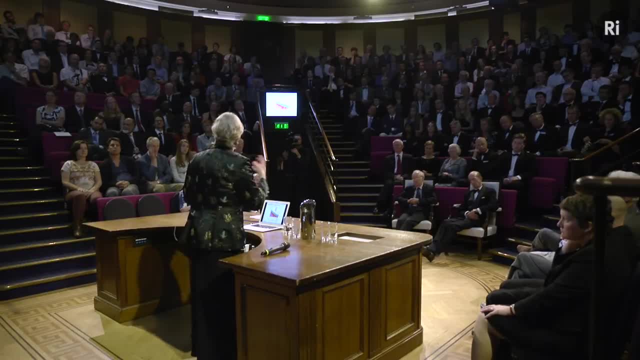 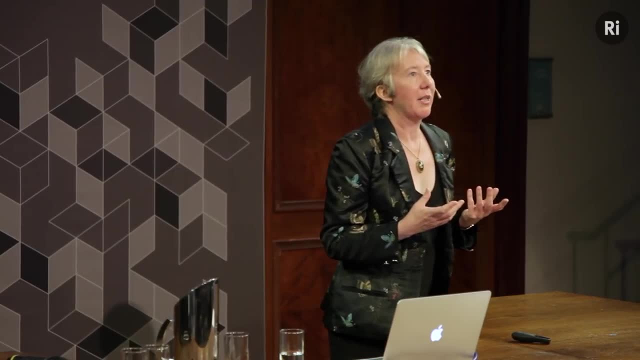 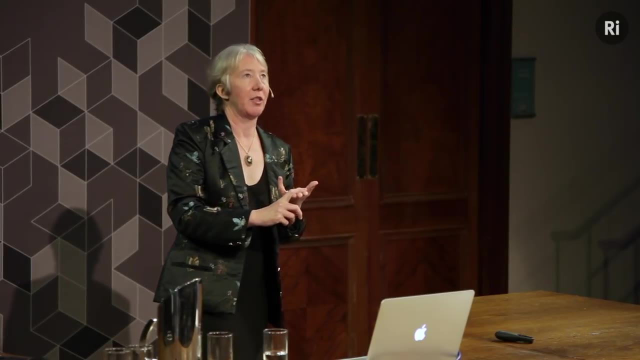 why is gravity so weak? Why isn't gravity as strong as the electromagnetic force or the weak nuclear force? And these theories bring in extra dimensions, But they're not dimensions like we know of. So we know of one time and three space directions. 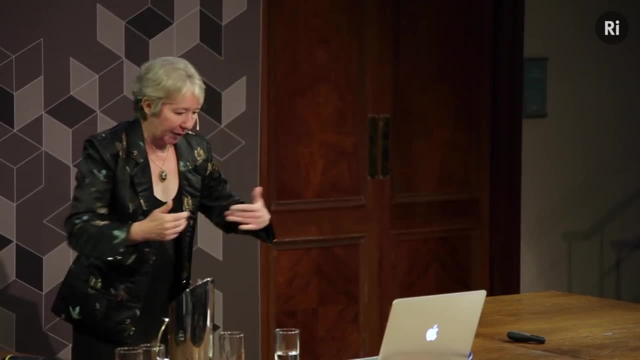 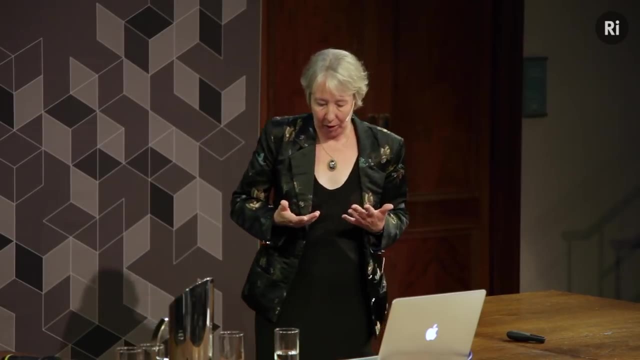 So the clock's ticking and I can move forwards and backwards, sideways, and I could jump in the air. So three directions that I can move in, Three spatial directions plus time. But then there could be extra dimensions that are so small I can't. 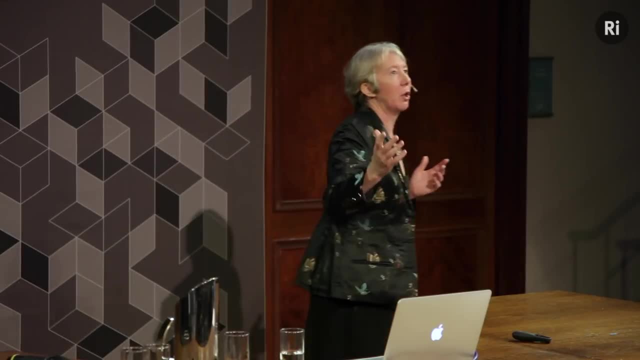 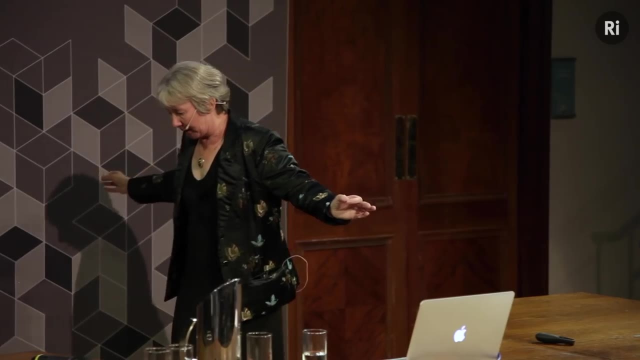 I'm not sensitive to them. And to give you an idea of what I mean by that, imagine you're walking along a tightrope. Or, if that makes you uncomfortable, imagine I'm walking along a tightrope And I can only go. 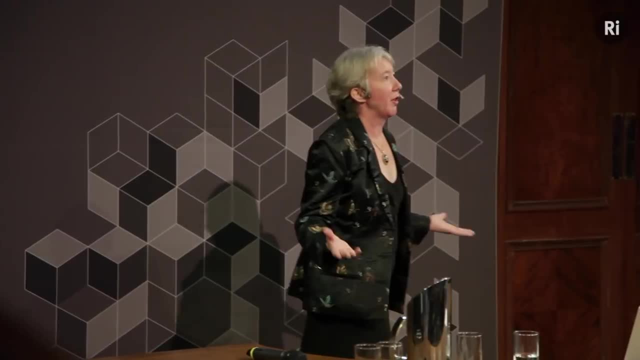 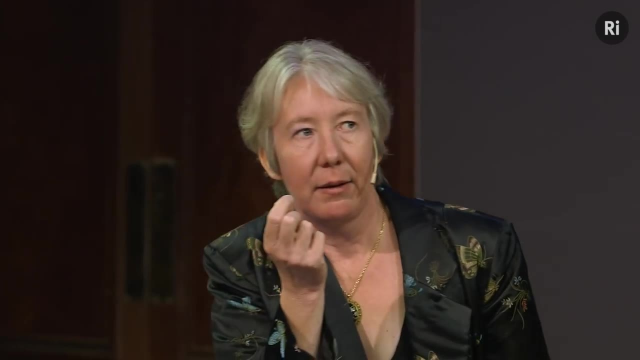 in one direction. I can only go along the tightrope. I can only move in one dimension. That's all I've got open to me Now. if there's an ant on the tightrope, it's a substantial rope, right. 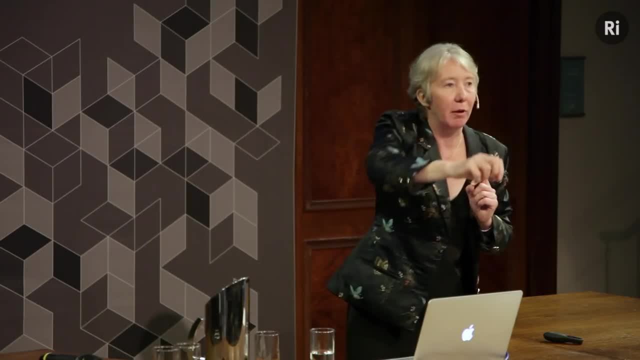 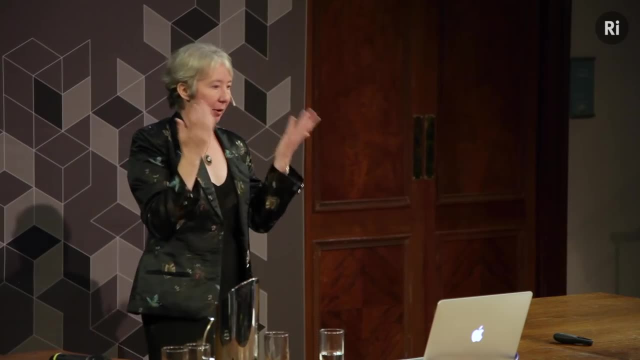 The ant can walk along the rope, walk along the tightrope, but it can walk around the tightrope. So, as far as the ant's concerned, there are at least two dimensions. As far as I'm concerned, there's only one dimension. 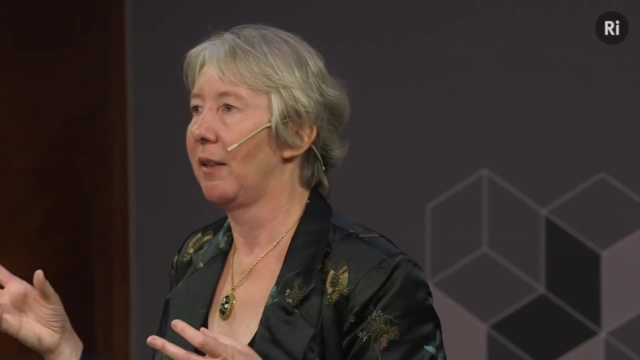 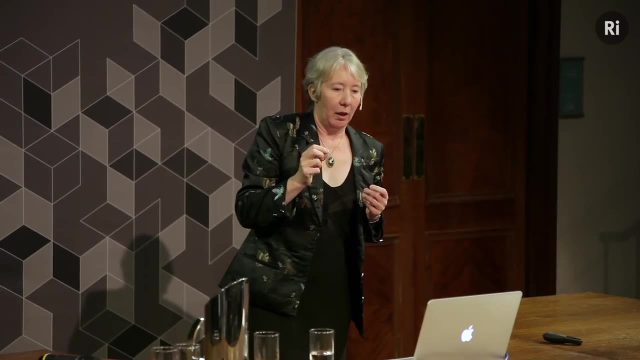 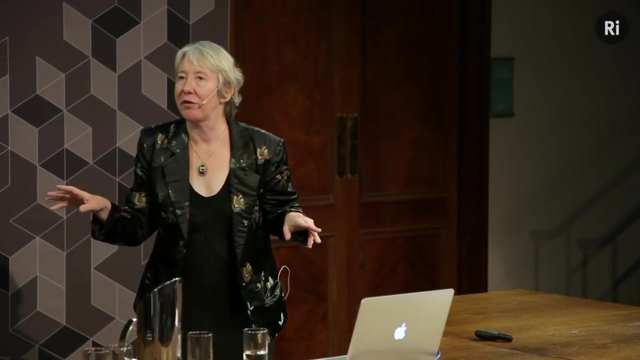 And that's what these theories are trying to do. They build geometries of space-time with these tiny curled-up, compactified dimensions, And gravity could see all these extra dimensions. The gravity's kind of diluted because it leaks out into these extra dimensions. And the other forces only see the three normal directions And you can create extra particles. If you make high-energy collisions you can. then in these theories you can start to probe these extra dimensions And one of the extra particles you might make. 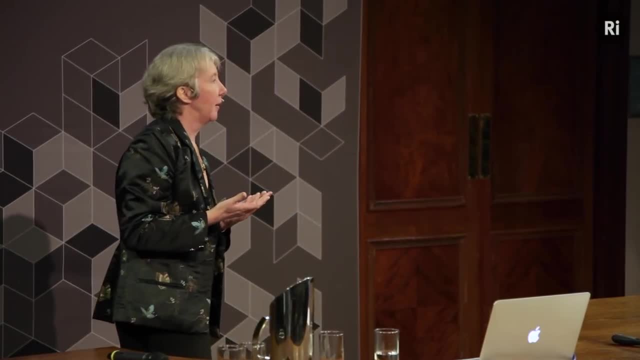 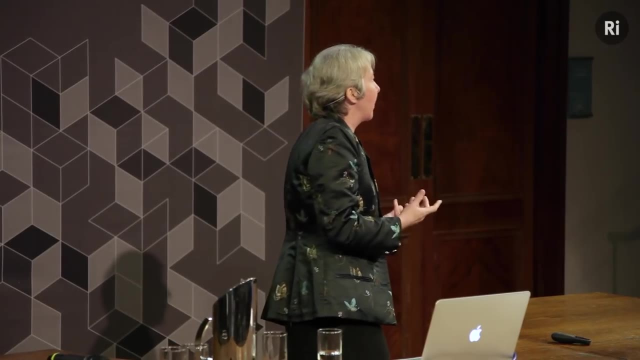 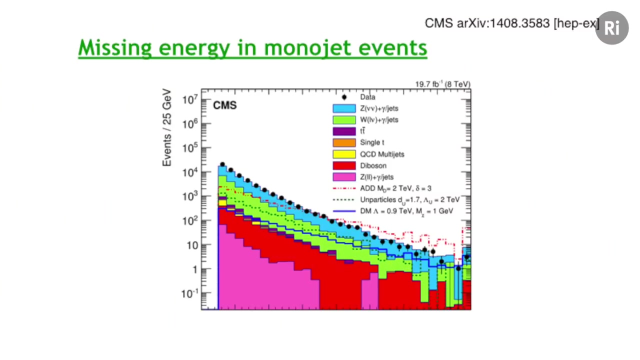 is the graviton, the fourth particle of gravity, But it would be invisible. So you can use this very same plot to put constraints on if there are extra dimensions. And in fact that's what's shown here. The headline is actually: what would I expect to see? 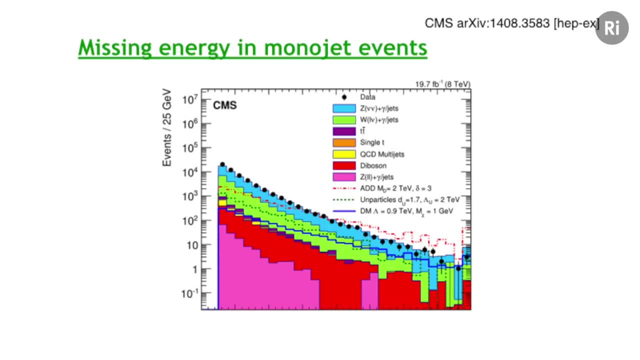 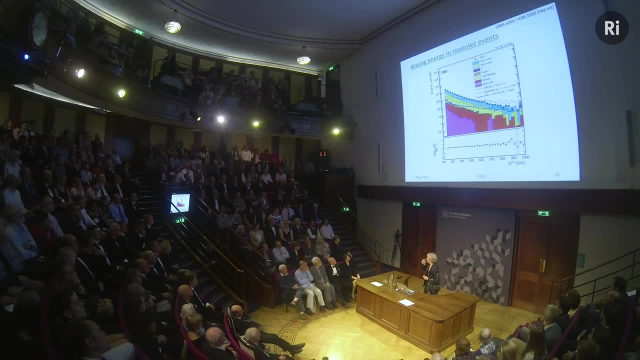 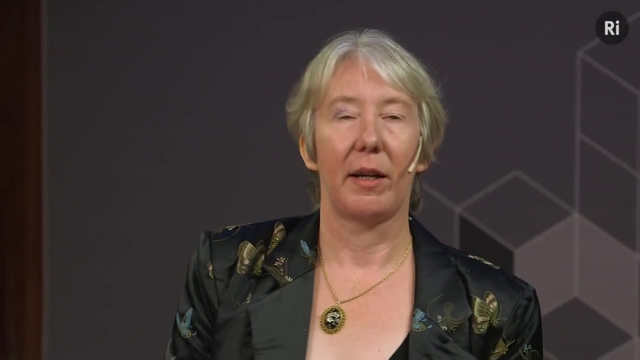 in this E-T misdistribution, in this missing-energy distribution, if there really were these extra dimensions and I was producing gravitons. But there are other things that can happen. if you create a theory with these extra dimensions, You might actually make particles. 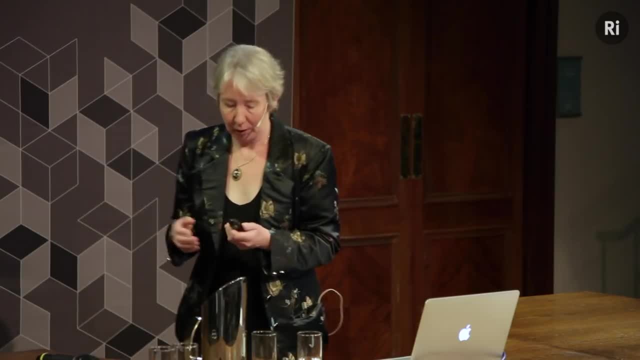 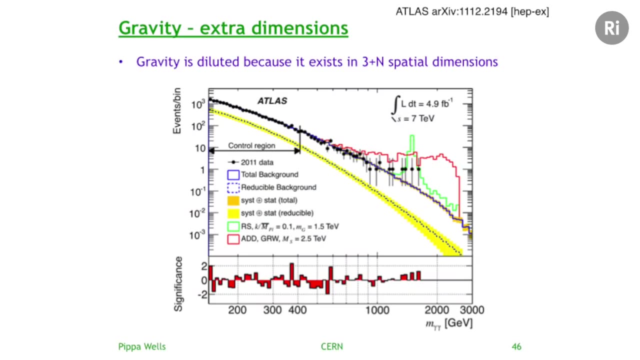 that decay in a visible way. So let's have another look at that two-photon mass spectrum. This is from a paper by Atlas. It's a slightly older paper, but I've picked this plot because it illustrates a few points that I wanted to make. 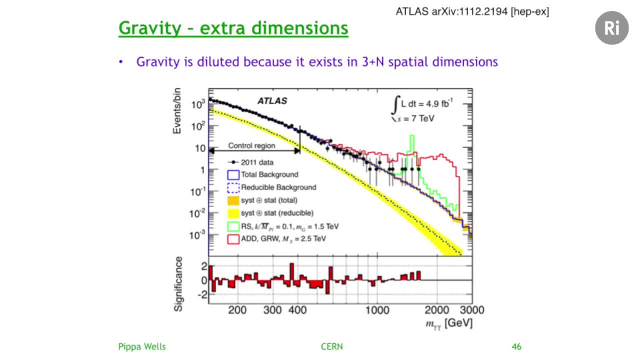 The gravity is diluted because it's leaking away into these extra dimensions, And there could be new particles that decay into two photons, Either just particular mass values with a big difference between the mass values. So that would create something like the green curve, a well-defined bump. 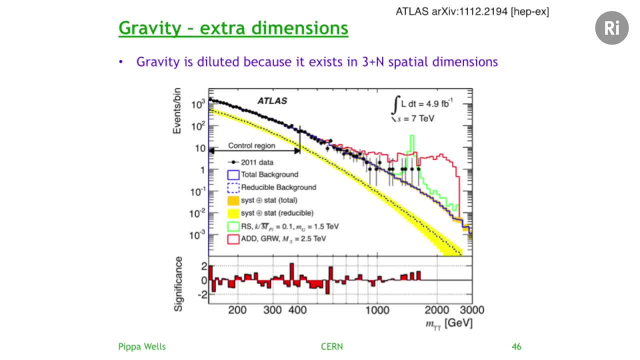 in the tail of the two-photon mass distribution, Or there could be lots and lots of new particles being created So you can't really distinguish between them. It just looks like an excess of events being produced. So that would be the red curve. 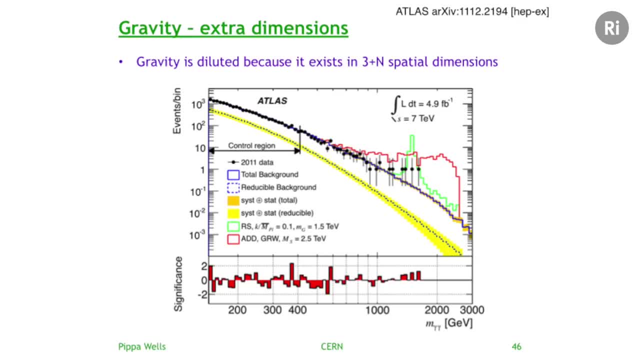 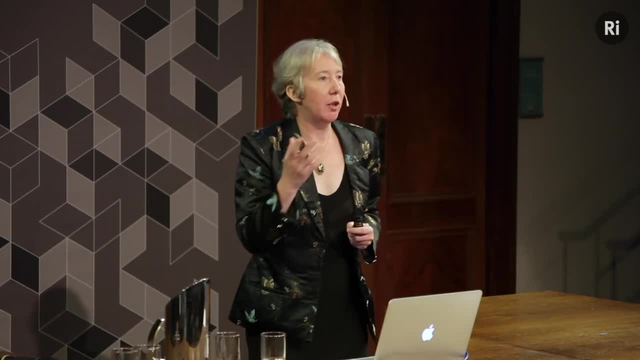 So this is the two-photon mass spectrum, but it's way higher energies than where we discovered the Higgs boson. The same thing applies. There's nothing new here yet, but we're going to start running at twice the energy just next year. 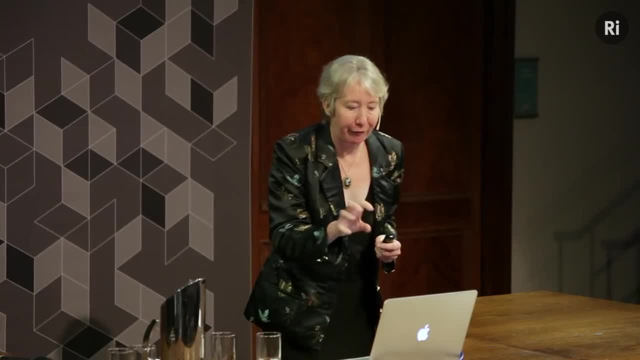 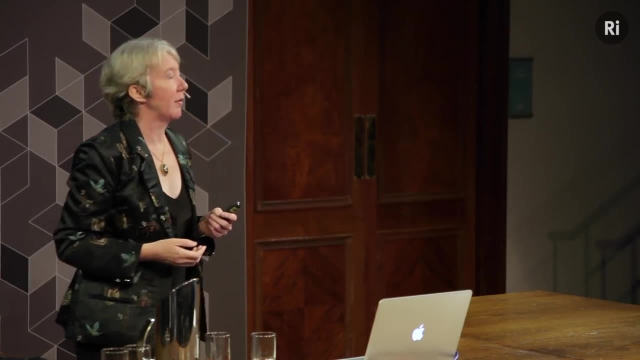 So we might start to be able to make something that fills in this high mass tail of the two-photon mass spectrum or of that two-jet mass spectrum we were looking at towards the beginning of the talk, And we're going to take 10 times more data. 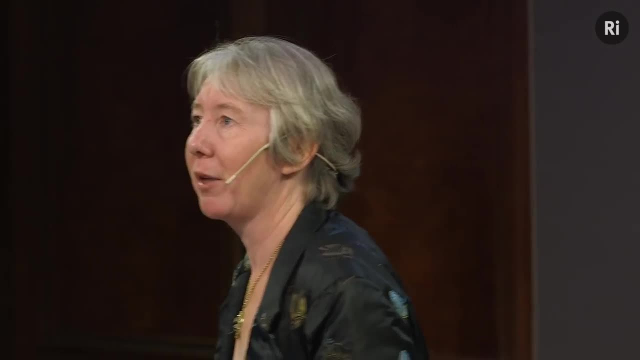 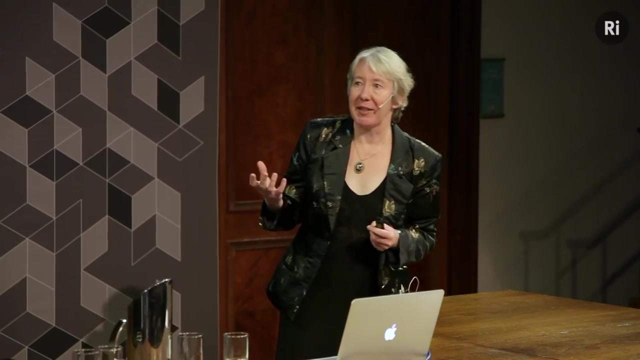 or even 100 times more data. once we get to the high luminosity LHC program We might actually find a new particle. Then we've got to work out: what have we found If we start to see extra events with missing energy? 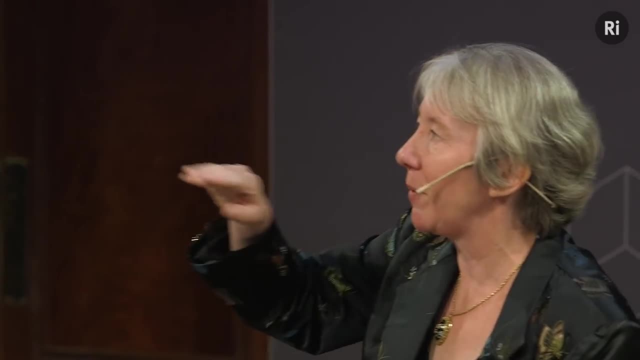 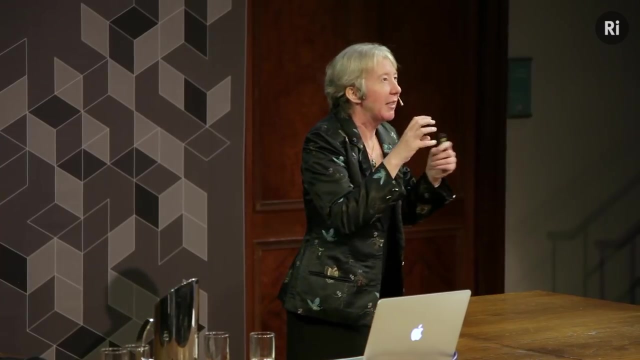 we don't know. Is that supersymmetry? Is it extra dimensions? We've got to measure, really, the details of these shapes, in these curves and the relative rates of different processes. So, just as I was trying to explain for the Higgs boson,